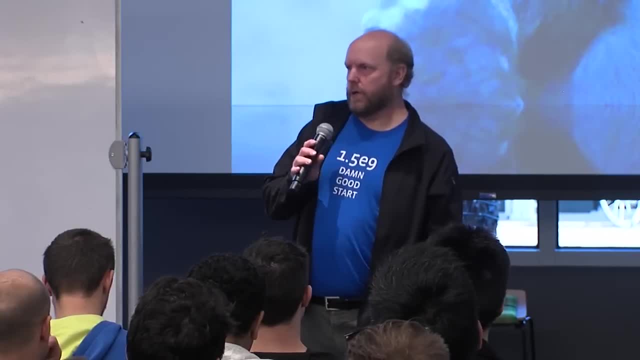 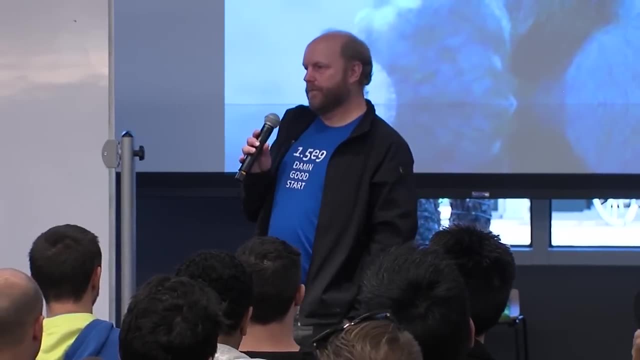 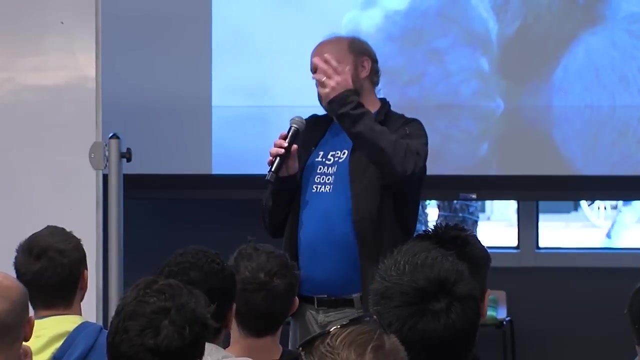 I always like introductions that are short- number one- and this will be fairly short- but I also like introductions that are that are personal, and the lesson that I learned from John is: I saw a post that you made at one point where you described you'd spent two months working on. 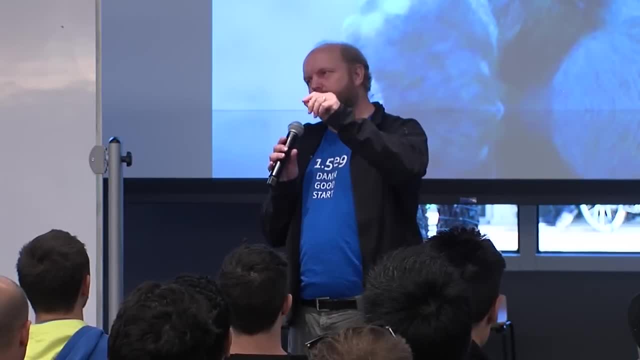 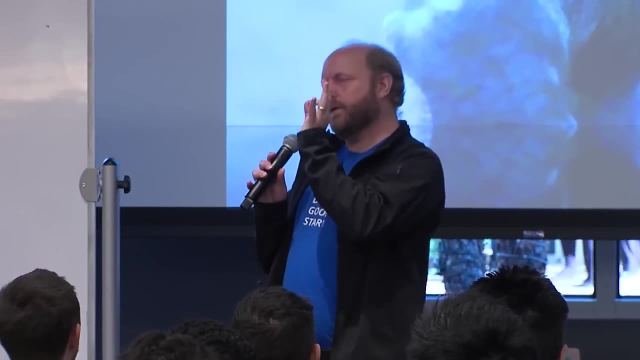 the perfect. now I'm going to forget the details, but the perfect implementation of I don't know sparks flying off a tracer bullet or something like that and there was a. There's a really good way to implement it. that was perfectly clean and you just couldn't. 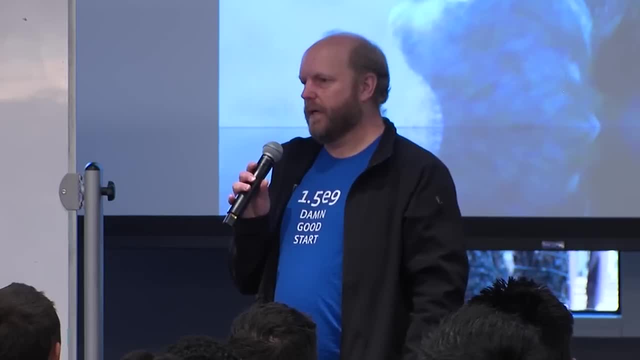 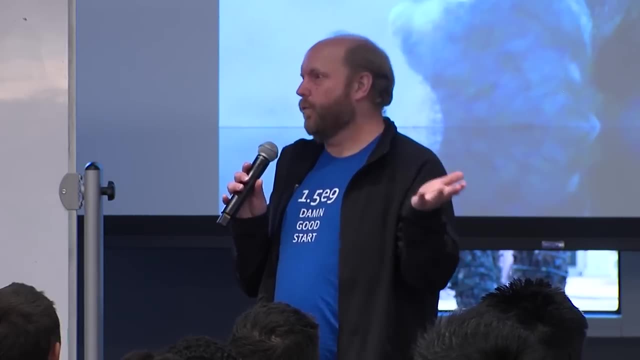 get a performant implementation of it. And so you just said: well, but there's this stupid trick, So let me just do this stupid trick. and it worked just fine, It looked just fine, Do you remember? Is this ringing any bells? 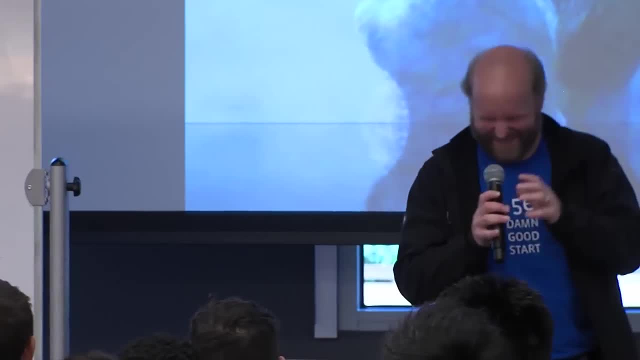 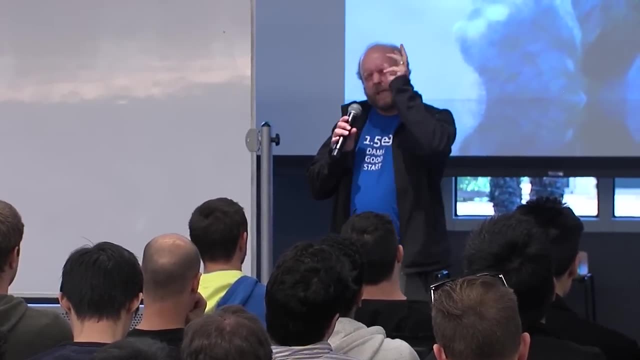 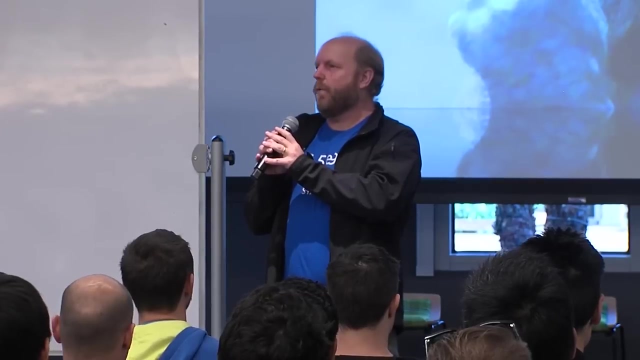 No, there's been hundreds and hundreds of things like that. So the lesson of that for me is that, even if you're really really smart, sometimes the best way to be really, really smart is to figure out why you don't have to be really. 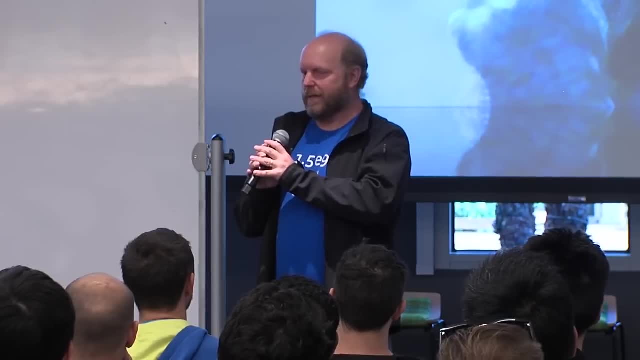 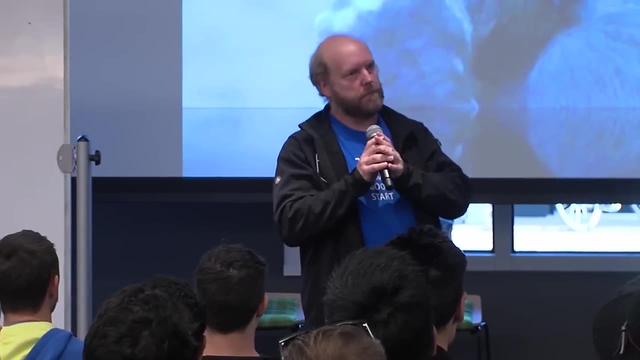 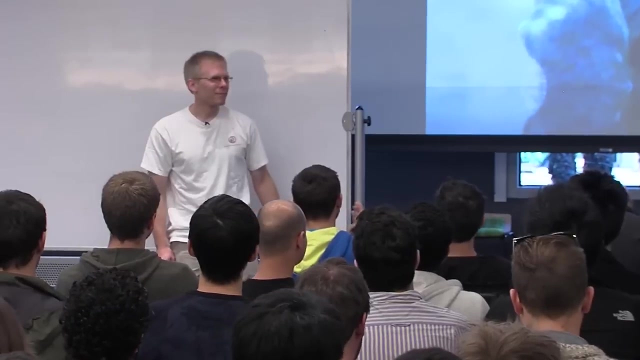 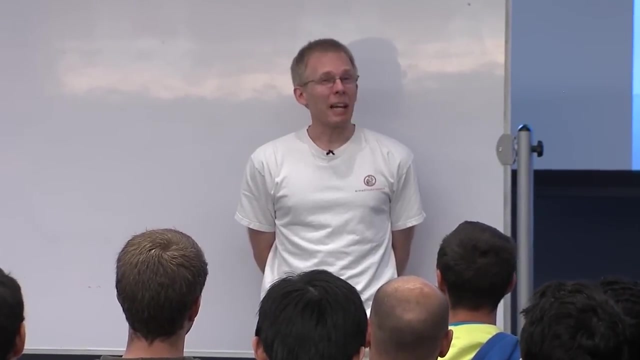 really smart. So I want to thank you for that lesson and I've tried to keep that in mind for the rest of my career. And now, without any further ado, I would like to introduce you to John Carmack. OK, so after I got the invitation- and I do kind of beat myself up for not being more- 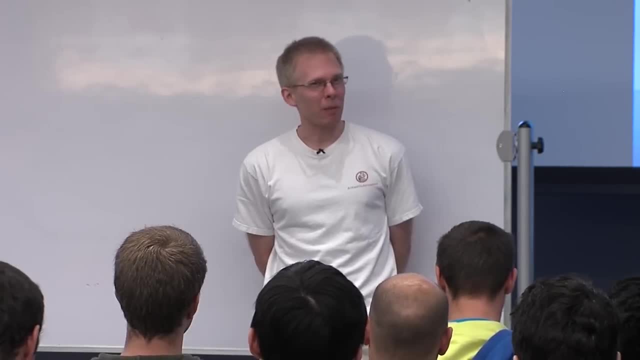 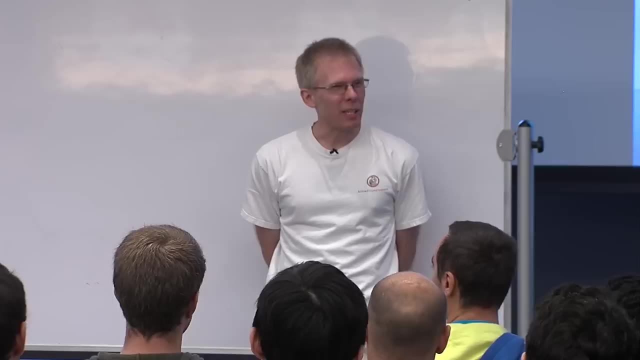 engaged with the broader Facebook engineering community. here I do kind of like my little vermitage down in Dallas, but there's more that I should be doing to try to kind of be a part of the community here. So I thought about it and I wrote down at least a dozen things that I could go and talk. 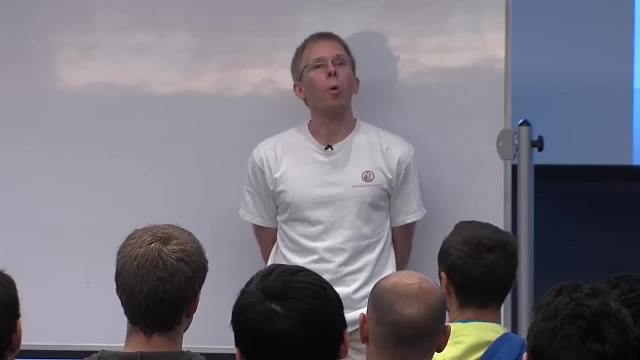 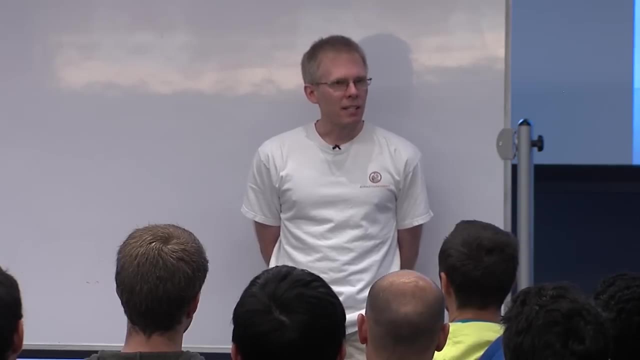 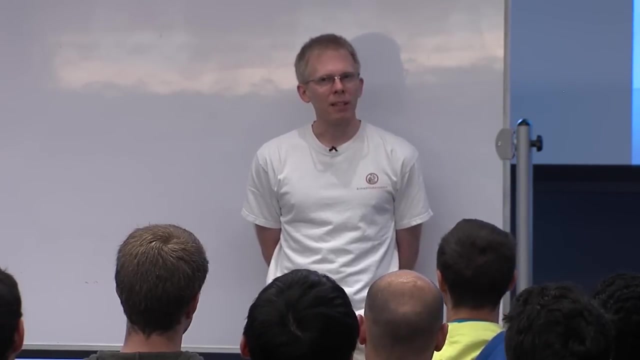 for hours about. that would be interesting topics, Hopefully educational to some degree. But what I settled on somewhat topically was this notion of ideas and engineering And this was kind of triggered by before Oculus Connect. a month before last, Michael Abrash had sent me an email asking if it was OK to tell one of the stories of the original. 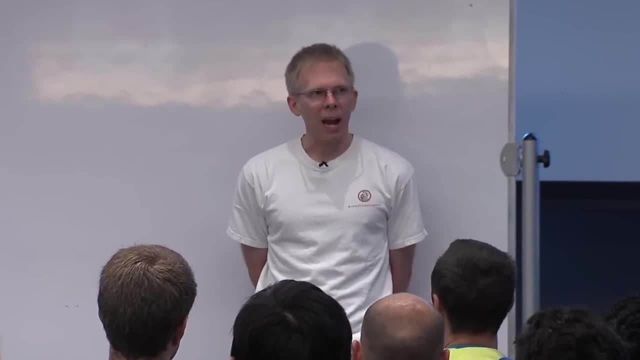 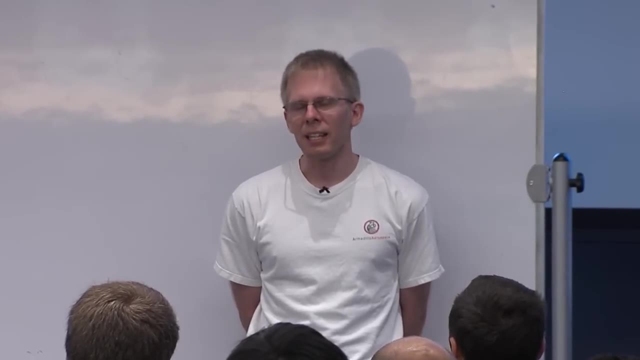 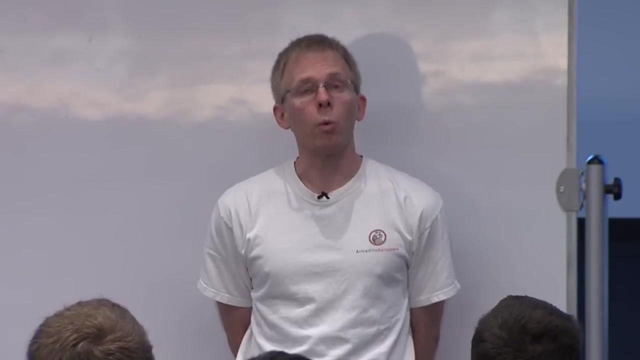 quake development about how I had gone through all of these different paths for basically visibility culling to get the speed up to a certain way before settling on this one potentially visible set idea- And he did a nice presentation at Connect with this, The basic idea being that research- what he's the head of here at Oculus- is not about these. 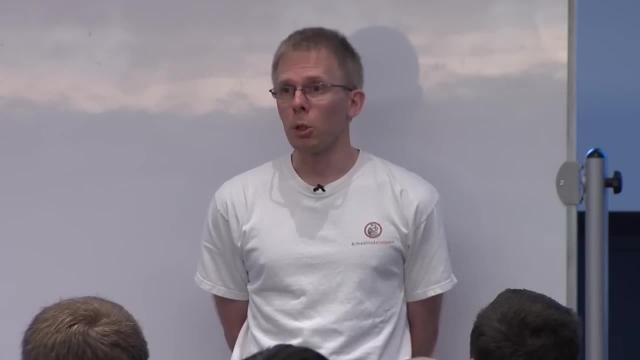 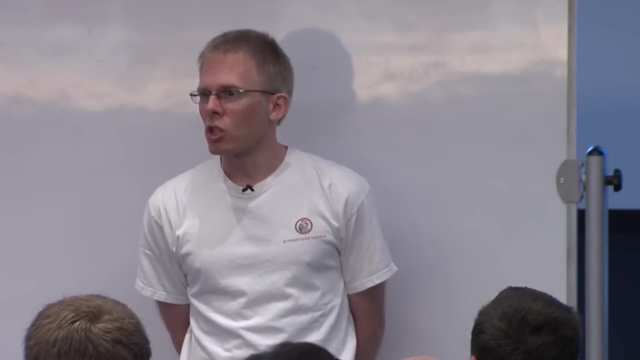 light bulb, brilliant ideas that just strike you out of the blue. but it's a whole lot of work that leads to the ideas, And I quibbled a little bit and said that there definitely are light bulb ideas where you can be sitting there working and something does come to you in a flash that may or may. 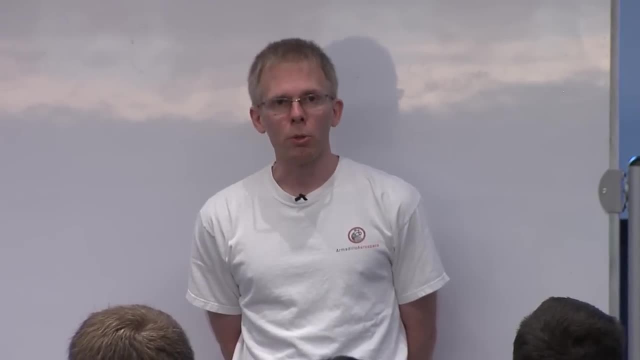 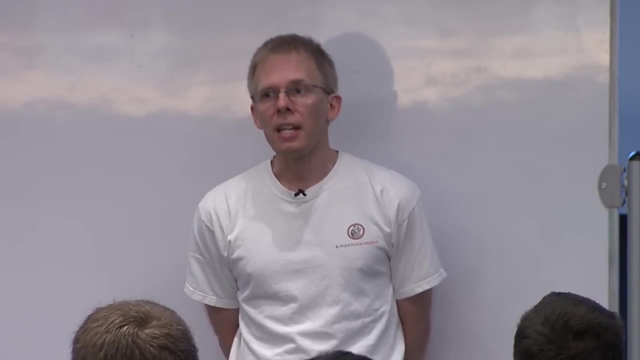 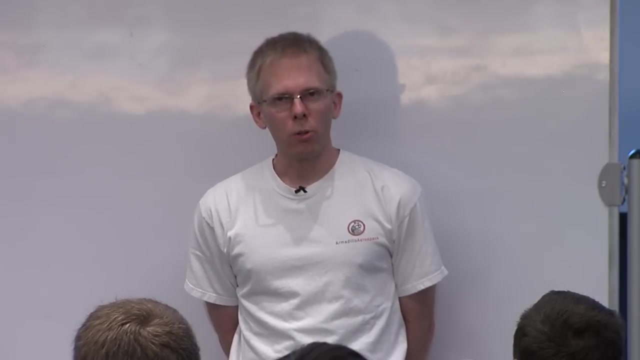 not be a great idea, But the core of the lesson is absolutely true. You get the ideas by being down in the mud, working on the problems. that it's the hard work that leads you to the insights that are, hopefully the great ideas. And we have in our culture, the broader culture here, this sense that everybody loves the. 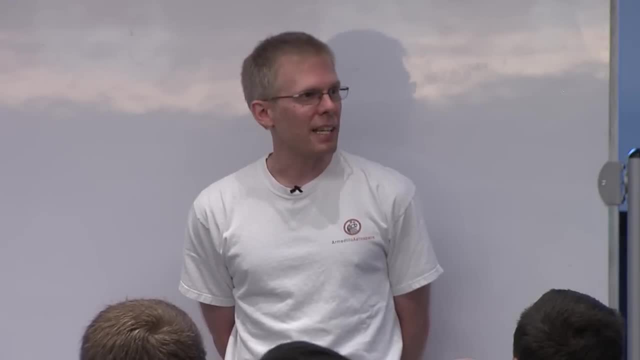 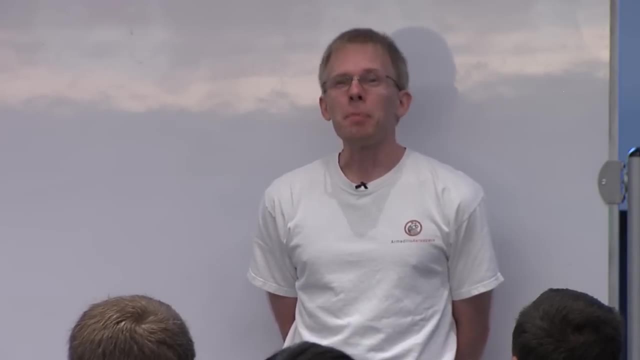 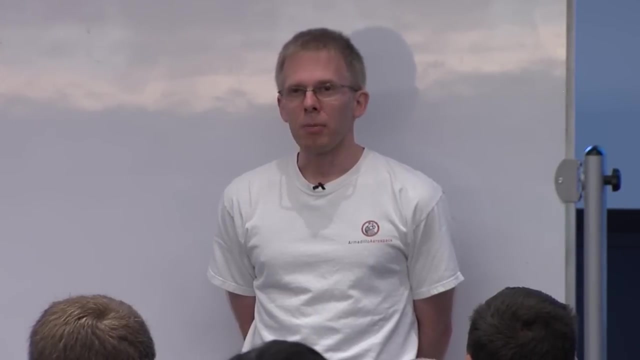 idea of the lone inventor that has the brilliant idea that then they patent it and they get rich afterwards, or it's stolen by some faceless evil company and they're exploited. These memes run through our culture in different ways And over the years. as someone with a little bit of notoriety as a game developer or a rocket, 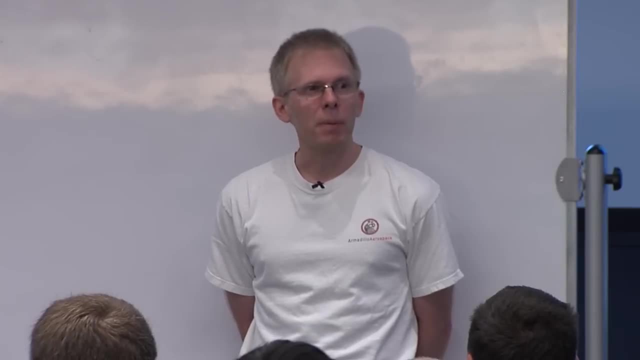 scientist or whatever. I get emails from a lot of people that are often earnest people that believe that they've gotten a magical idea, And usually it's approached by saying: I've got a great idea, I need you to sign an NDA. 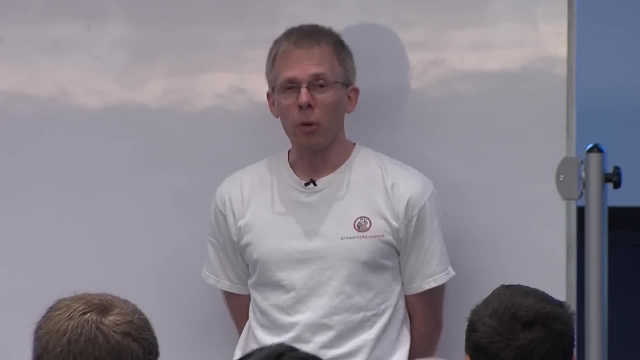 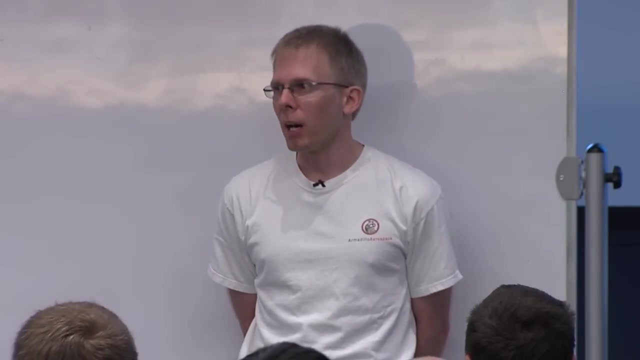 so I can tell you my great idea and then maybe you can work on it with me. They're usually people that think, okay, this idea is magical, I can't build it, but we need to find somebody that can implement this idea, and then we'll. 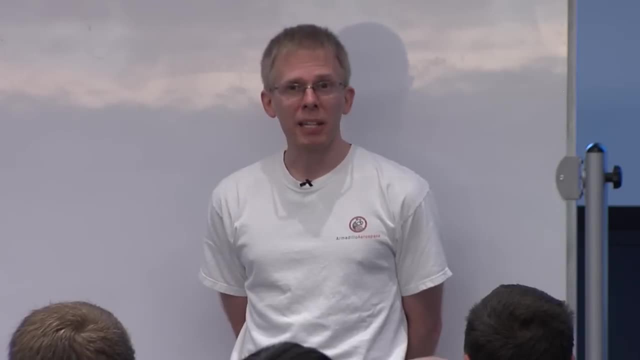 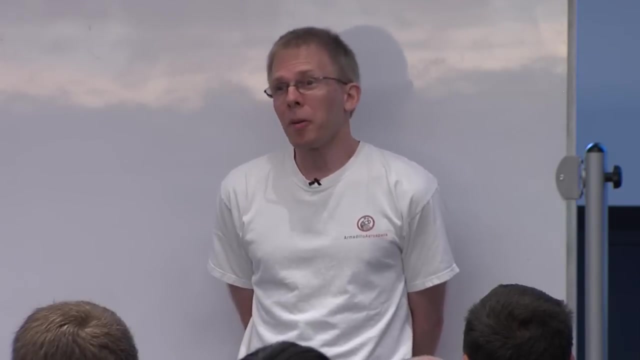 all be hugely successful. Now, sometimes I can talk these people down from their patent application and their NDA requests and I can look over the stuff. I mean, I give advice for free. I am happy to look, I'm happy to hear your ideas and tell you what I think about them. 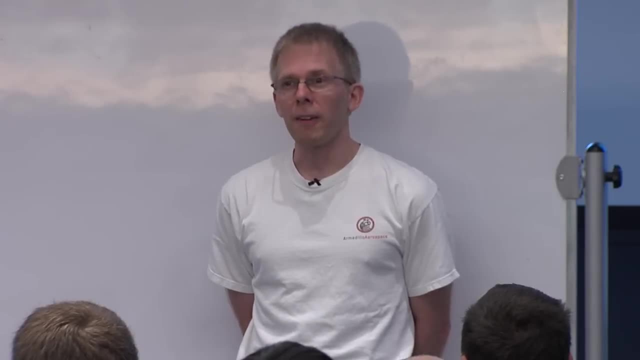 And invariably in these cases we'll go through the stuff and it's either something that's obvious to someone, that's a part of the idea, It's a part of the industry that they're talking about, or it's something that has. 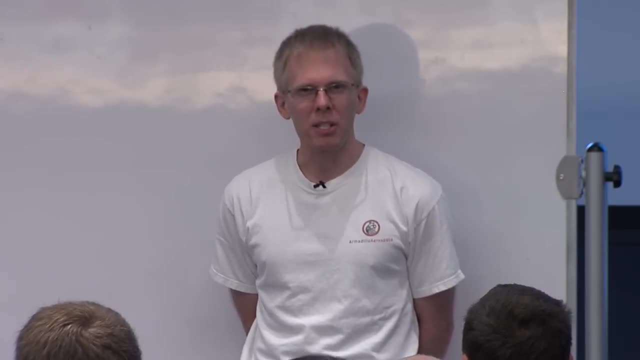 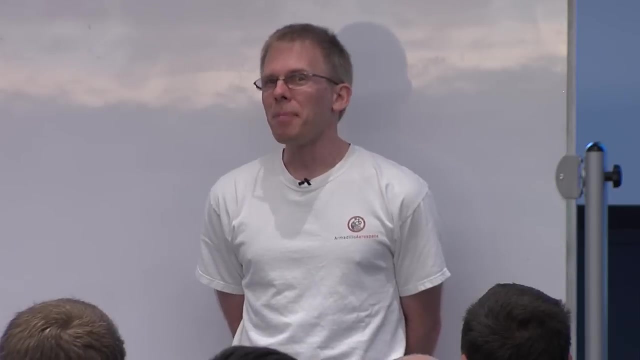 a fatal flaw, or it's just kind of incoherent or it doesn't really address things in different ways. But I still try to encourage most of these people that, if you're thinking about ideas, this may be the first time they felt that they had a really great idea. 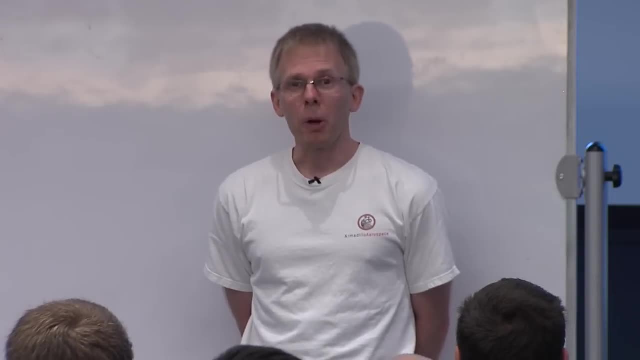 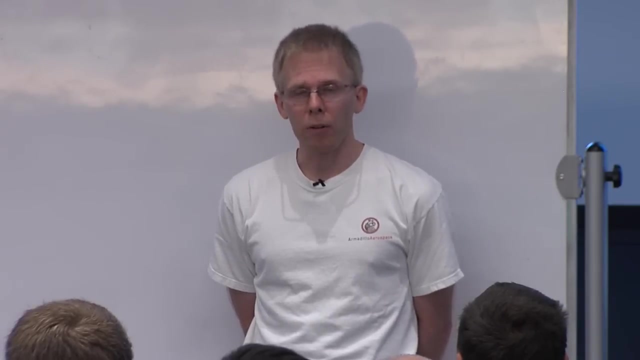 And often they're young- not always, but I try to let them know that it's great to have ideas, but you need to have lots of them, because lots of your ideas won't work out very well, And the way to go about it, of course, is to try to build the things, try to build the. 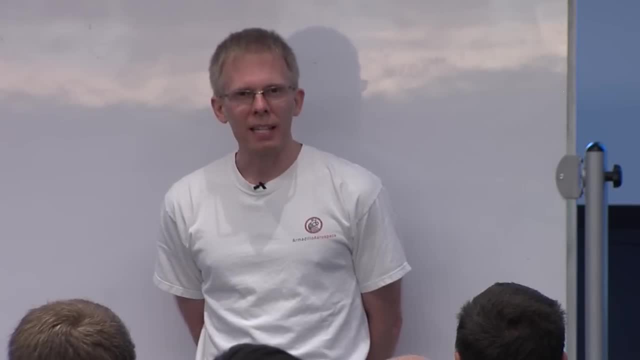 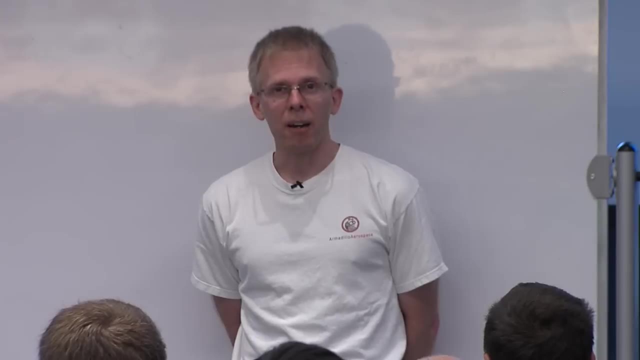 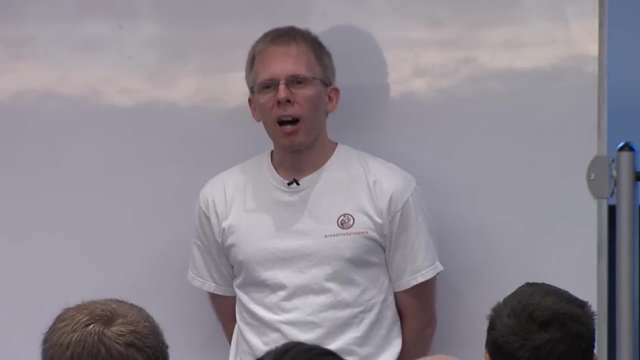 prototypes, And often it means really knocking your ideas down- that it turns out that your great idea is probably not that great. You may need to have a dozen more ideas before you land on something that really is great. There's a quote by Robert Heinlein, the science fiction author, and he said that an idea is 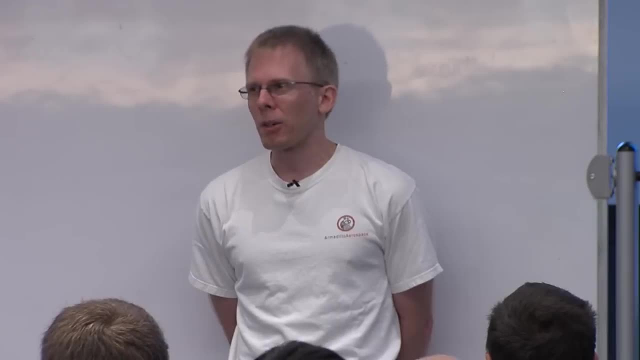 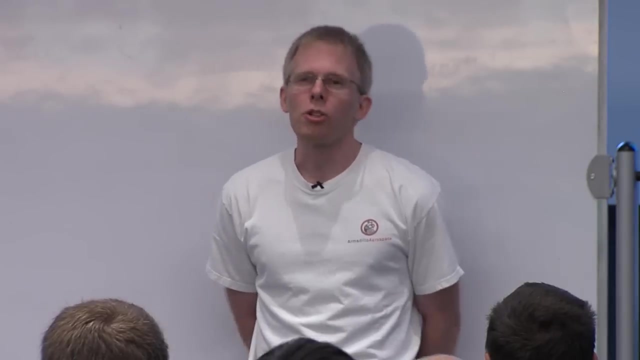 worth exactly one bottle of scotch Where, for a writer, You know someone who's Who's even more than software. in many cases, where ideas are the stuff that they build, it's still a matter of execution is much more important than that sort of original core. 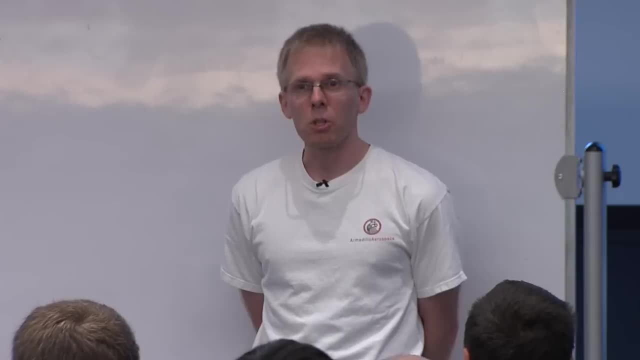 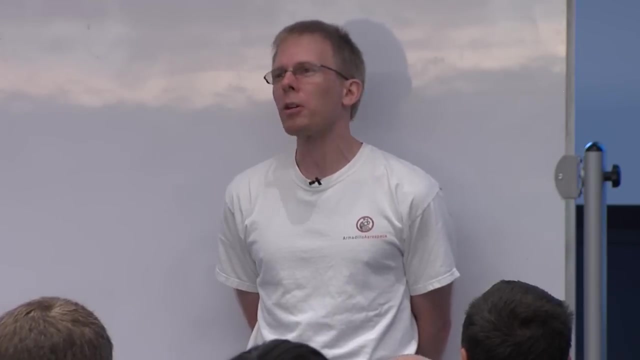 idea. And there was another Heinlein story about how one of his friends that was a struggling writer was really down and he just, Heinlein, sent over a whole page full of ideas like wonderful ideas that could each be turned into some great science fiction story with. 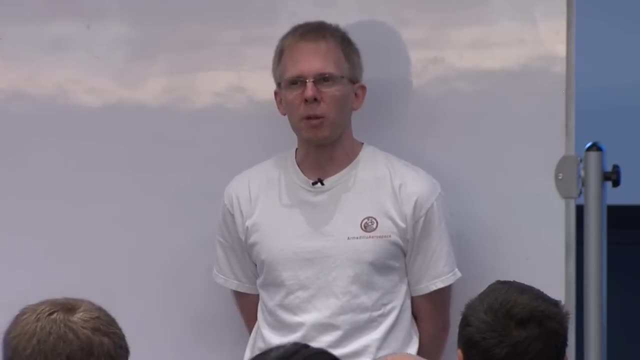 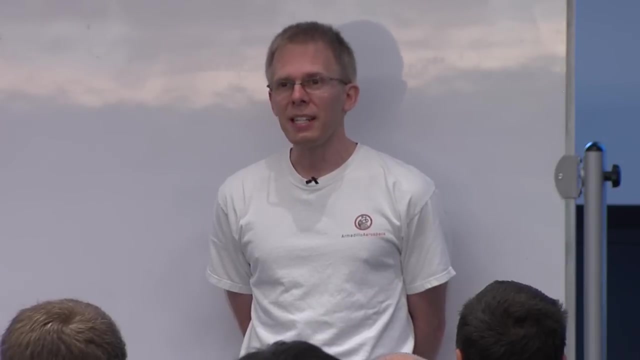 just a you know, we hope that this gets you unstuck, that you can follow something off from this, And I've taken that tack through most of my career, trying to say that you know, the ideas really aren't the important thing. 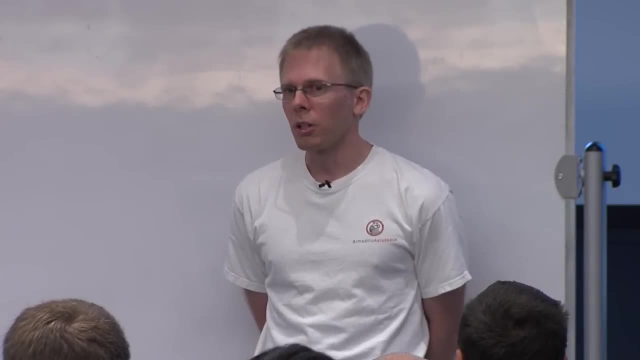 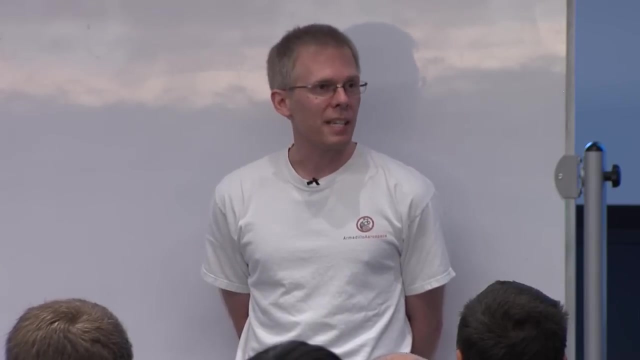 It's the execution, where a good project is a result of hundreds and hundreds or even thousands of good decisions that are made along the way that you know you could start with a great idea and if the implementation's not good it's, you know it's gonna fail. 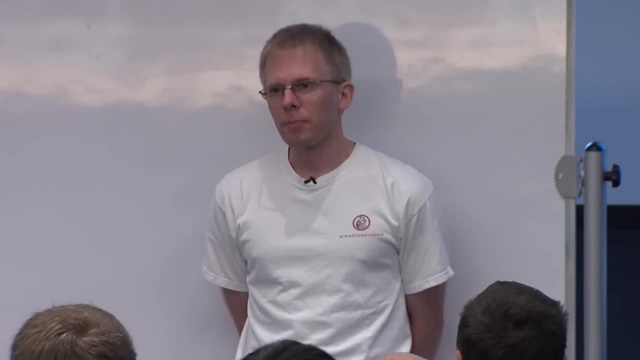 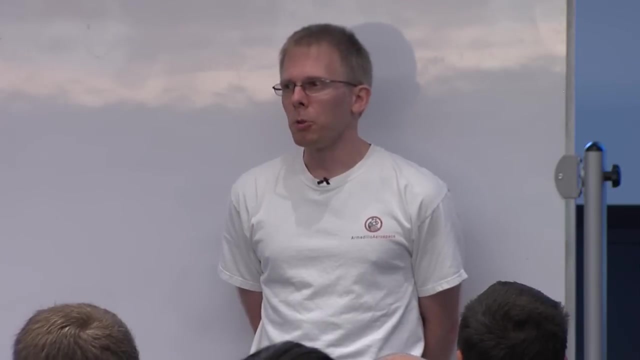 That good implementation is where you need to focus your efforts on, because the ideas they do, They come and they go And it hasn't mattered that much. Now I carry this into a lot of the way I think about things. This influences in many ways my views on software patents and some of these other areas. 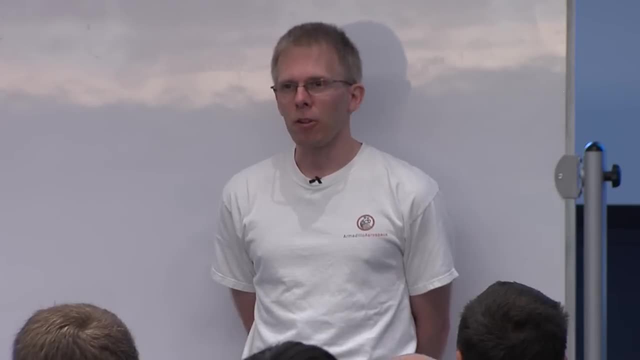 where you know. I don't think that trying to nail down this high value on a specific idea when the idea is this tiny fraction of the product is a particularly good thing, But still there's this sense that clearly ideas mean something. There's plenty of cases where you have conflict. 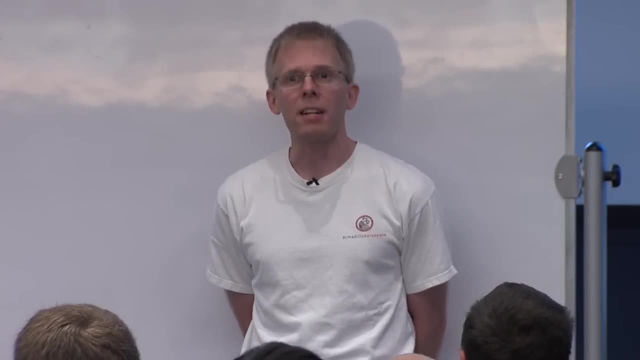 There's plenty of cases where you have competently executed projects that fail to leave any dent on the world, even though they were done with all the right decisions, But there was something missing there of maybe there was grand ideas that were necessary to make the big impacts. 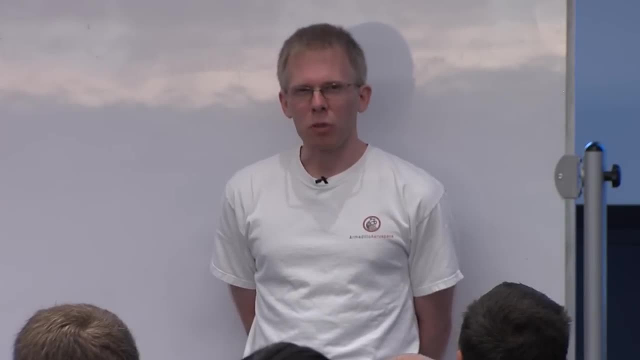 So I've actually been toying with this idea, about ideas recently, And this is, you know, what you'd call sort of a cocktail party theory, something that you wouldn't necessarily defend to the death, but it's worth thinking about a little bit. 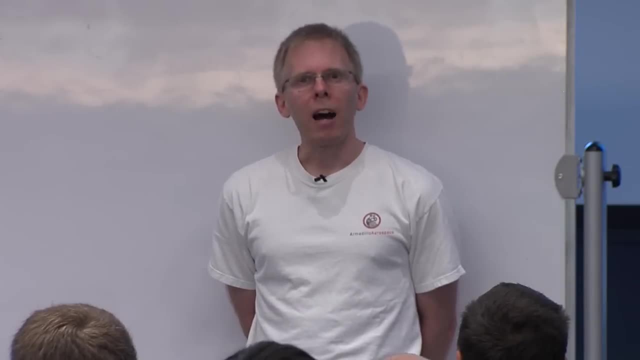 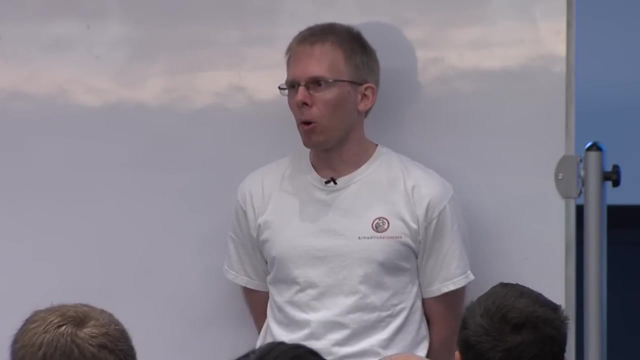 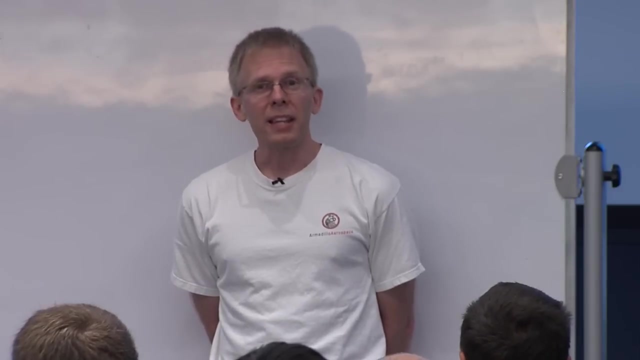 And that's that ascribing low value to ideas may be helpful in getting more ideas, where I see a lot of these people that feel that they've gotten this idea and it's so valuable and they latch on to it and they, you know, they think that this is something that's going. 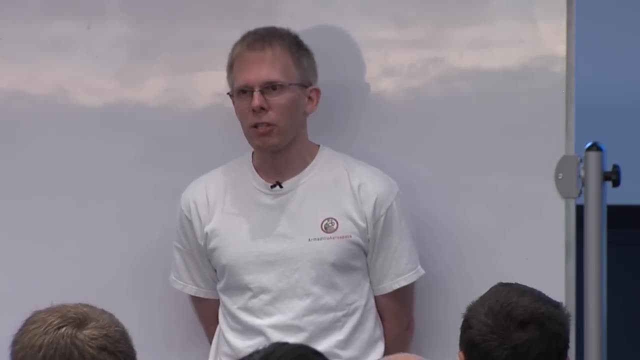 to be great. They won't necessarily look at it as critically as they might want to, as they probably should, or they will be jealously guarding of it or different behaviors that I see, You know, I see in other people and in fact I've seen in my earlier days. I can remember 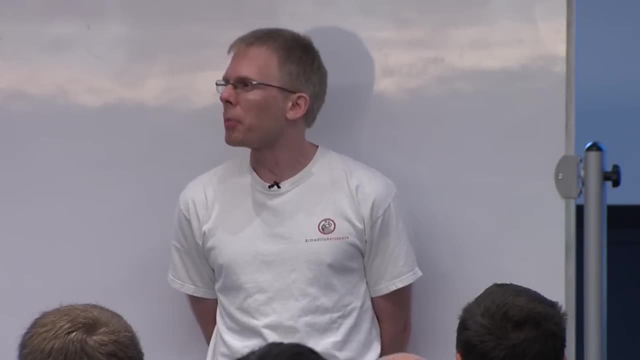 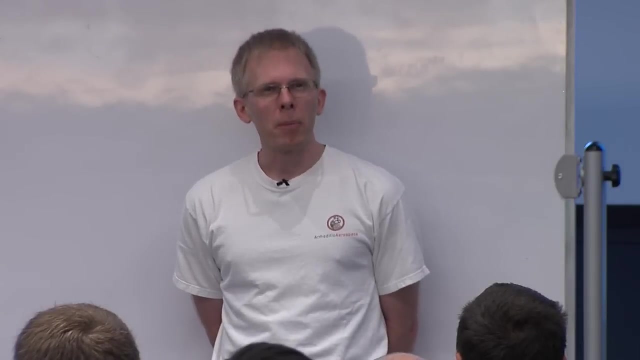 having early ideas when I was at the age of many of these people that email me and say you know it's like: oh, this would be, this is going to be a great idea. Like I can remember on the PCAT, thinking I could hijack the DMA controller to blitz. 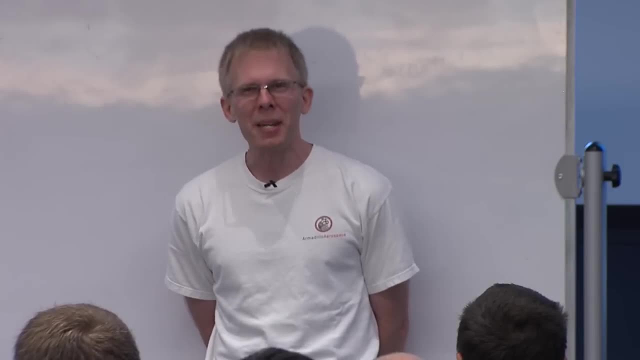 screens and I'm like, oh, this will be great, This will be an enormous speed up, It'll be asynchronous and it'll be great. And I never could get it to work and I was bummed out for days afterwards. 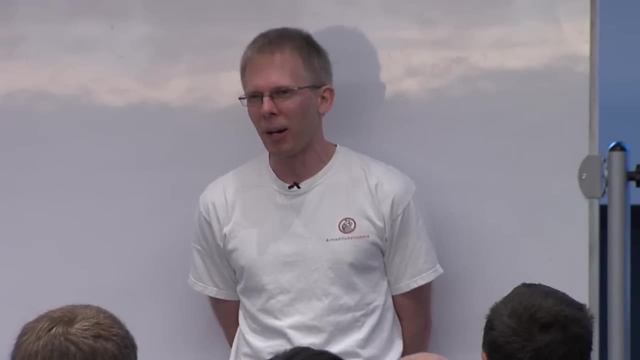 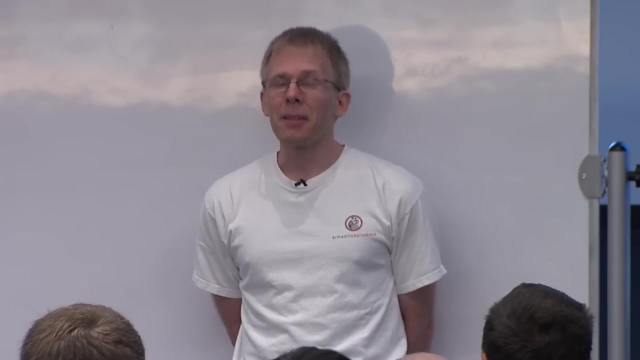 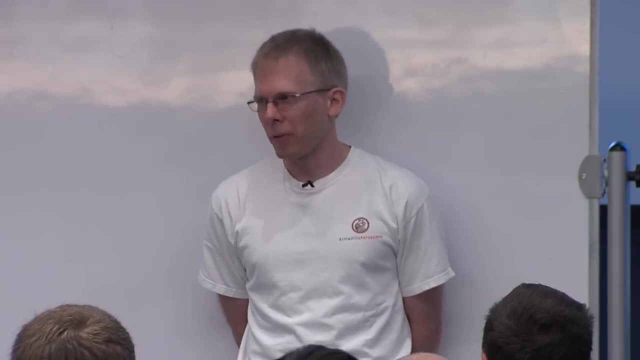 I was like, oh, This brilliant idea that I was all kind of hyped up on just wasn't going to work out, And so I try to when I've got like the timely thing about this was I had already decided on this topic, you know, a few weeks ago, and last week I got yet another one of 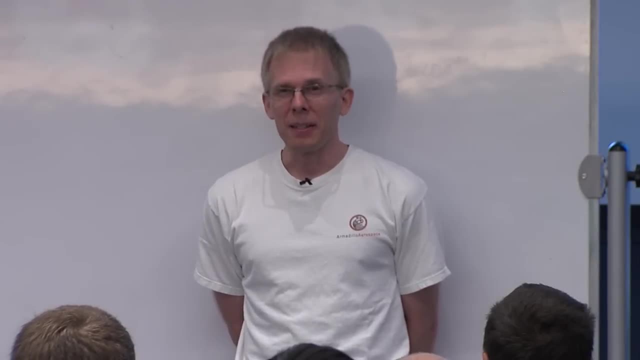 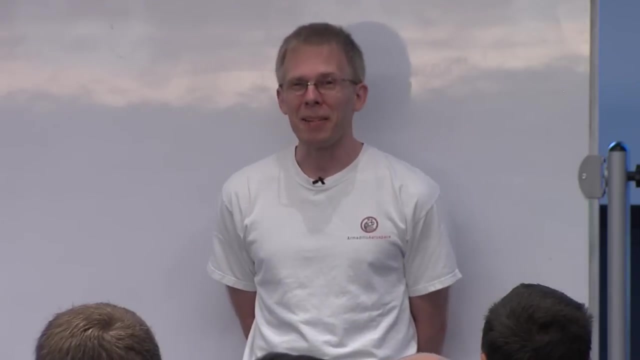 those emails coming in from you know a young guy that said: I've invented the holodeck. You know I have. you know I've come up with this invention and I filed a patent for it and he sent it to me and Michael A, Brash and Palmer. 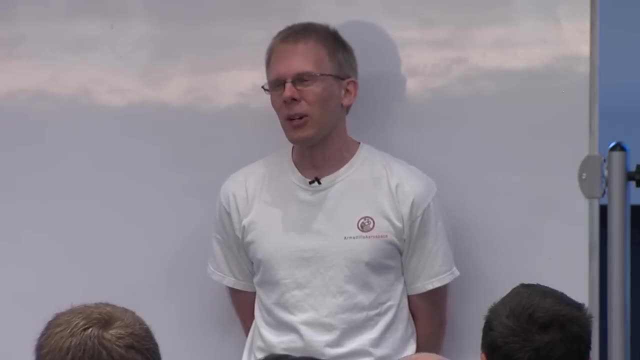 You know Palmer's probably getting a lot of these things now also, And you know I had to tell him it's like. well, first of all, I'm sorry but I can't read your patent application. but you know I try to be encouraging still. 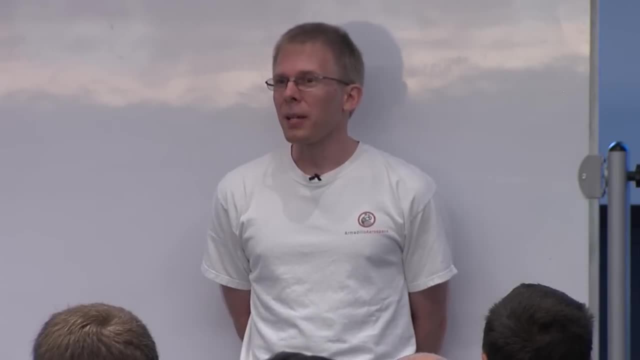 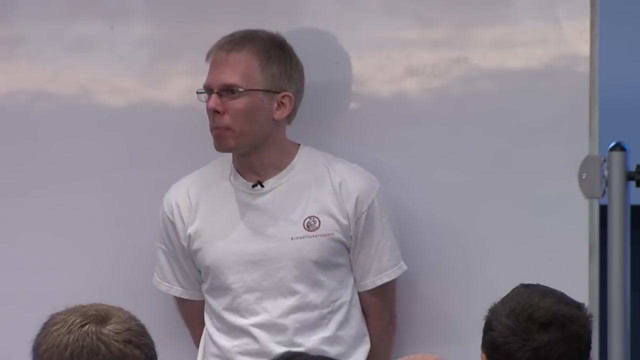 I try to say it's like: all right, well, if you need to start prototyping things like. I should have mentioned that the reason Oculus is here today is because Palmer not had a bright idea, but built a whole bunch of prototypes that eventually were physical artifacts that could make their way to my hands and 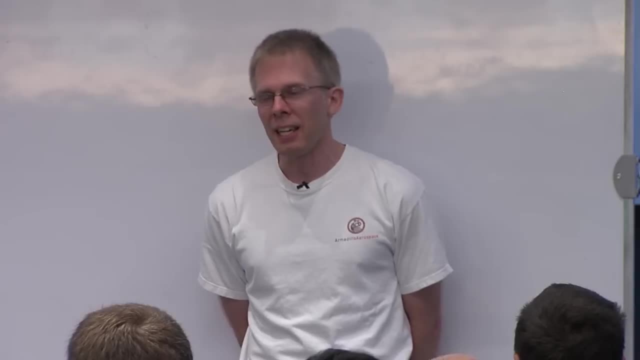 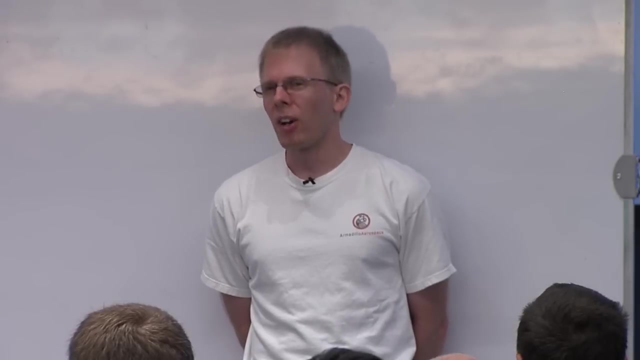 could wind up building a whole bunch of things, Building the things that kind of got us where we are here today. So this sense that the idea wasn't the important thing, but you know, going, iterating on it, building it over and over. 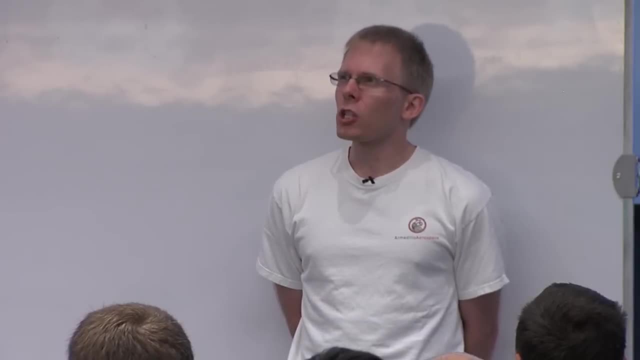 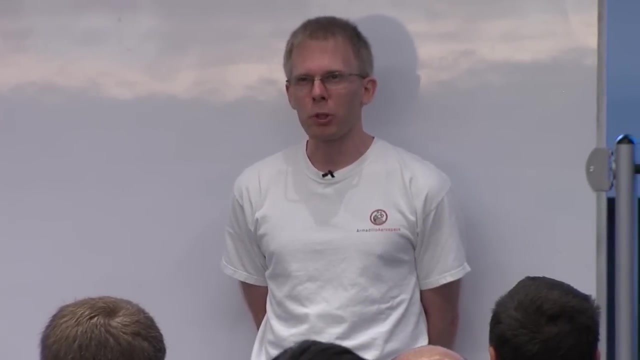 So I've been thinking kind of through that lens, though. is that well, am I ascribing perhaps too little value to some of these things, but doing it as a psychological hack, where I'm tricking myself into not wasting time or spending time in ways that I you know that are not going to be as 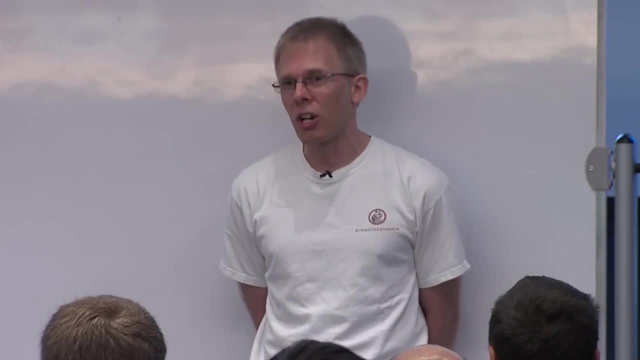 productive, As if I just say: well, ideas come, ideas go, And I like another. after I had mentioned to Mike Labrash about the original my comments on there, I sent a couple more e-mails just like: well, here's the idea that I had this week. 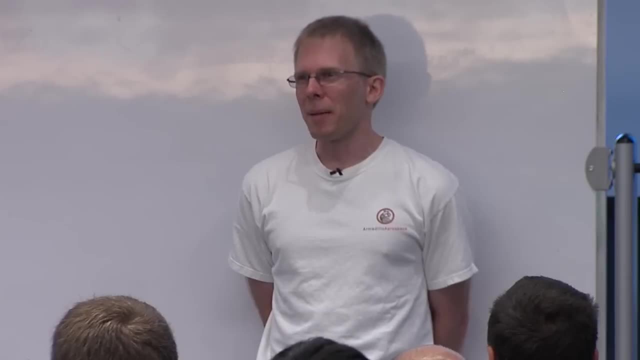 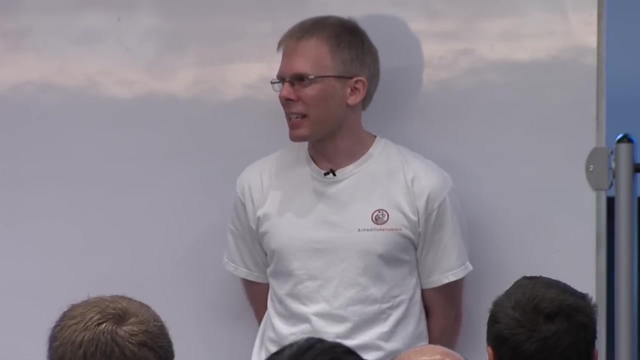 Here's the idea that I had right now, And now I look at them and say, well, this is kind of interesting, This would be awesome if it works out, but it probably won't. I almost look at these things now. it's like I've been through the idea train enough times now, where you 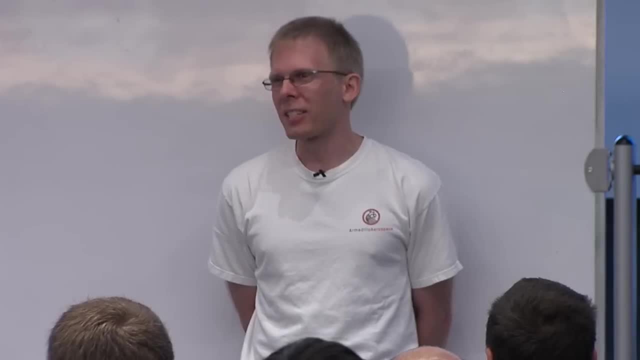 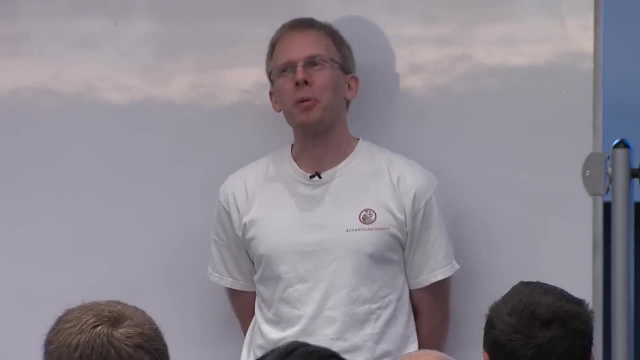 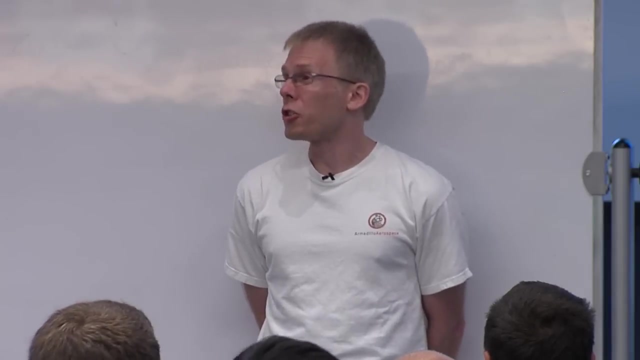 look at something And think, oh, this will be glorious if it works. you know, and I get the idea high at the beginning, but done it enough times now you can say, well, it probably won't. And it can almost be the puzzle game then to find out how to bust my own idea where I, for instance, just a couple 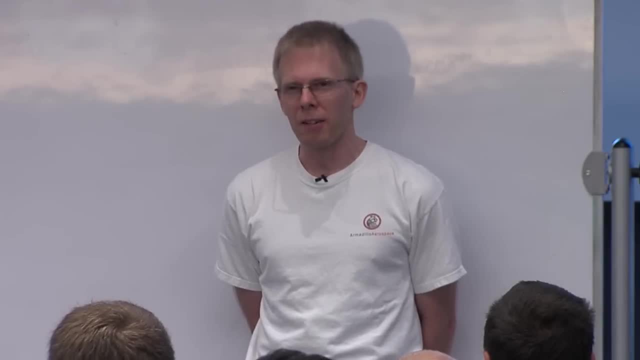 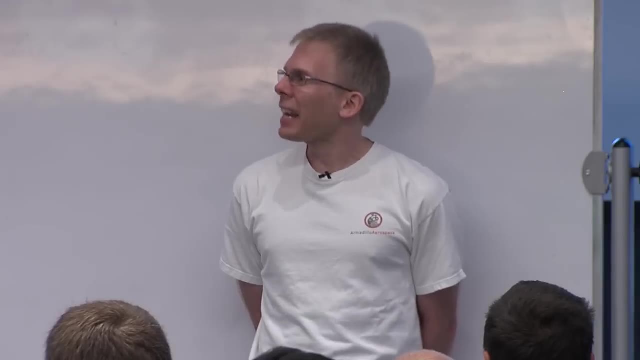 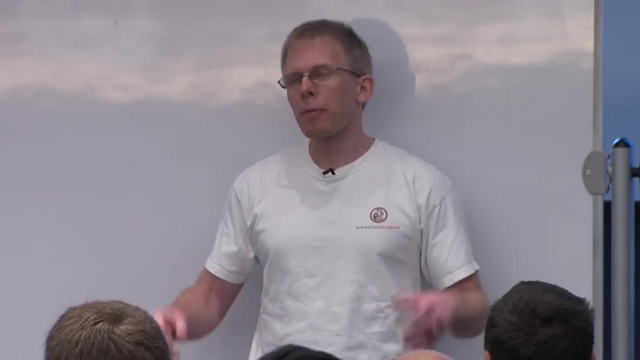 weeks ago I was discussing with the Microsoft Mojang developers about Minecraft- you know, ways to optimize Minecraft for VR and different things- and this kind of tiny little topic came up where. this is a little bit of a very, very small idea. I'm thinking that, okay, if we optimize, sort of everything is broken up into all of these blocks. 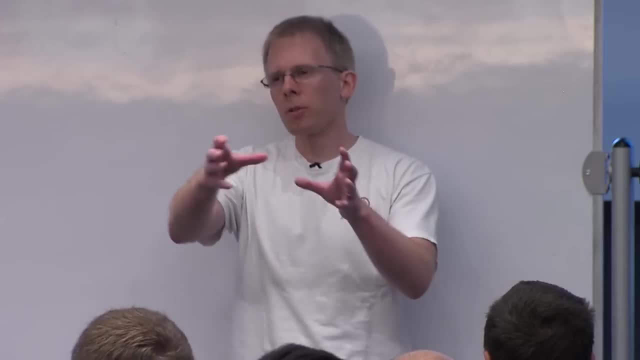 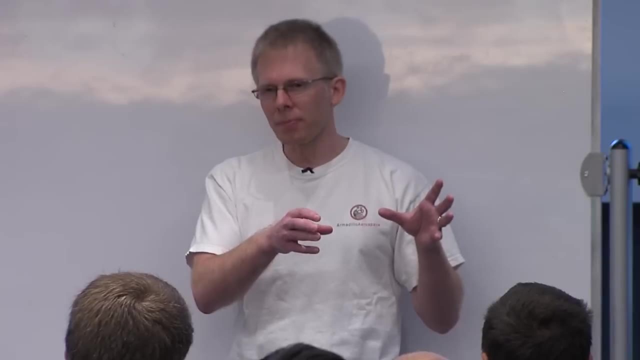 the world is broken up here and they're chunks and they're rendered. you know they're sorted in the order that you render them, but maybe there would be a way that we could optimize the ordering of the indexes that make up all of these. 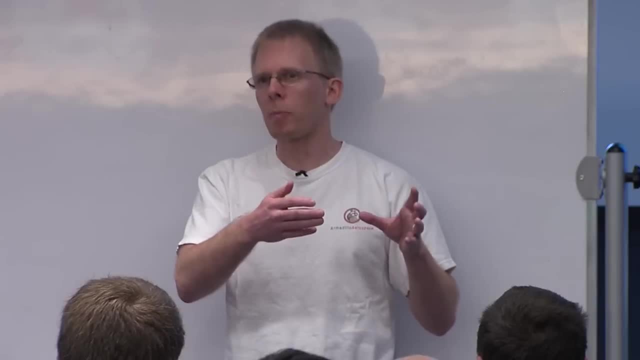 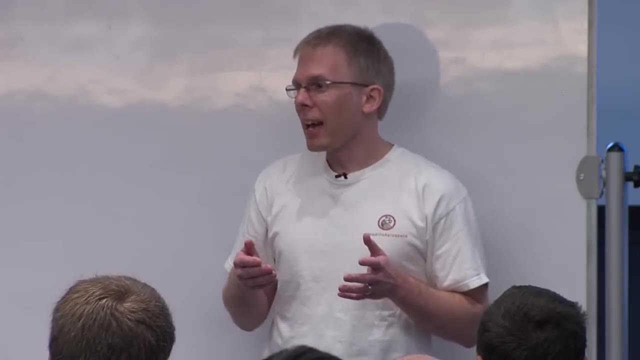 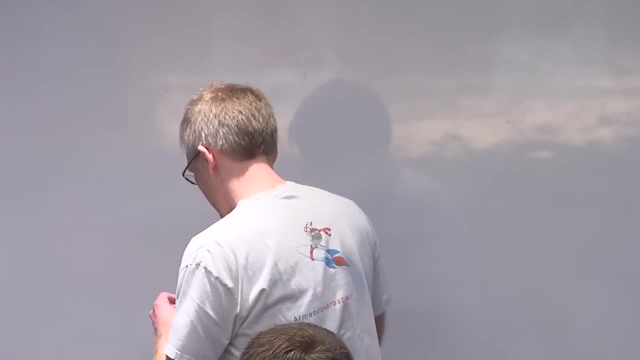 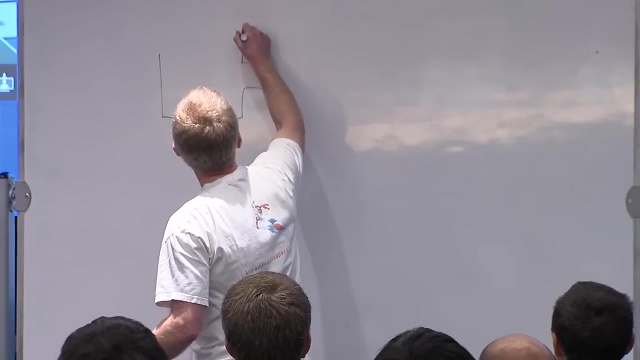 individual blocks so that we could guarantee a certain draw order, irrespective of where you're at. This would be a minor benefit. it would make certain scenes go, you know, a few percent faster. I started thinking about there are some cases like there are some classic cases with occlusion technology and what's. 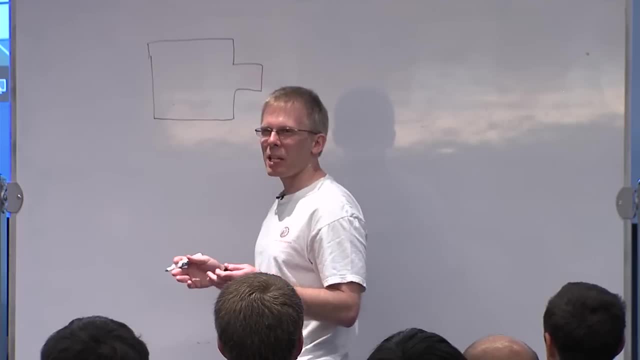 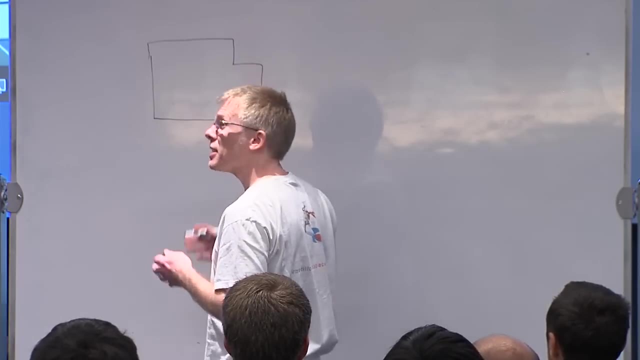 interesting is these thoughts go all the way back to, like, the times of Quake, thinking about draw order, and the fact that they can come up in topics that are happening, you know today, 20-something years later, is interesting. There's something to be said there for ideas that even didn't pan out. 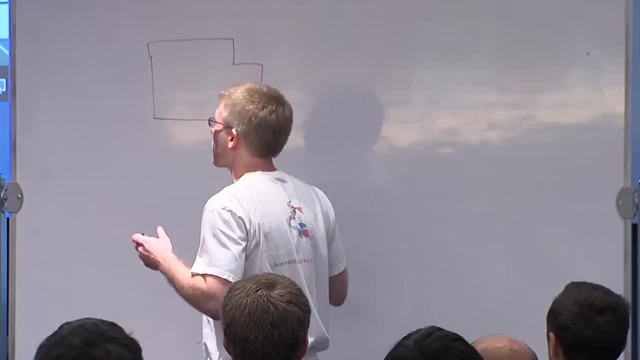 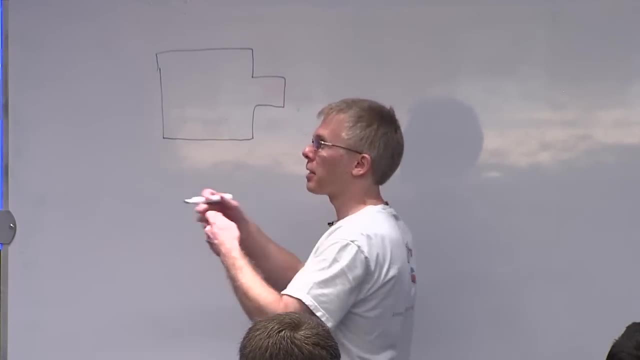 In the old days sometimes come back and can make an impact. later You can even say virtual reality is like that. but one of the classic issues with computer graphics is drawing order. Either you're drawing back to front-end painter's order or nowadays, on modern hardware, you're trying to draw front-to-back. 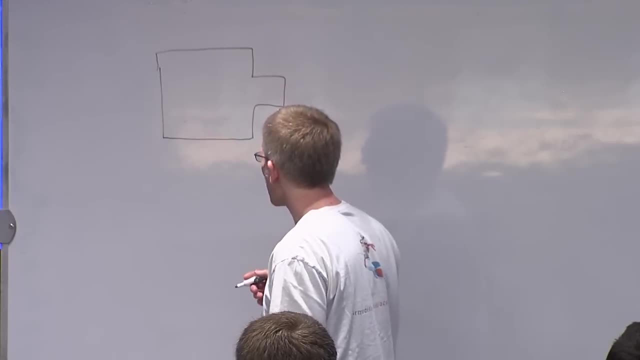 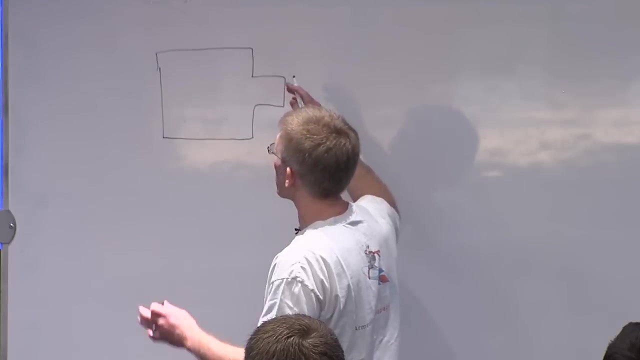 so that you don't wind up drawing things once you've already filled them in. So in some cases for simple geometries, there are orders statically that you can assign to things, where if you had a surface like this and you had back-face culling, you could say that if you wanted to draw front-to-back, you could always draw this one, this one, this one and this one. 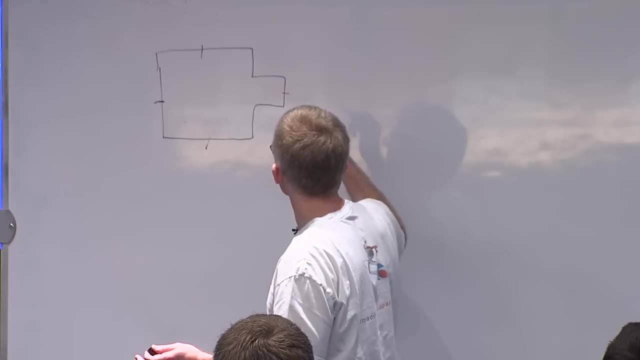 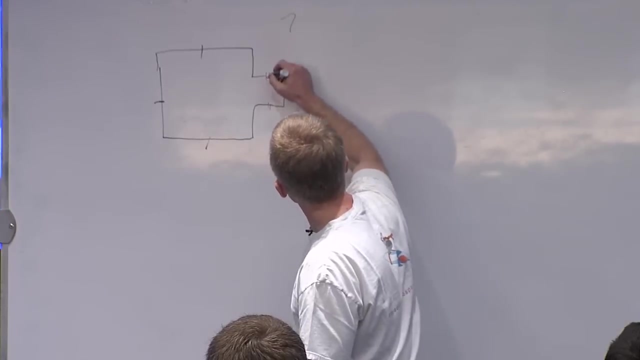 because nothing can ever occlude those. They would be the topmost things. Then you would have to draw these two, because if you were over here looking at it, this one could occlude this one. and then, at the final part, 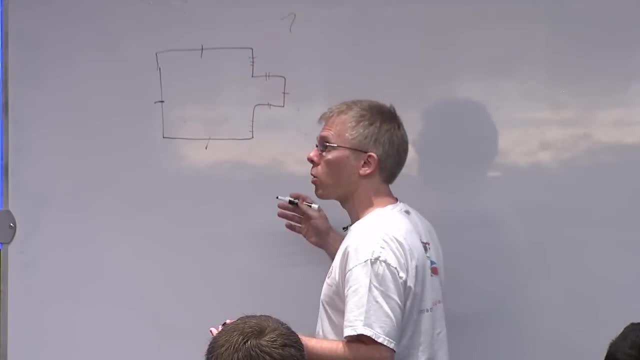 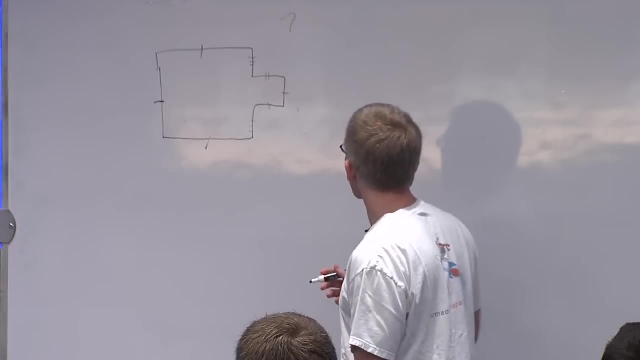 you could draw those in stage three. So for some things there are static orders. This is a you know, this is a small thing that I that I looked at back in the days of Doom and Quake, in the early days of graphics technology. 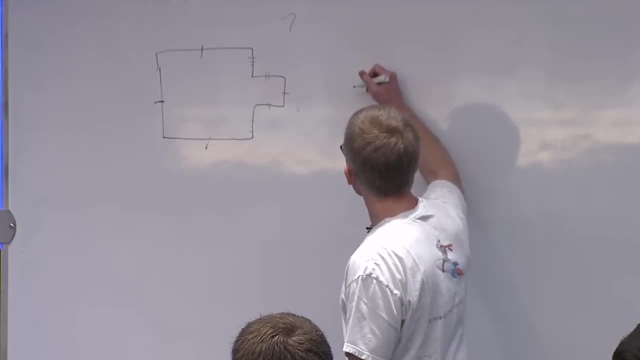 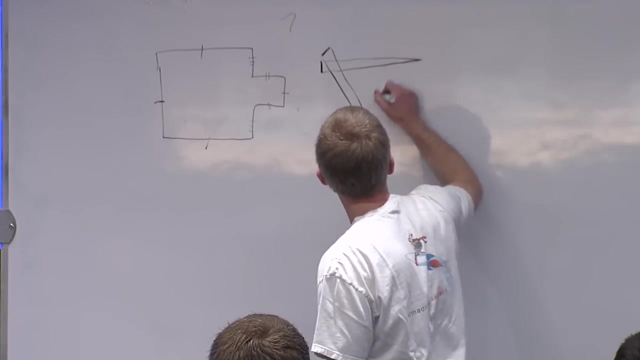 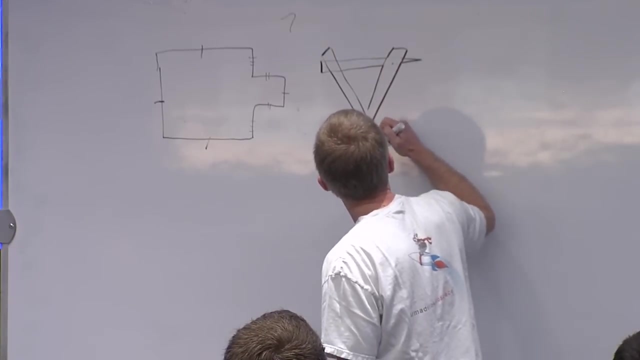 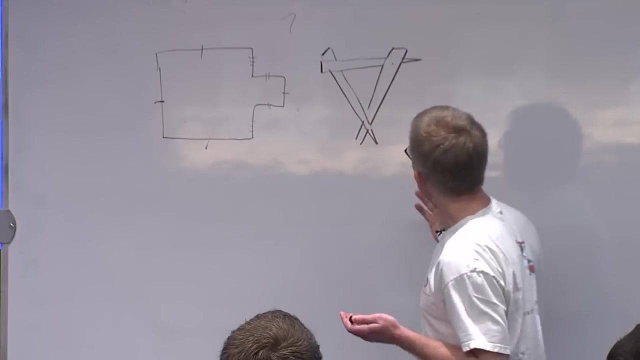 Now there are lots of surfaces, lots of orders of geometry that don't work out like that, Like a. You can make a set of three things that go- you know that overlap- in a way where there's no static order. you can draw the draw the triangles in a way that will guarantee that they get they get drawn in the right order. 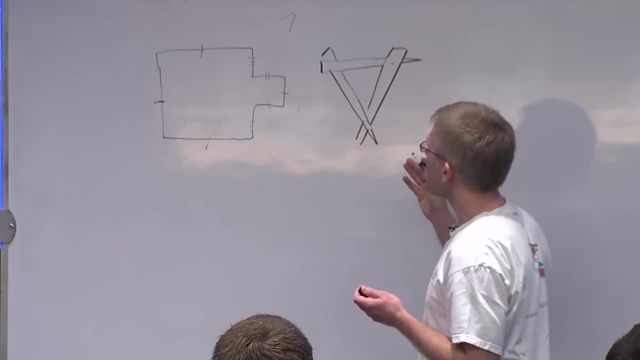 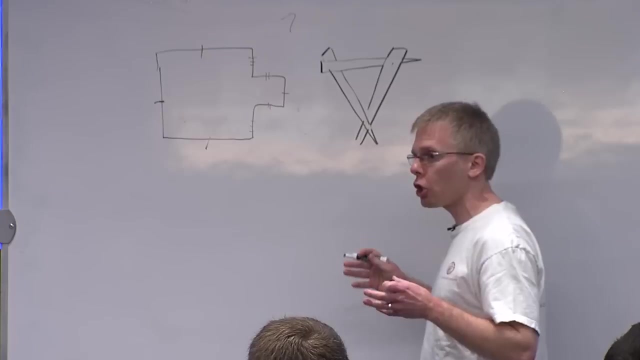 You have to introduce splits. So you know, being aware of both of these cases, I was at least thinking it's like okay, well, Minecraft has this interesting characteristic that everything is diced into blocks. It's all just cubes. 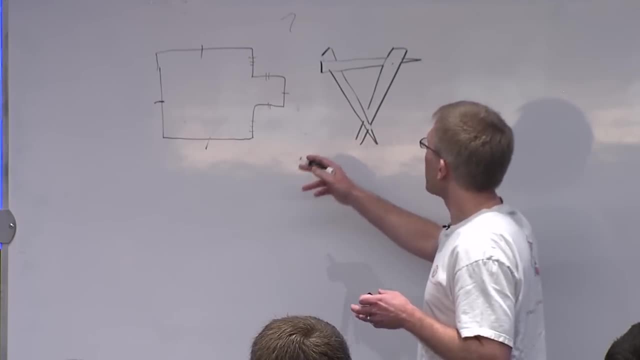 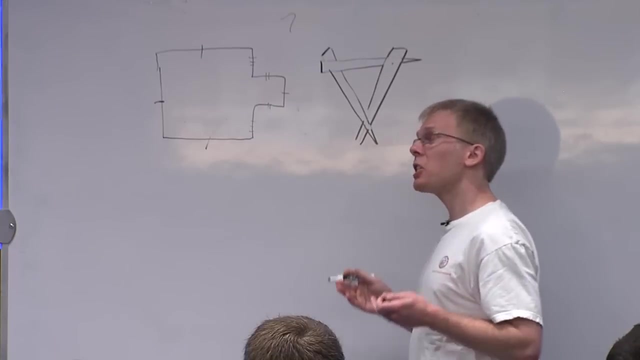 So is it possible to apply a static ordering? since you know that nothing would ever have to be split like this, because they can't cross over that, would it be possible to make a static ordering? This is one of those things that 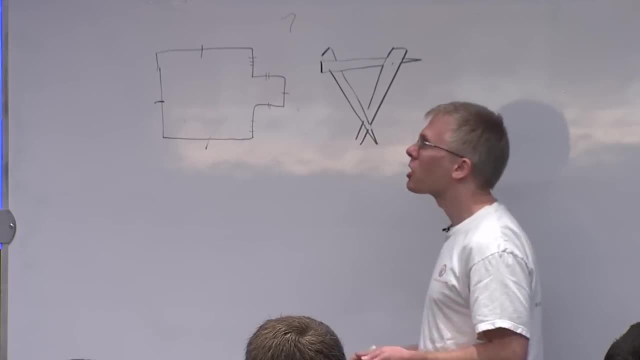 this would be clever. It would be no additional memory. It would give us some speed up in some of the worst cases when you have lots of occlusion And I'm thinking, oh, this is a great idea, Aren't I clever? This will be fun. I can start thinking about the implementation. 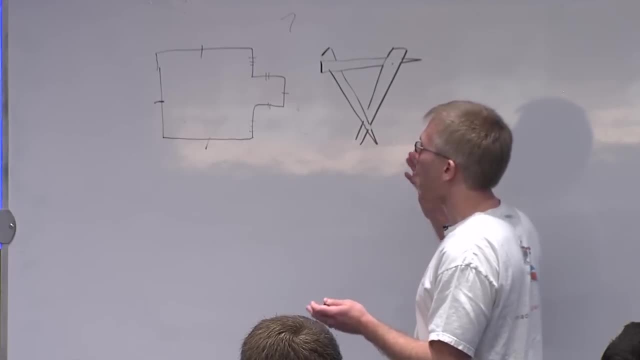 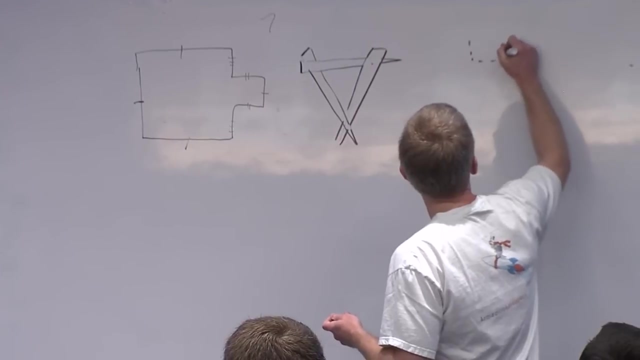 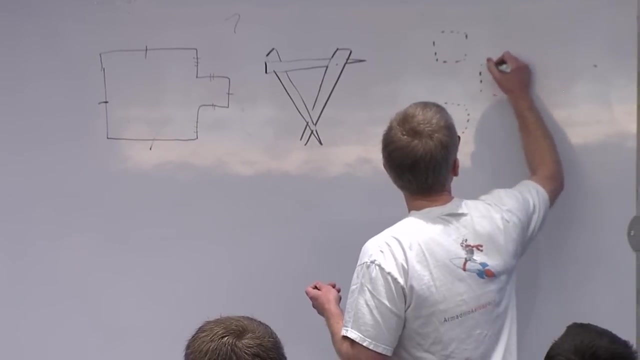 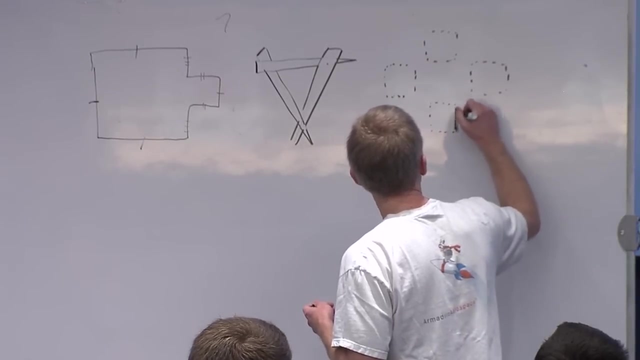 But I I look at it like, okay, I start thinking through how would I build this, going kind of from the outside in, until eventually I started drawing the pictures of the blocks and figuring out what busts the idea. So you have blocks like this with a solid wall here, solid wall there, all that wall there. 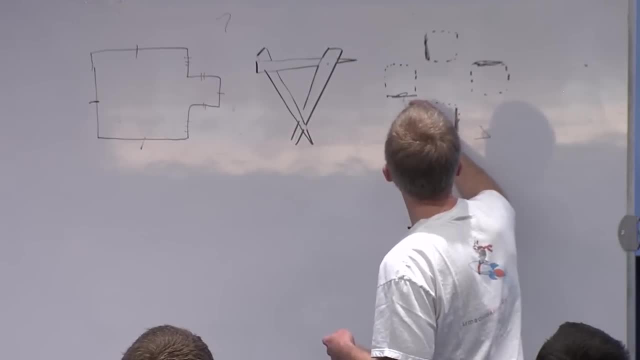 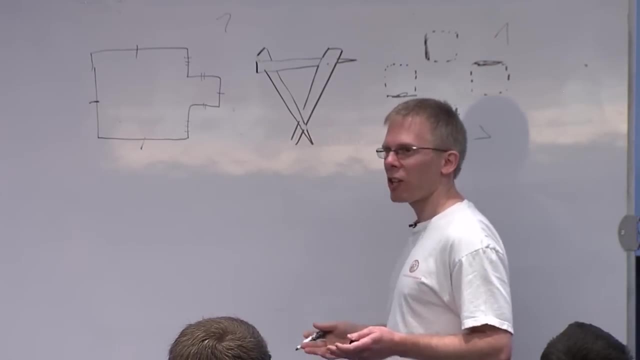 And there you have a sequence where from over here, this one has to occlude this one, from there, that one has to occlude that one, But from here this one has to occlude that one. So the idea is busted. It doesn't actually work out. It seemed like a great idea, but there's a clear failure case. 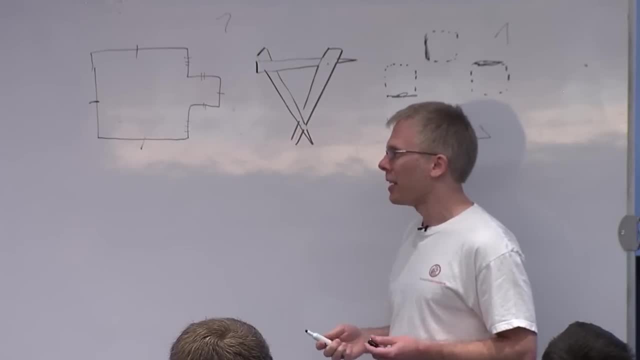 and it doesn't work. So this is just the type of little idea that i i ride the idea high. at the beginning i'm like, oh, this is a great idea, this has all these wonderful characteristics, but it's a little puzzle to figure out how to bust the. 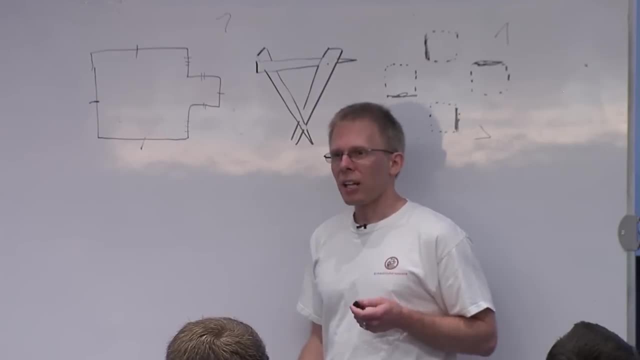 idea and i. so the author, nassim talib, wrote the, the book uh black swan fooled by randomness, and his more recent one was uh, anti-fragile, and he espouses a kind of interesting theory that i that i recognize from the way, a lot of the way i look at a lot of things, and the idea is that 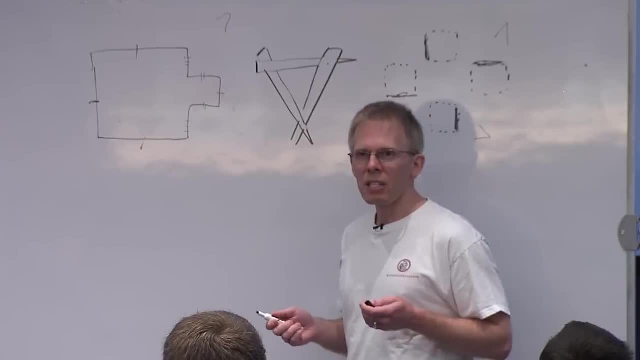 your best system is one where you can take great gains from the highs, from the winning solutions, but you are not damaged much by the lows. and that's the way i approach ideas. now, where i get an idea, i get the light bulb with a little moment of enlightenment there. 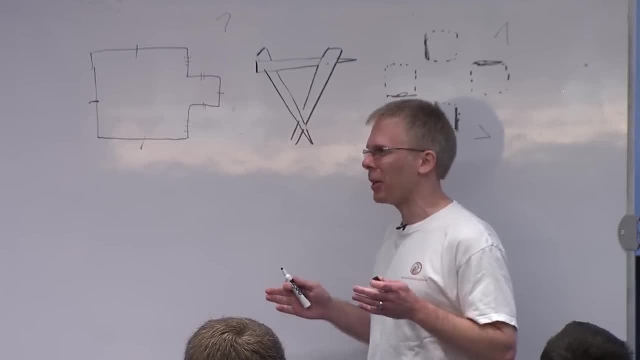 and joy. this is great. this is like the best time to be, you know, doing what i'm doing, having a brilliant idea, thinking it's going to be great, but i am already kind of slyly smiling to myself. it's like it's probably not going to work out, but it's sure fun while. 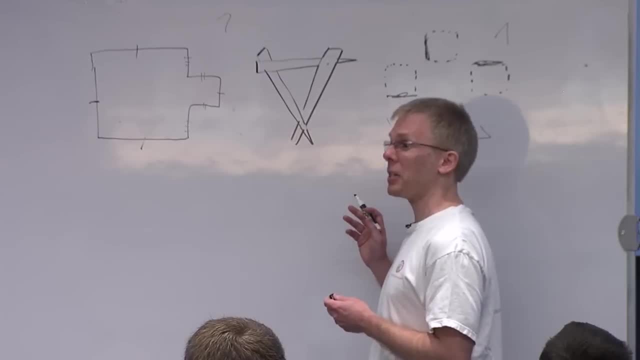 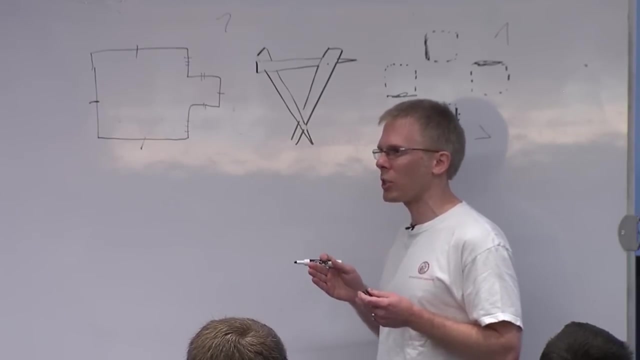 i'm having the idea and then hunting. the way that it winds up not working out is- uh, it's gone about- is an effective challenge where that's the best use of the time, where, if you're not trying to bust your own idea, you swerve away from the things that may wind up punching holes in it. i mean, you see, 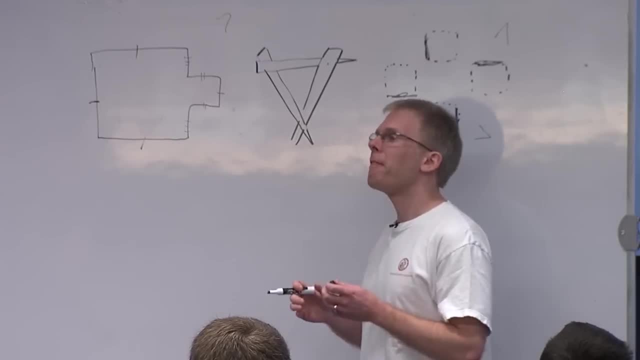 this in all sorts of things about how you know people when they're they're invested and attached in onto certain ideas. they will look at the things where it looks like the idea is working out, but not so much on the things that may punch holes in it or the things that that may challenge it in different. 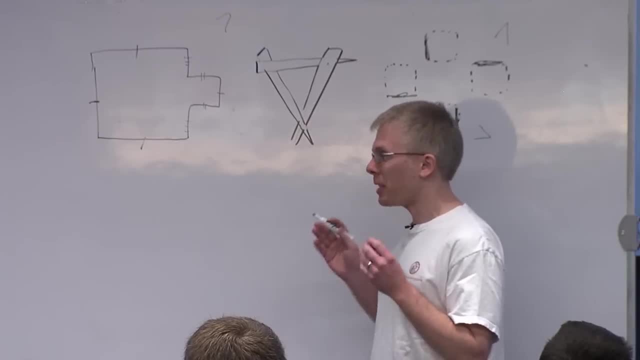 ways. so now i try to look at these things like, okay, get the joy out of it, but then really try hard to punch holes in my own idea here and that becomes almost an enjoyable task there and i can pat myself on the back when i break my own idea. it's like i'm very happy with showing clearly. 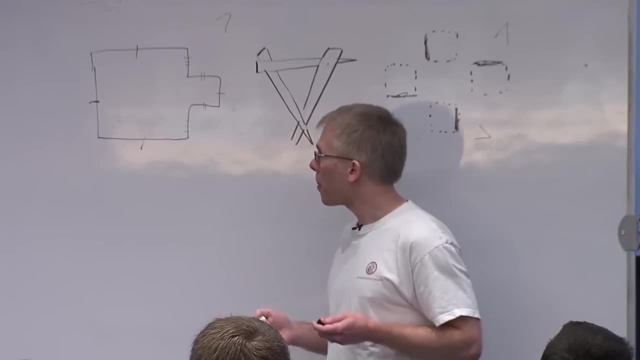 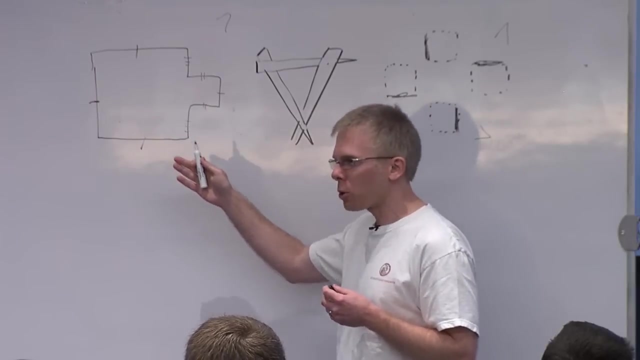 that this doesn't work, but these wind up coming from. you know i could trace the even on the broken idea, the depths of these things that went back to- i especially like, from when i first got into graphics work 25 years ago, and that's down to. 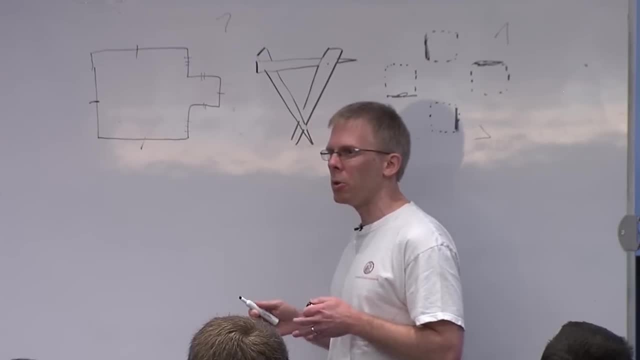 again the part about being down there in the mud working with the idea, and that's how you get these moments of enlightenment. it's working through, uh, you know, farming the ideas and the things that go into it. i have this argument or this discussion or lecture, even with some creative people, where 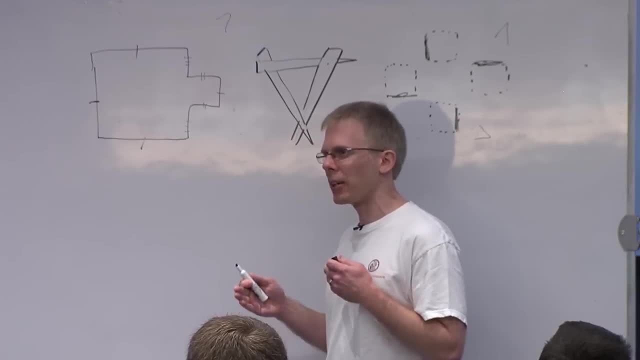 i would have some designers that i would talk with. that would be in kind of this: you know this funk, you know they're not getting their creative spark that they're looking for, their muse isn't with them in some way. and I will be brashly telling. it's like 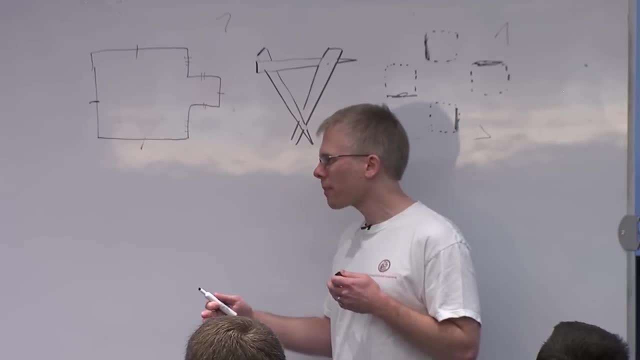 no, you can farm your creativity by just working through. you know, exposing yourself to lots of things, always looking at them through the lens of the problem that you're working on and plowing through, not staring at a blank wall, which I think our culture somewhat inappropriately does give this vision of. 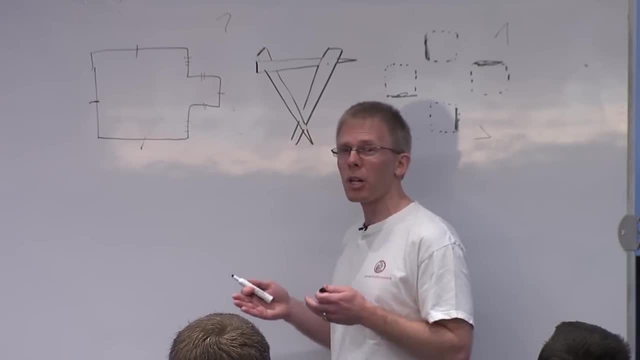 the genius that is just staring there doing the, the thought experiments, staring at a blank office wall, and that's how you get your enormous insights. and while some that does happen works for Einstein in some ways, but I think that it's far more productive to be just trawling through all sorts of 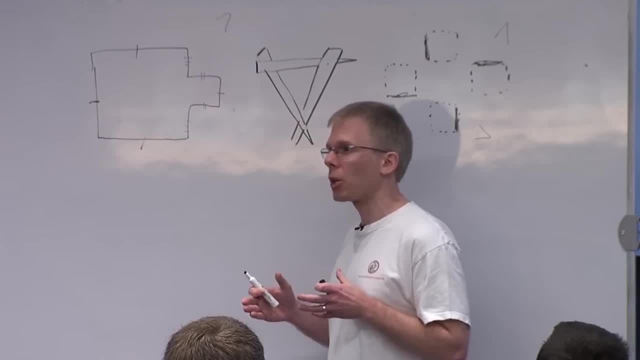 stimulus for the different things that you're looking on, looking at it through the lens of your current problem. I mean, sometimes it pays off and I sometimes, like I was recently reading the book the annotated Turing- I have a pet solds book on, kind of going through Turing's old papers, and there was talk about it. 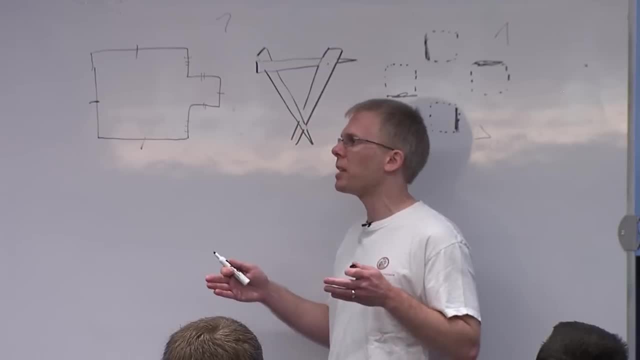 started going through something about how there's a mapping from the continuum to all points in an indimensional space, and I got hugely excited because there's all this stuff that I'm working on with or interested in with light fields and some of these other areas that are these high dimensional spaces that are very sparse. 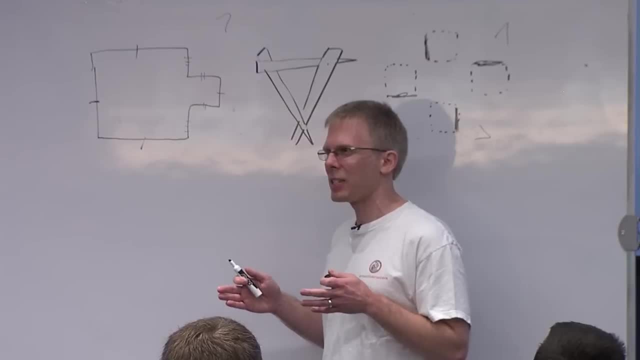 like: oh, and some new mapping for this would be a wonderful thing, this would be, you know, great. and once I deciphered, the mathematical language, unfortunately, was like: oh, I already knew that this is kind of just the bit spreading trick where if you have a, you know a sequence of bits. 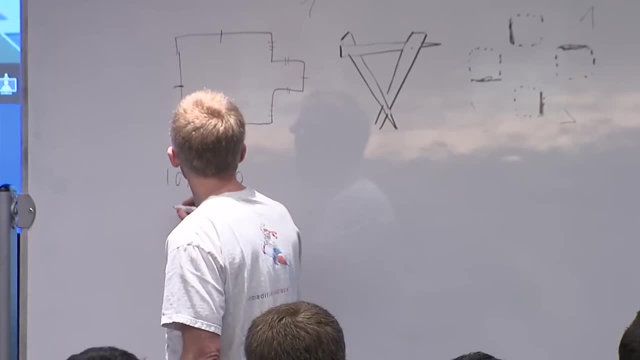 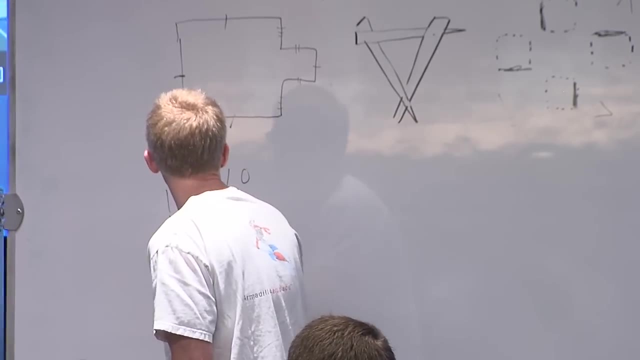 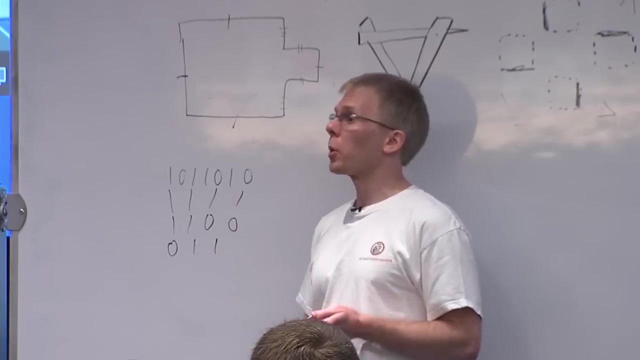 going off in some way. you can just turn that into a two-dimensional space by taking- I like every second bit here, making coordinates out of it like that, and you can do that for any in dimensional space. you can spread them out, but still it was one of those things where I was reading a book completely. 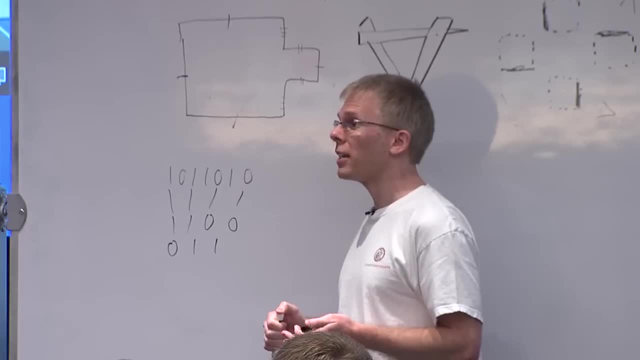 unrelated to anything that I was I. you know that I was working on and if I hadn't already known that, that would have been a good insight. that's something that's useful for a lot of cash- blocking things and different stuff like that- but I had kind of run across on my own. but that sense of being out. 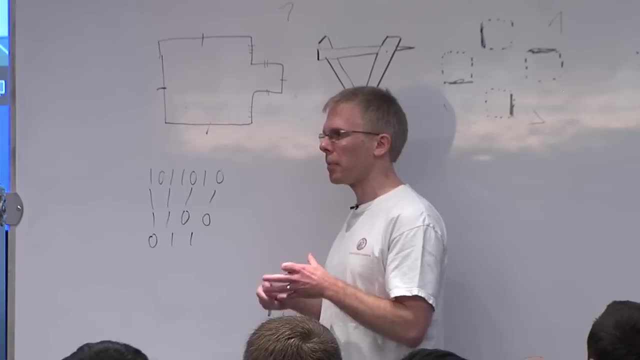 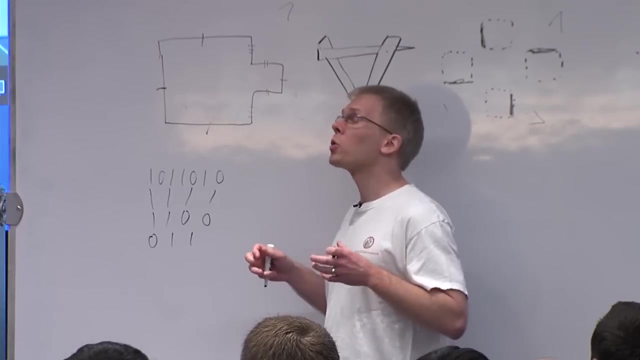 there searching for- not so much searching specifically for something, but continuously exposing myself to all of these other things and seeing what the current problem that I'm looking at, I applies to it, and I find myself more and more nowadays seeing this serendipity that seems almost- you know, almost- weird. 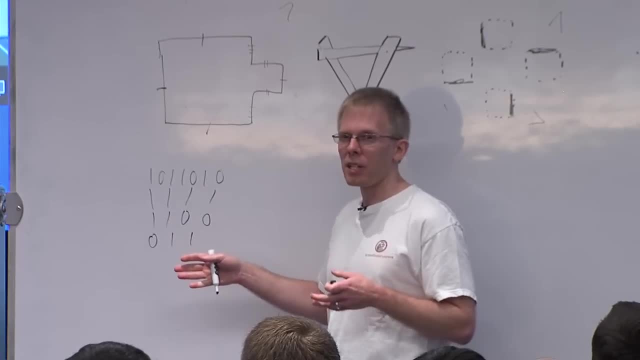 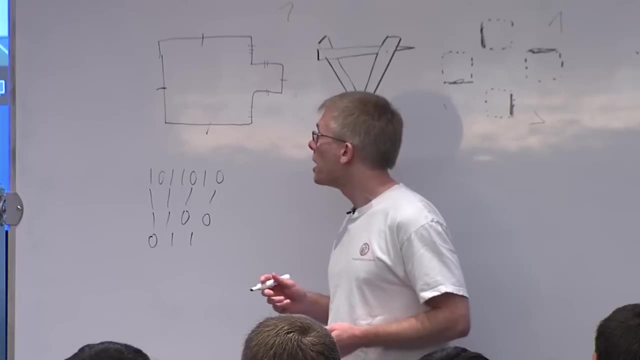 in some ways that I can be learning something in one place and then reading something completely unrelated and finding some reference to it or some tie between that, and then I don't know what to do with it, but I find myself more and more interested in that and that's. you know, that's been very interesting, but the 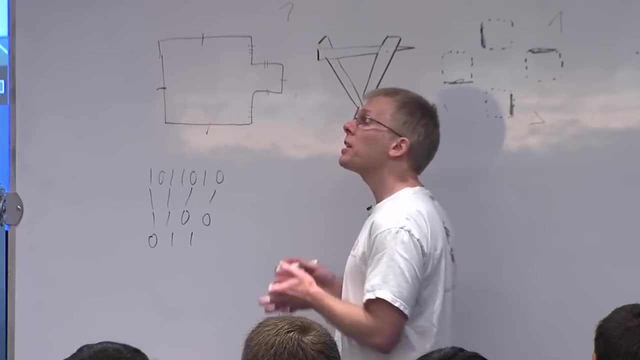 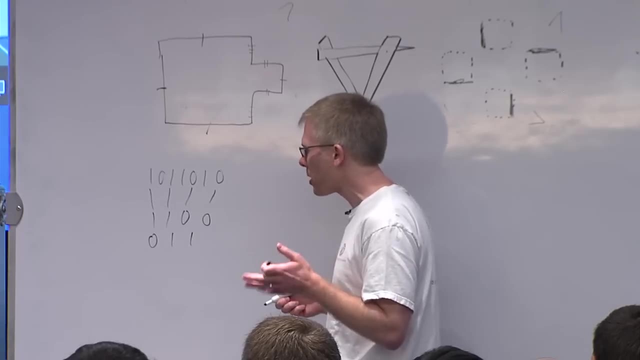 problems have been like different things. one of the one of the significant problems with virtual reality- and this was the first idea that I forwarded to Michael right after he had sent me this- I'm, you know, the original email there- one of the things that you've probably heard people talk about in VR is that we 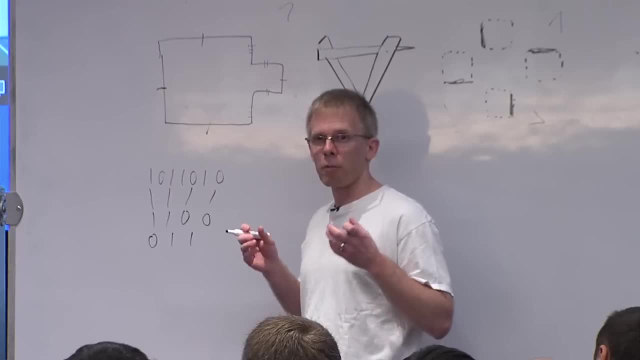 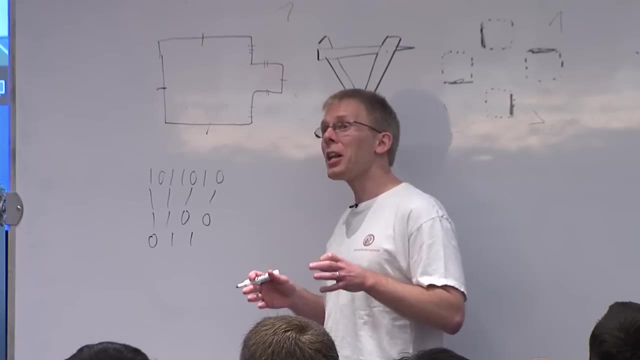 need 16 K by 16 K displays to kind of really give retina class resolution for reality. I am- and historically you look at that- say clearly, while we could actually use virtual reality, we could use virtual reality, but we couldn't really build that with like wafer scale integration of silicon micro displays. I 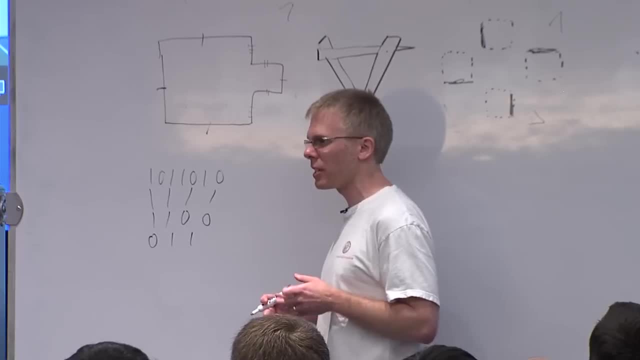 that would be kind of an interesting thing. we couldn't render that in any reasonable system today and really that's not the direction that things will eventually get. it's not nearly as bad as that seems, because the eye only has that resolution in a very, very small area called the fovea, and several of us 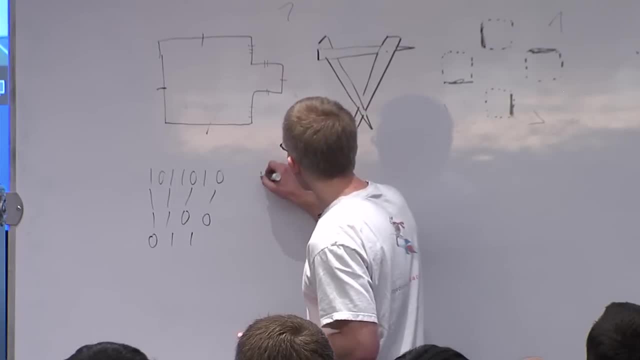 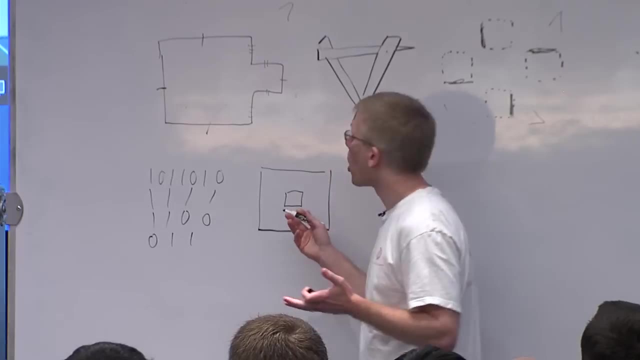 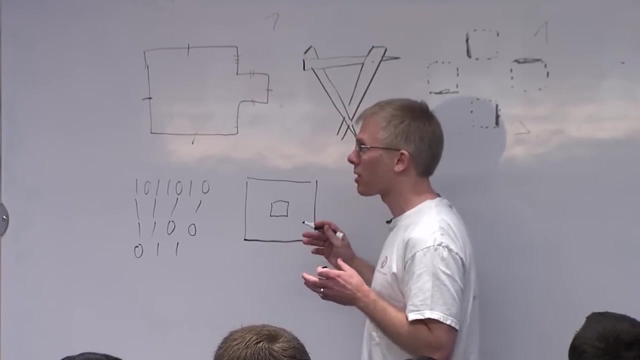 have done research and prototyping where, instead of rendering the entire screen at a super high resolution, you render the screen at a low resolution and then you render a smaller inset area at a higher resolution. this works and is useful even on our systems today, because our optics are not great across the entire field of view. they're clearest in 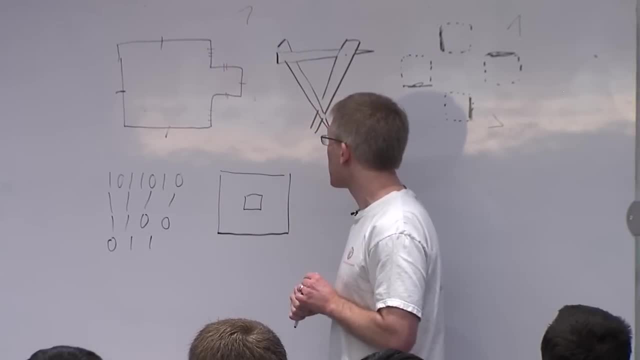 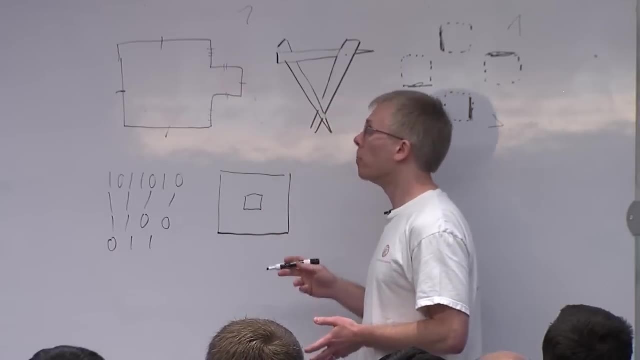 the center and they're blurrier as you go out. so there's some argument that doing this sort of rendering today is even a good idea, and this is one of the reasons we've been pushing for the multi-view extension, which is a way for us to kind of push all the draw calls for a scene down and then 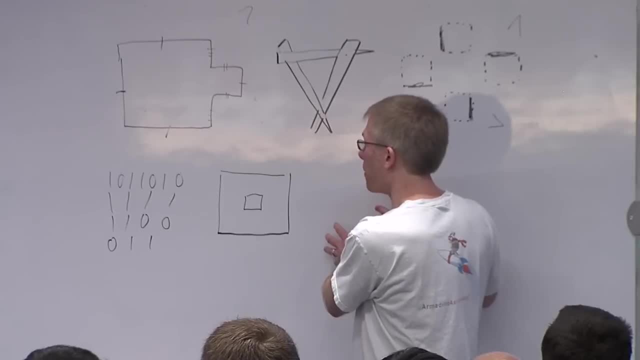 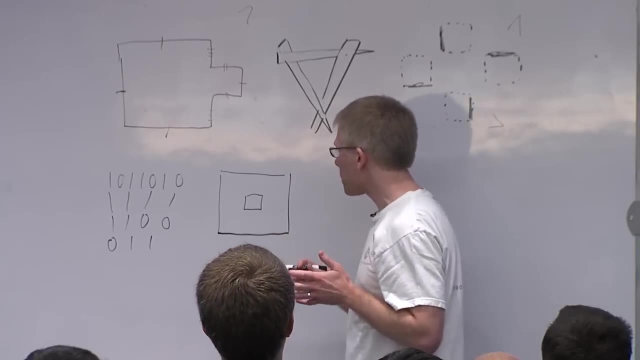 have the driver and the hardware, reissue those to make a second stereo eye view and ideally then a second foveal insert and another foveal insert for the other eye. so this is something we've been kind of pushing on for, you know, for a while. 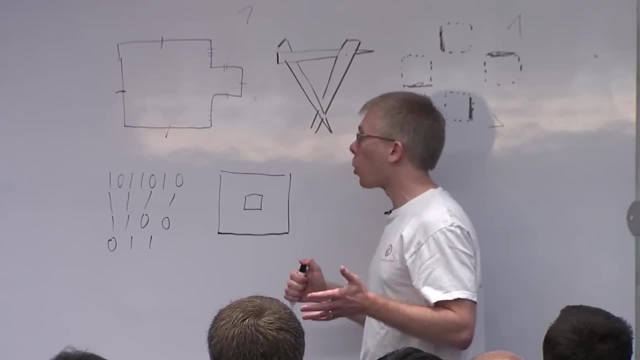 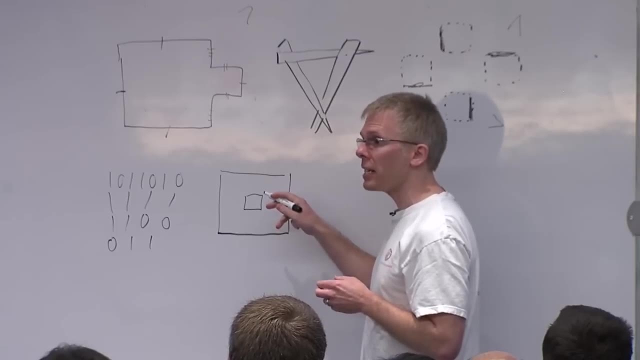 but the the magic screen that we want- and there's work being done on this now- would be something that could track your eye and then move this region around to exactly where it needed to go. that would be something where you could deliver, hopefully, this retina class resolution by having 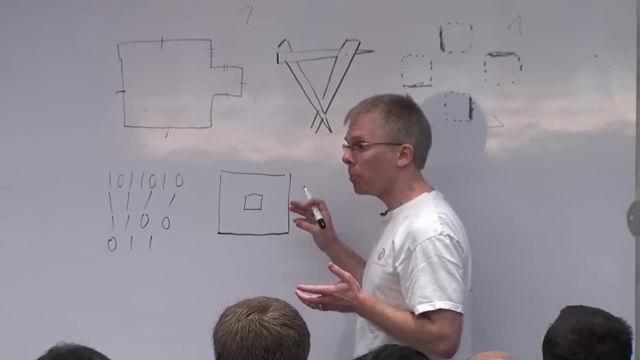 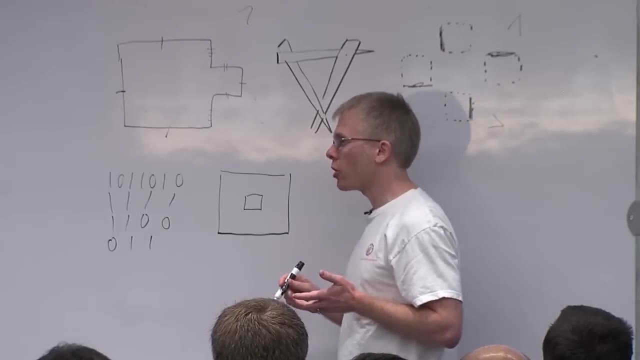 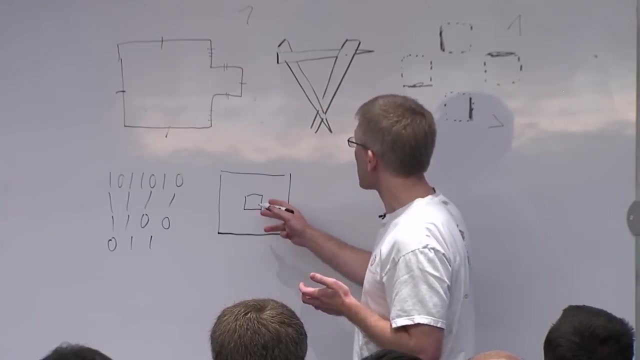 only this tiny little area. no screen like that exists now, but we have people that are working on technology that may get us this maybe sooner rather than later. so there's still the question of how you wind up delivering all those bits to it and rendering it. a few of us have built systems like this, where you 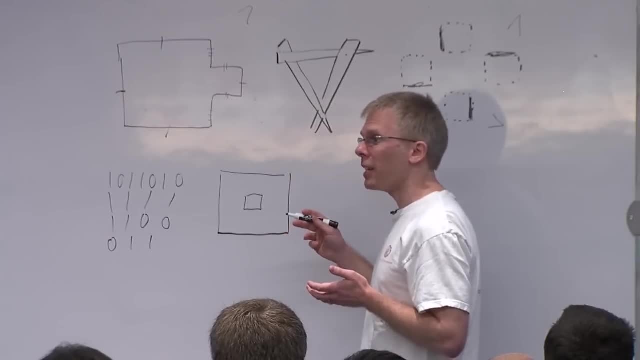 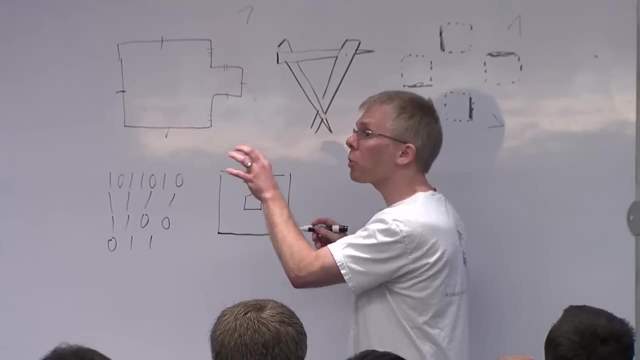 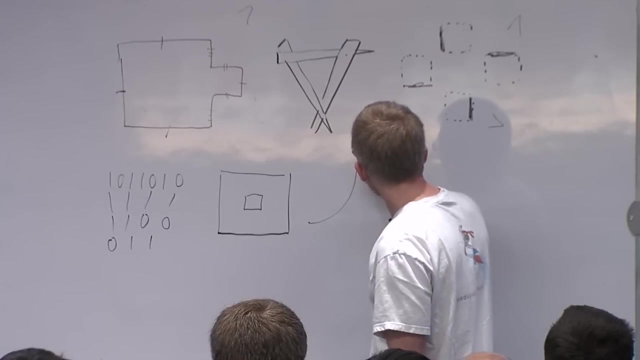 render kind of two separate views. but we talk about the fovea as if it's this fixed little region like: here is the fovea region of your eye and it occupies this many degrees of arc. but it's really not like that at all. uh, if you look at the wikipedia graph picture for it, you wind up having a you. 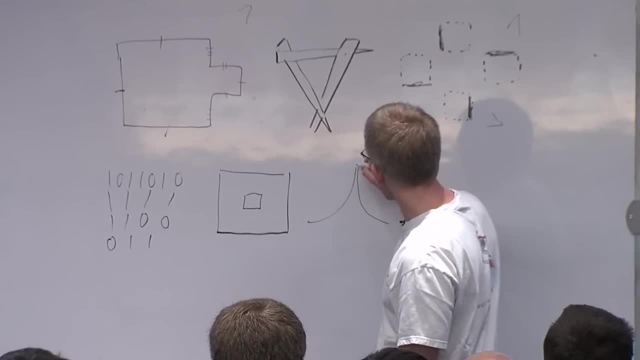 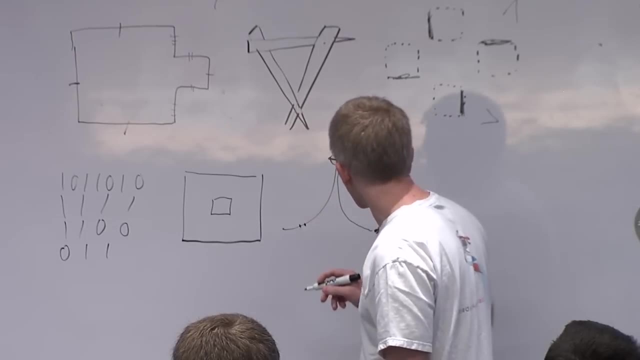 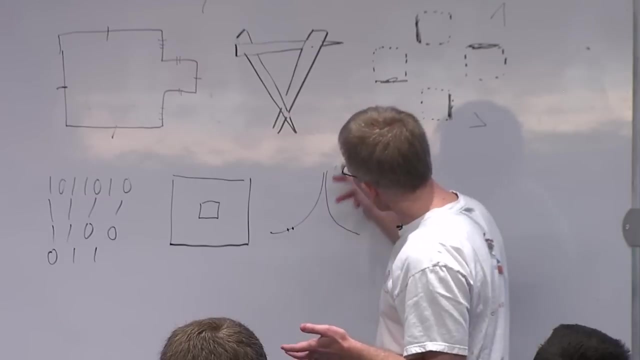 know something that looks kind of like this for the resolution of the fovea, where lots of resolution right here and then a smooth curve going down, with like one little gap where you've got your blind spot, where the, the optic nerve kind of goes in. and looking at this it occurs to me it's like well, you know the shape. 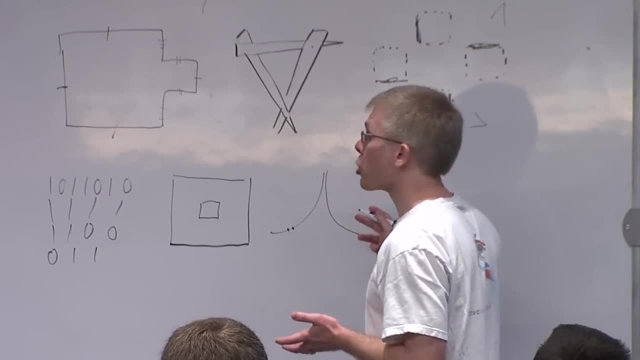 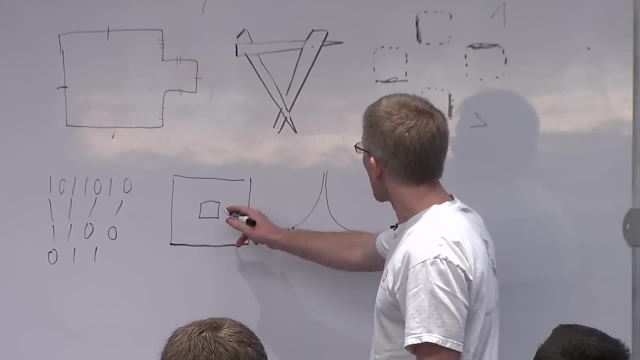 of that curve that looks a little bit like I'm like a projective, like a projective texture mapping curve. you've got to divide in there somewhere. and I start thinking about this again where, if you had this two-step thing, then you're looking at saying we have 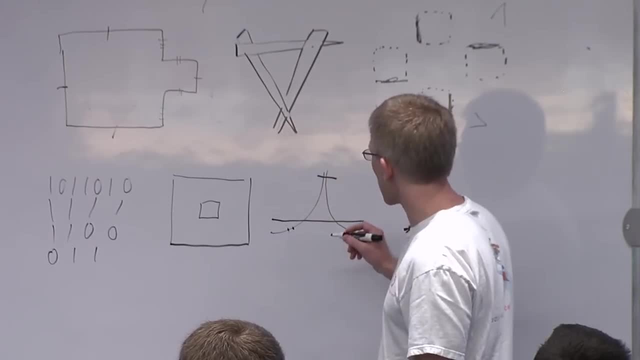 one image at this resolution and then one image at that resolution and you can sort of take the integral of the difference between there to see how non-optimal that would be for what you're trying to do. it's still a whole lot better than picking one average sort of across the whole thing, especially if 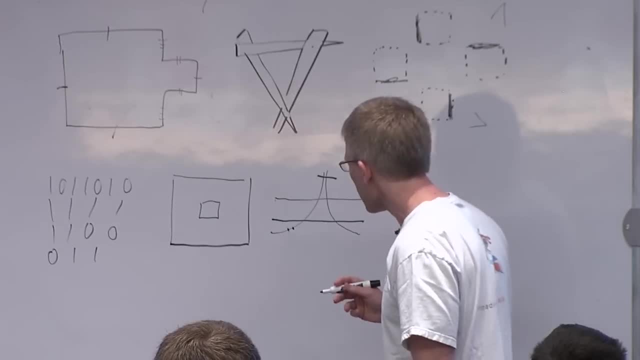 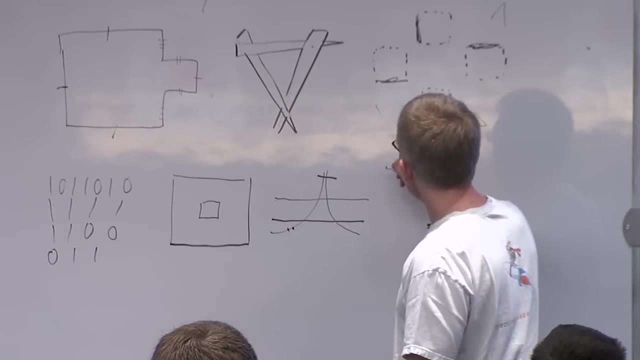 you want to get a lot in there, but it's not really what you'd like to have. so I start thinking about how else could we address to build some rendering like this? and one of the tragic things about the conventional graphics pipeline is: the wider you make the field of view, the 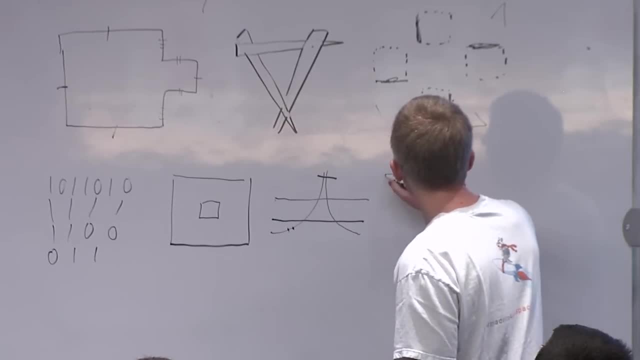 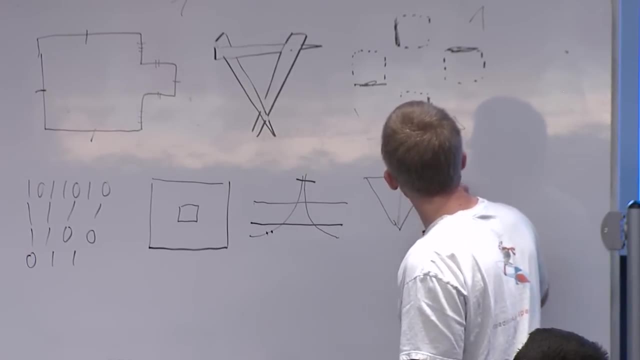 worst, it puts the pixels in where, if you have a field of view something like 80 degrees or so each pixel on here, it's not too far off between the angular resolution, what you get as it goes over here and what's in the center, but the 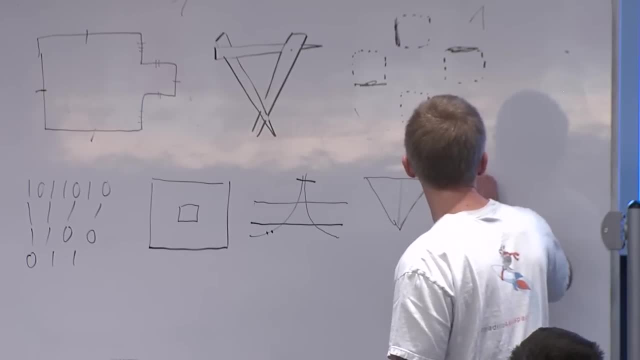 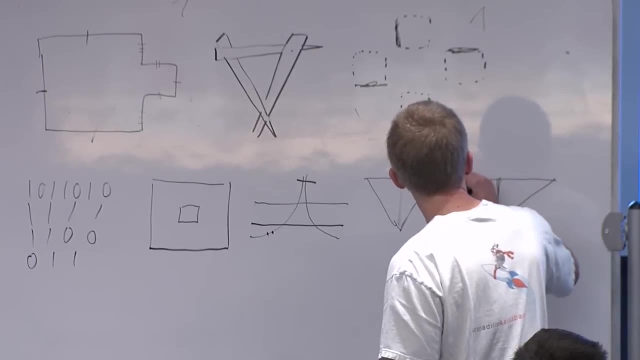 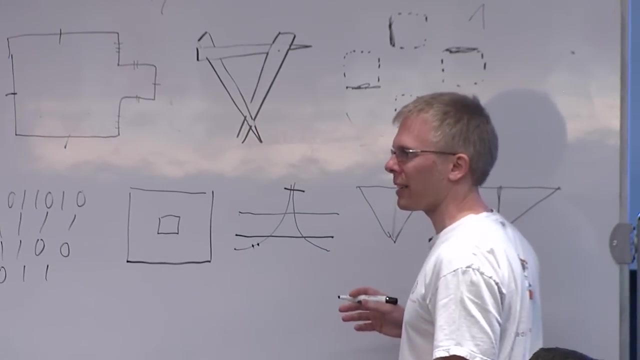 wider you make it, the worse it gets. if you go and you render 120 degree field of view, something where it's like that, at that point, the pixels over here at the edge, you actually have much more resolution on the outside, which is exactly where we don't want it. it's doing the inverse of 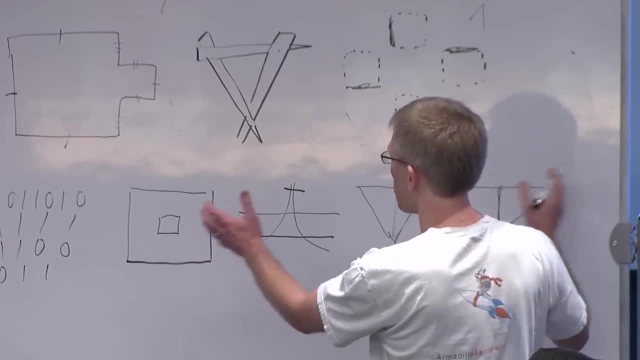 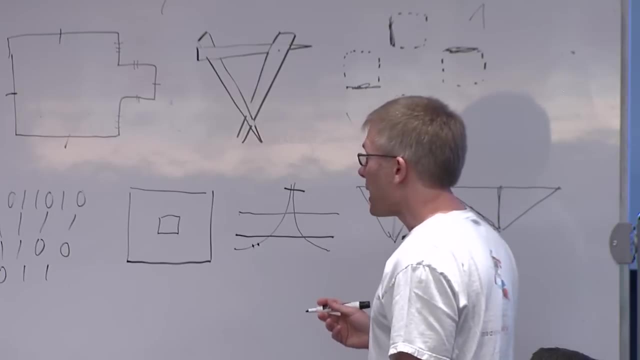 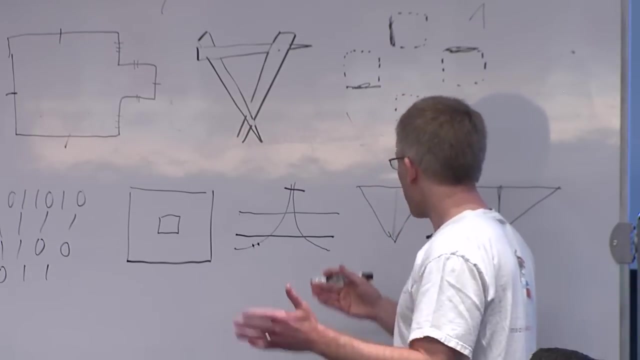 what we'd like to have, which is what pushes us to saying it's like, well, we'll do the whole broad thing at some low resolution and then we'll do a tighter inset, but started thinking that I projected Geometry might be able to help help us with this, and this is something that i- i think a lot of people may take some heart. 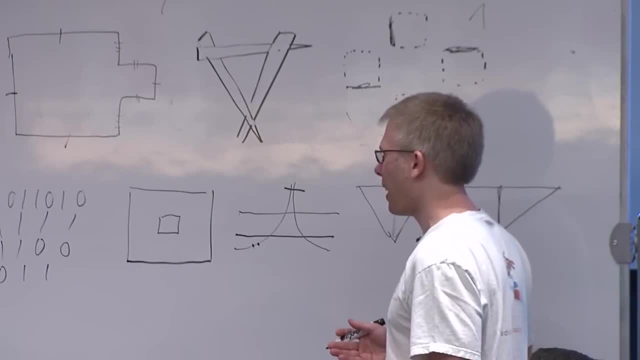 from this, but a lot of the, the math, the heavy math in projective geometry and, uh, you know, a lot of the higher end math. that goes on. it took me a long time. there were many, many years, a decade, when i was considered this graphics guru genius, when i really couldn't do from scratch a lot of. 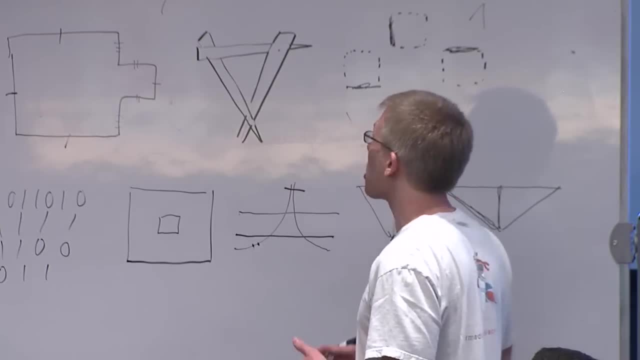 the. you know a lot of the mathematics that underpins a lot of that, but slowly, eventually, with a couple decades of experience, most of it did eventually sink in on me to to be able to do, to formulate some of these things more directly, and what i started thinking about was: well, what 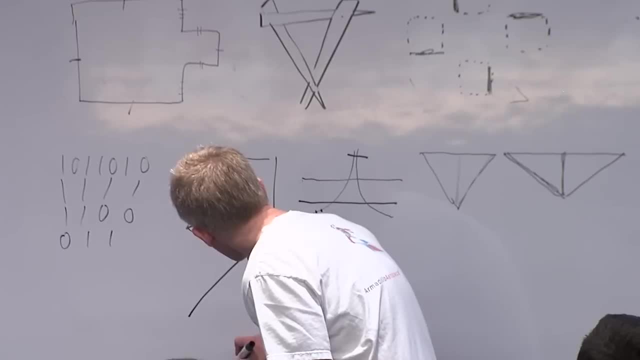 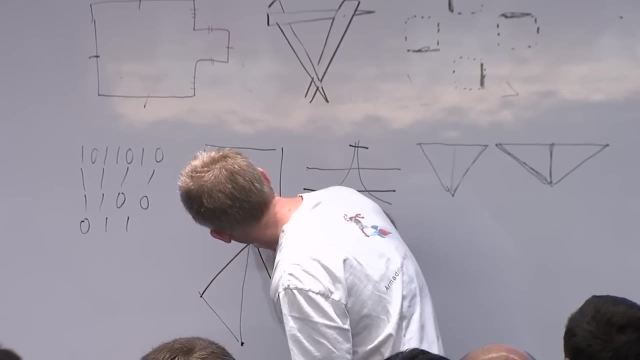 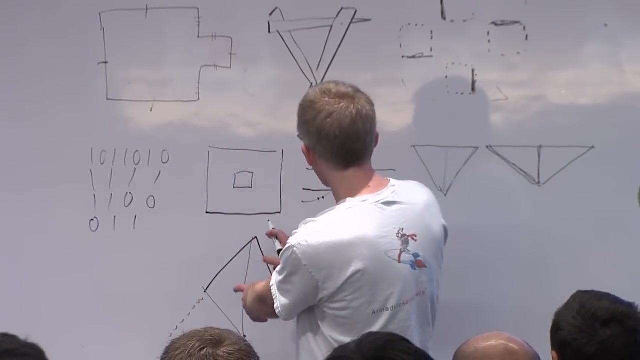 if you had, if you have a single view that projects, instead of projecting normal onto the surface, you're projecting kind of off-centered there, which you could think about this like: well, it's almost like you had the whole screen there, but you're only taking the the end of it where it's stretching. 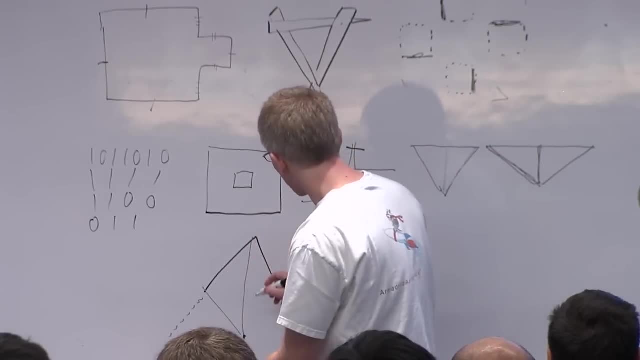 you're only taking the the end of it where it's stretching. you're only taking the the end of it where it's stretching out in the wrong direction that we want there, making it the right direction and then doing the entire way. so you're looking down, sort of at the corner of something. 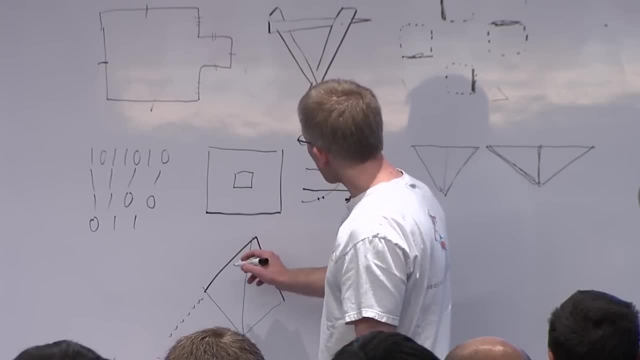 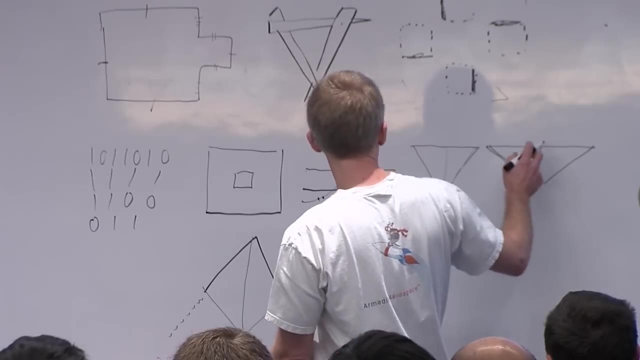 it would be rendering once that way and once that way that winds up giving you the direction of the, the compression of the angles going in the right direction. it's taking what's doing the opposite of what we want there, turning it around and making it do what we want. 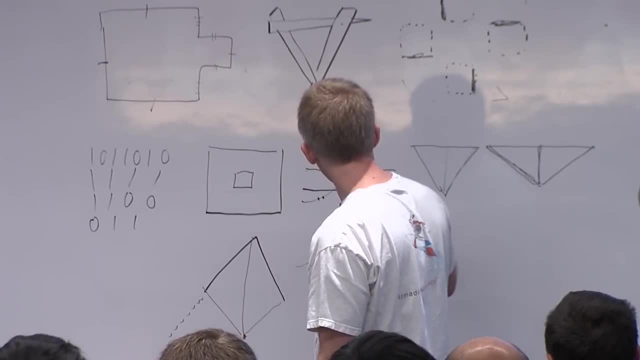 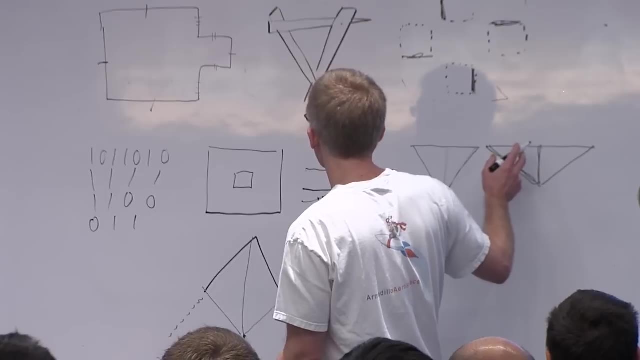 there so that winds up getting something that that kind of curves up gives you an increasing curve. so that winds up getting something that that kind of curves up gives you an increasing curve there. not an enormous difference, you know this. here goes maybe a factor of two off from what you'd. 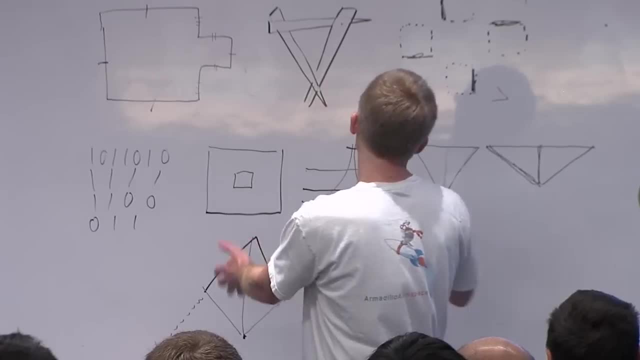 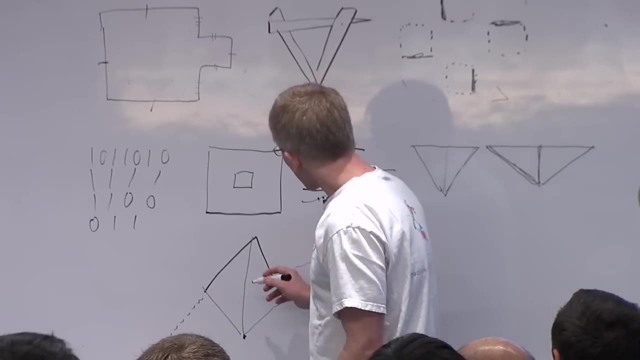 like to have. but this makes it a factor of two in the right direction, which makes it a factor of four better than what we would have from our conventional rendering. and a factor of four is, you know, is nothing to sneeze at, um, but then you'd say: well, what if you wanted? 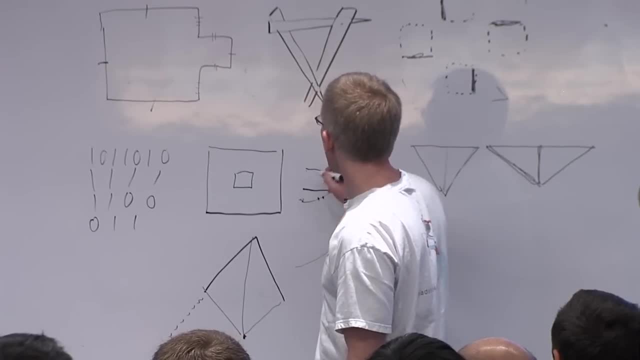 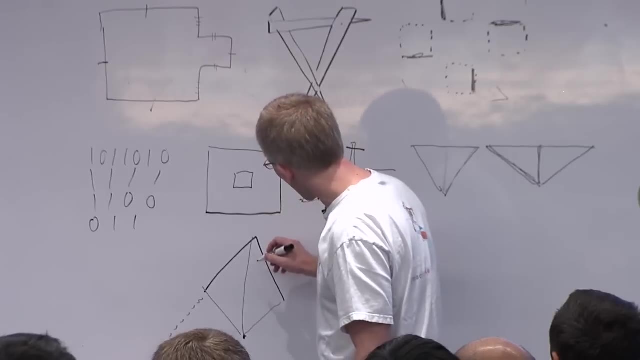 this is. this goes down by like a factor of a hundred in the total case, from the very outside to the very- uh, the very top it's. it's much larger. well, maybe you could start stretching this out. you know what happens if you, uh, if you stretch it out to something extreme like this, you can build. 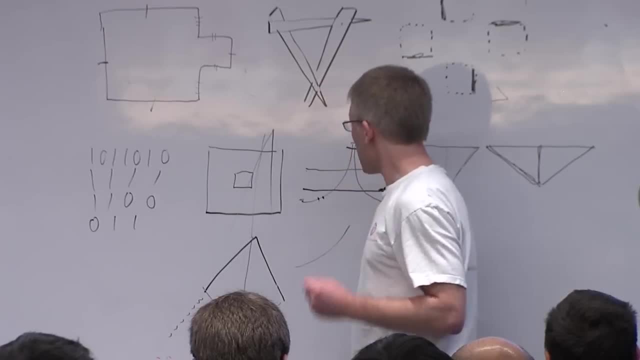 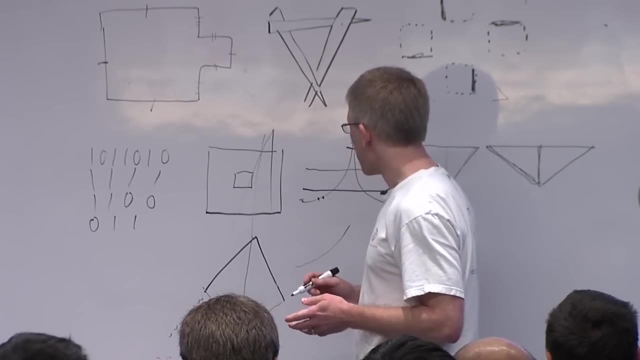 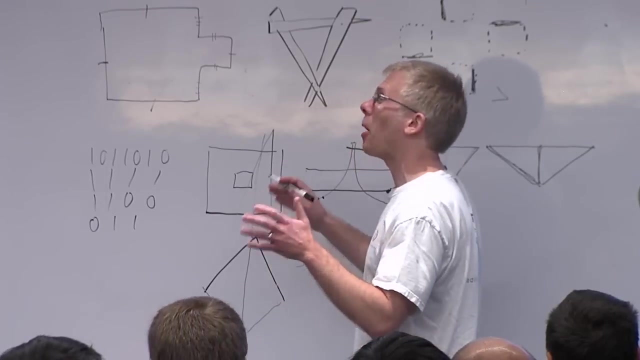 any amount of angle that you want out of that. so this seemed, i, like an interesting idea. this is one of those ideas that i has direct impact on what we're doing. i may have some real value to getting this. this big thing, the retina class, uh, virtual reality display- i mean the hardware people have. 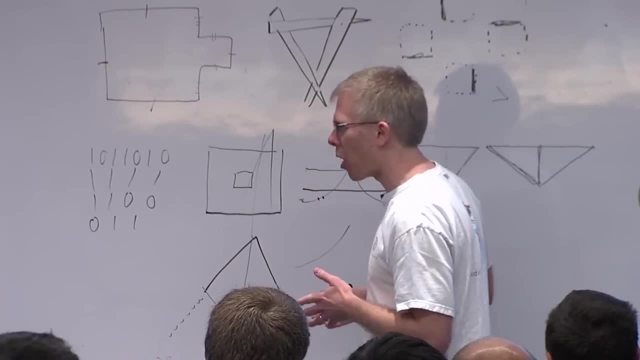 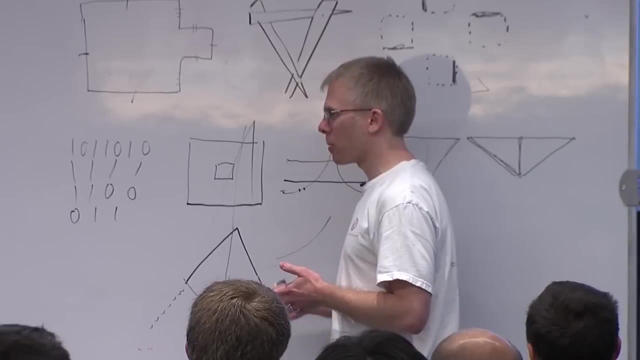 to figure out the magic to make it happen and focus. but this might be the software side of things. so i'm it seems like a good enough idea, i start, so i i take the steps to try to bust it. i go ahead and i write the you know, i write some, make some checkerboards and render the images there start. 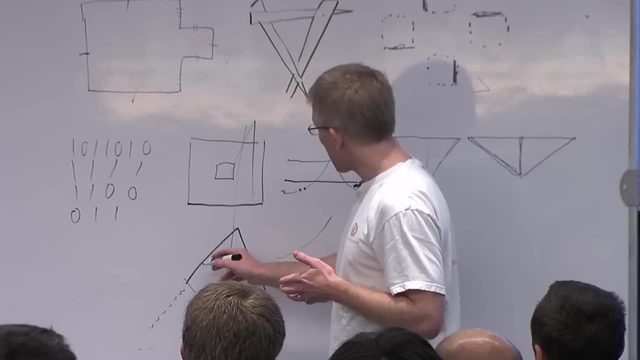 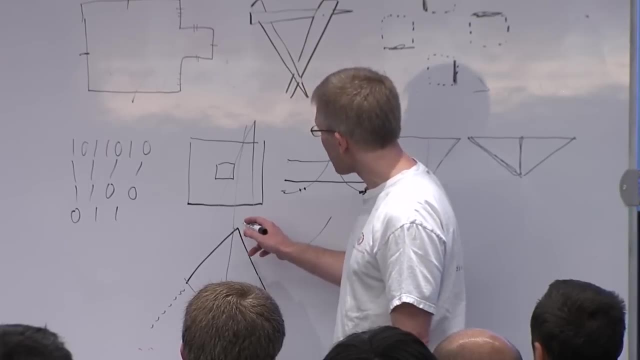 putting some images on it and it looks really pretty promising. looking at the corner of a cube, i get tripped up a little bit because the three-dimensional aspect of this is not the same as the two-dimensional, where, looking here, it's clear how everything breaks down. but 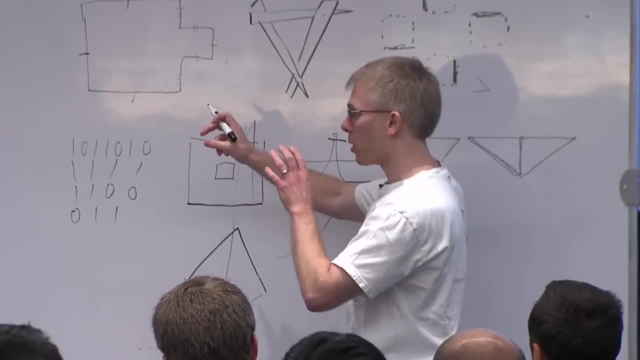 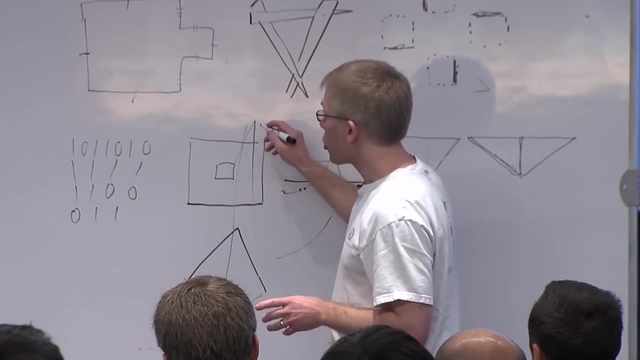 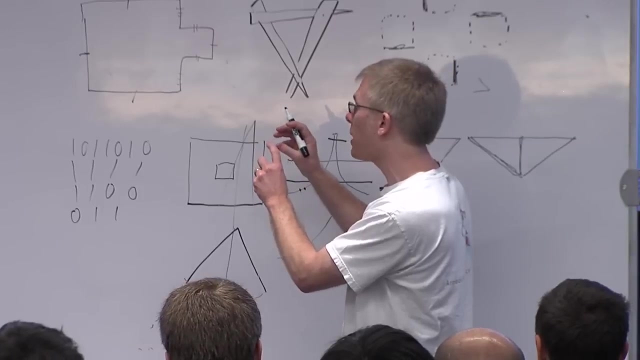 looking in three dimensions. you've got a degree of isotropy as you look down into the corner of a cube, but still it looks pretty good. stretching it out starts to show some issues where the pixels then get very distended and there's a degree of anisotropy where the core center of it, where your fovea would be looking, is extremely high pixel. 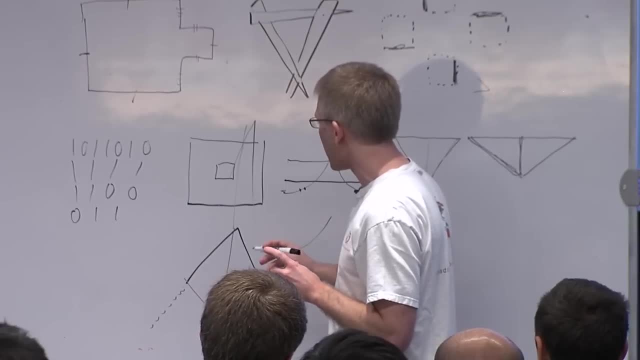 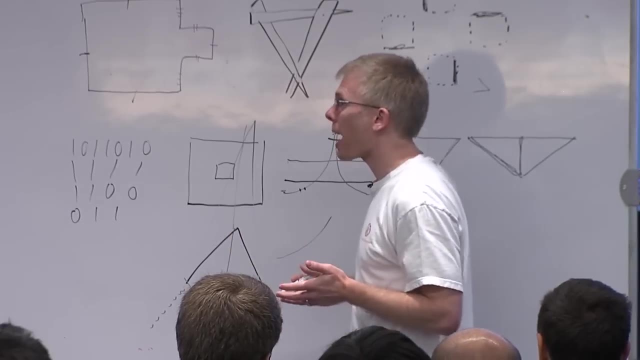 density and could get up to very much what you'd like to see like that. but on the outside you've got these i very stretched out pixels and i don't know whether that's uh good or bad or a problem or not. that's something that might not be a problem because that's inherently what you're not looking at. that's something. 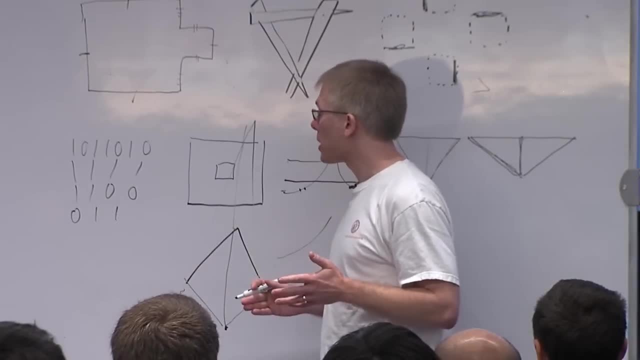 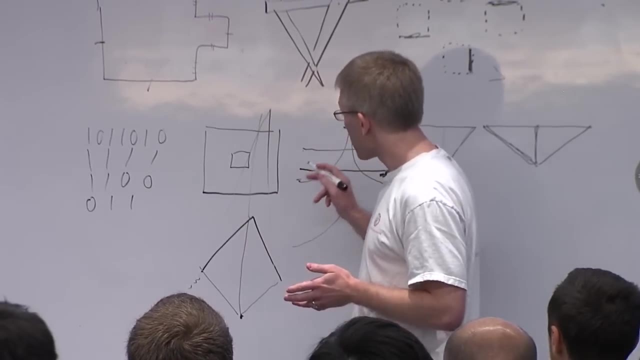 that's only happening at the edges. if they're well filtered, maybe that's a good enough idm. but even if it only works out where you don't distend it, you just leave it at the cube. there are some gpus have hardware support already for distributing primitives across cubes mostly. 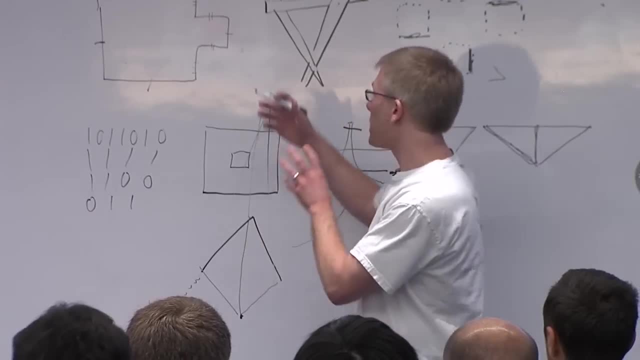 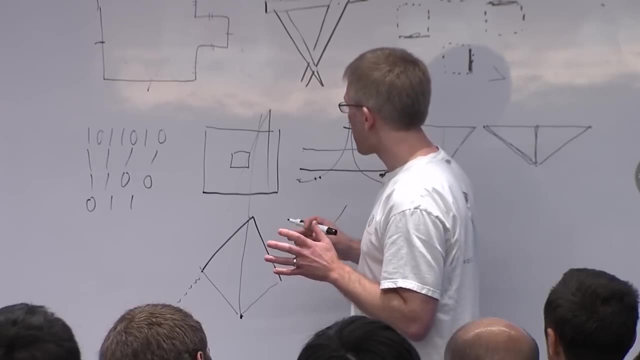 for rendering environment maps. so if you say, well, we're going to take the three sides of a cube here and we're going to push one stream down, it can split them all up. that seems almost optimal. maybe that's only a factor of four better than what we're doing now, but factor of 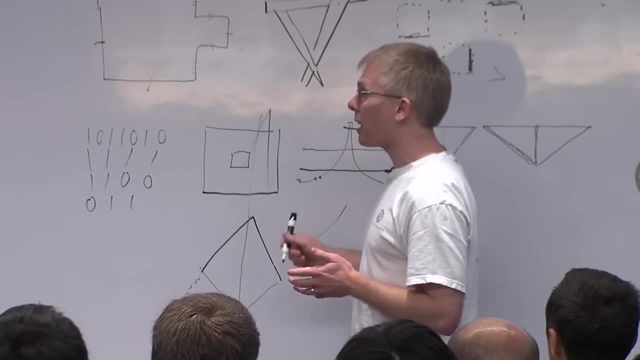 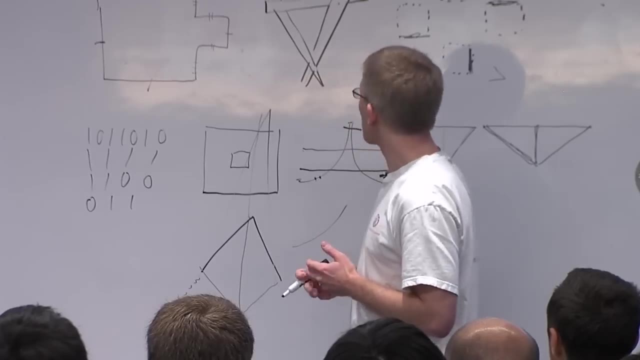 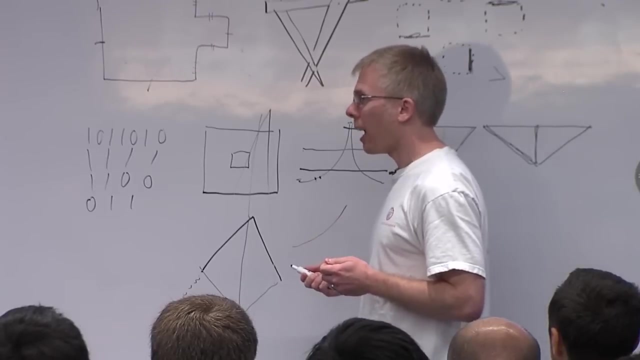 four is a pretty wonderful thing in a lot of cases. so this is an idea which i'm at least cautious i'm about may be a great idea. this may be something that you know that has some real significant win to it, and i i noticed that i feel good when i try to attack the idea early. i see this where. 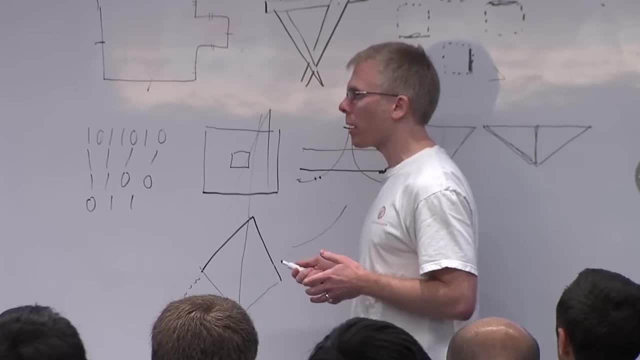 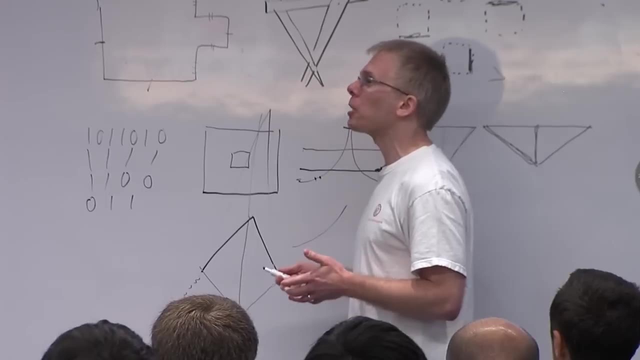 ideas that i have that i don't try to engage and grapple with quickly. i find myself falling into more of the pet idea side of things, where i have this problem a lot now with i'm not actively building rockets, but i still think about aerospace stuff. i still think about, uh, all this stuff when 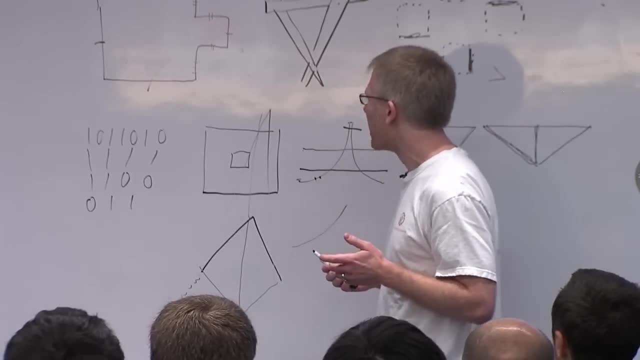 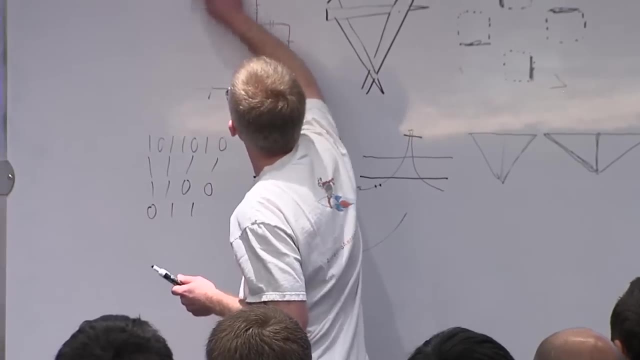 i'm trying to go to sleep some night, having rocket systems dreams, whatever i'm. but that's problematic because i don't have the shop running where i can go and build and test those things right now. so i wind up getting ideas and they sit there and they churn around in my head for a while. 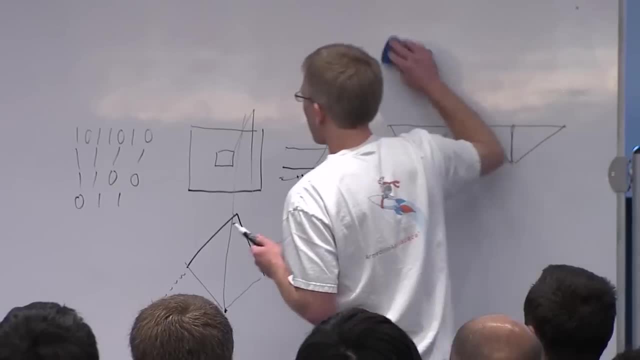 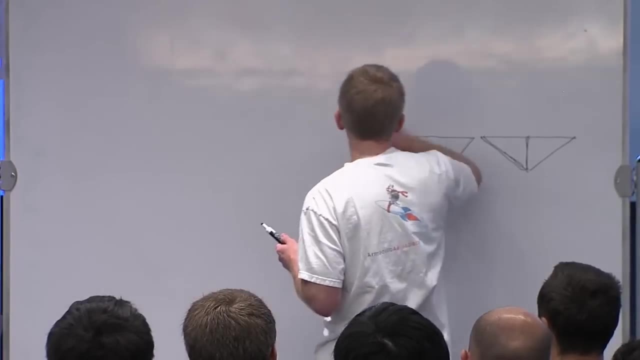 and without testing them, i get a little bit attached to them. they're like my, my pet ideas in some ways, and i think that i fall into some of the same traps that i you know, the the people that wind up emailing me about the things, wind up thinking, for instance, i'm 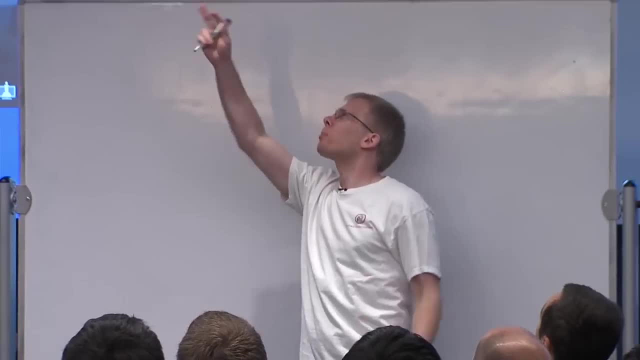 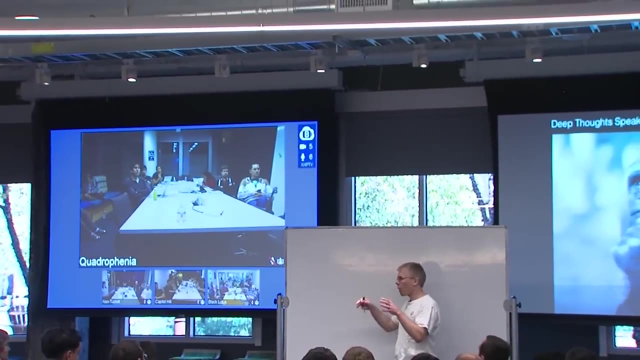 well, one thing just: every time i look up at ductwork, i see spiral welded ductwork. and this is done by you. take a strip of metal and instead of forming it into a cylinder and welding it in different ways, you have a machine that winds it and makes a continuous weld. and now that's. 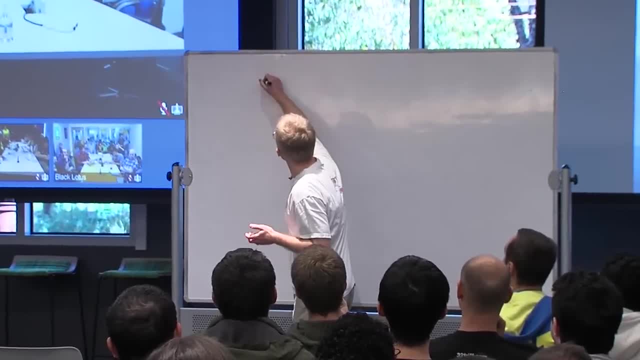 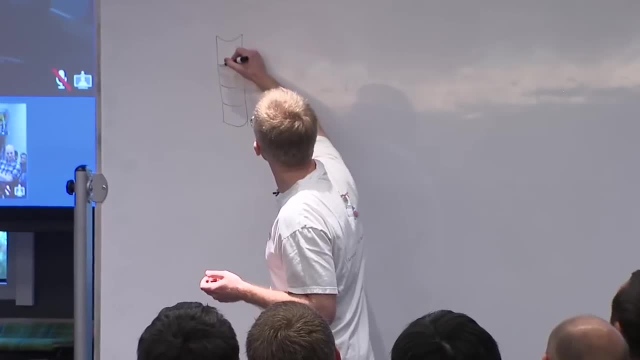 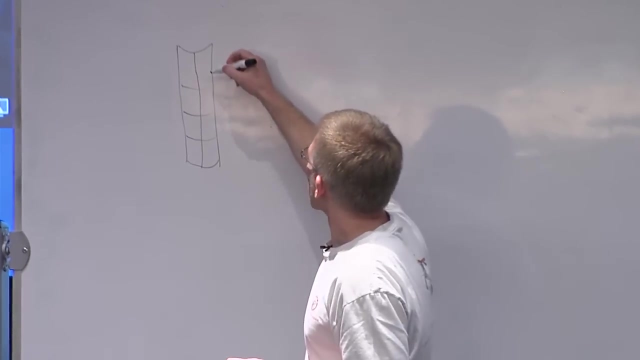 an exciting thing from like from a rocket engineering standpoint, because normally when you make a cylinder you have- if it's a long cylinder, you've got welds like this, and then you have one weld that goes down the side. now the problem is: is that in a cylinder you've got twice as much stress? 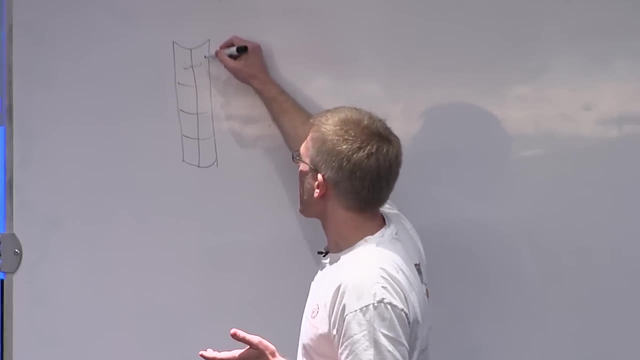 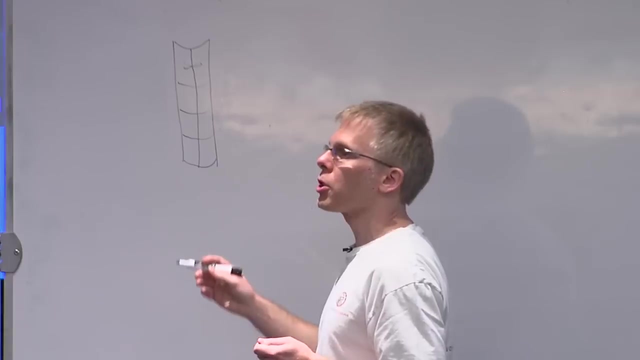 going this way as you have going this way. and welding always impacts the strength of things, so you have a super critical well going down there. so you get companies like spacex that do very nice stir welding to try to make the best possible things, but if you spiral weld it, then all of 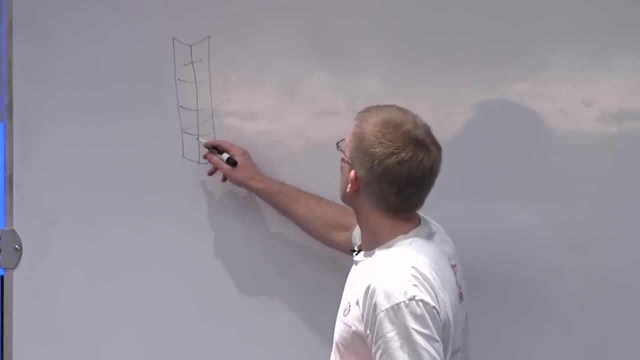 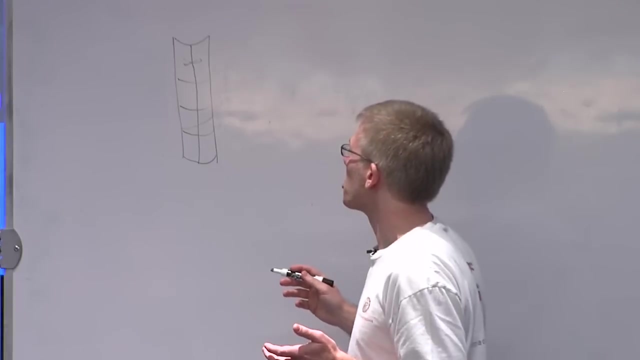 the welds are at a small angle like this, which is you've got twice as much strength going this way. so even if the weld de-rates by 40 percent, you still have a really good solution, and plus it's really cheap, which is why they make ducts out of those. so i wind up thinking about all these. 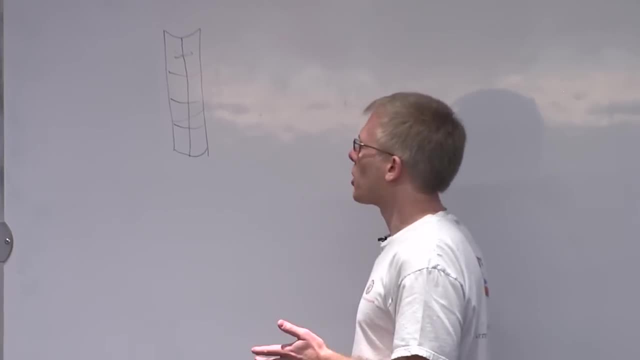 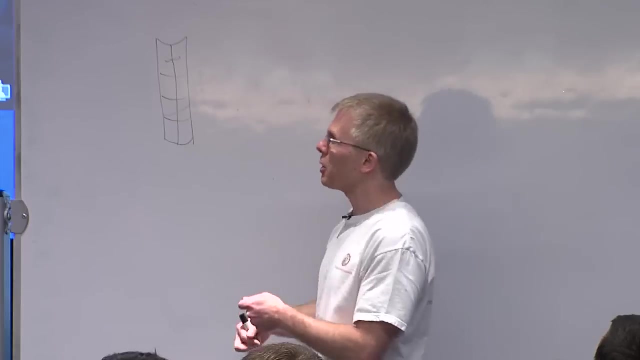 ideas about how okay we should just let's take some merging steel and roll this through here, get that worked out, and then you've got a great system that can be built inexpensively or even on site. you can build enormous things like this. maybe you can spiral weld a saturn 5 tank on. 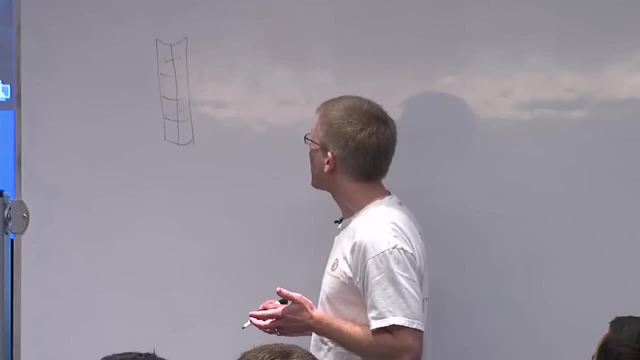 site where you're going to launch it, or on a barge or whatever you need to do with that. maybe it's even possible to to gently adjust the angles to make tapers to be able to make, you know, actual cone sections from there to make a one-piece mono propellant based, i you know, launch vehicle tank. 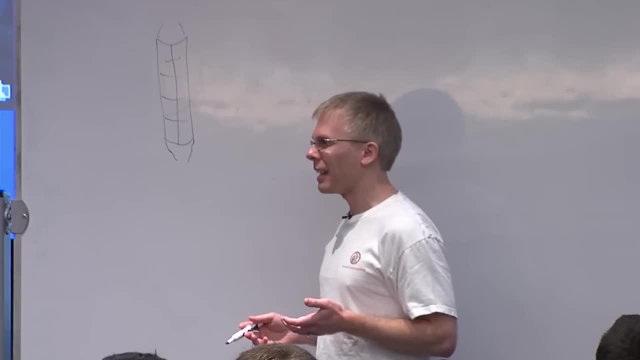 and this is an idea that i've actually been kicking around for a while, and i'm it's probably going to be years before i wind up getting around to testing this, and it's so that's not as valuable of an idea in many cases because i haven't been able to test it. 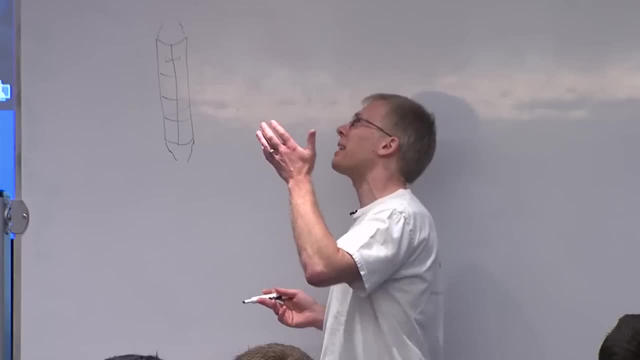 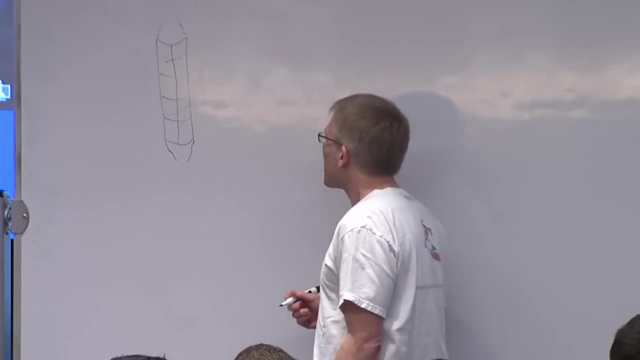 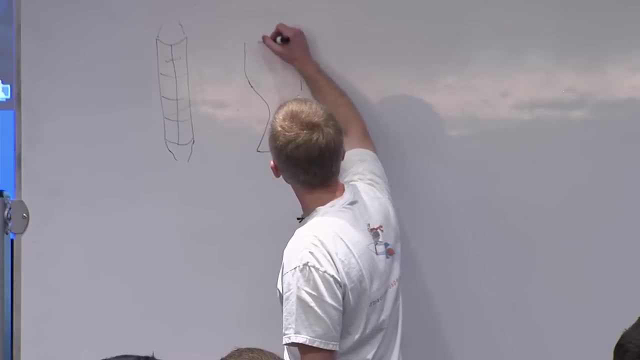 i probably won't. i have a fondness for this idea and i get reminded of it every time i wind up looking at exposed infrastructure. i am, but then there's other things like i'm. you know the way a rocket engine works is i. you know you have a combustion chamber. you know you make hot gas. 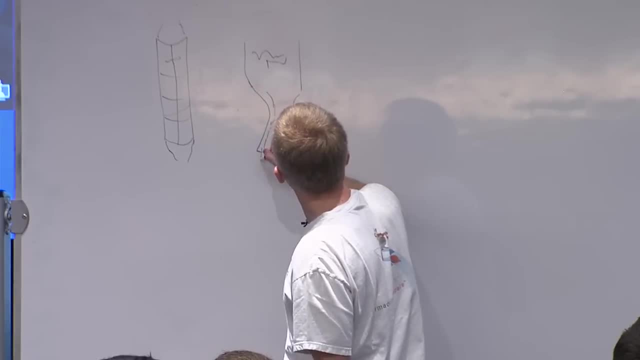 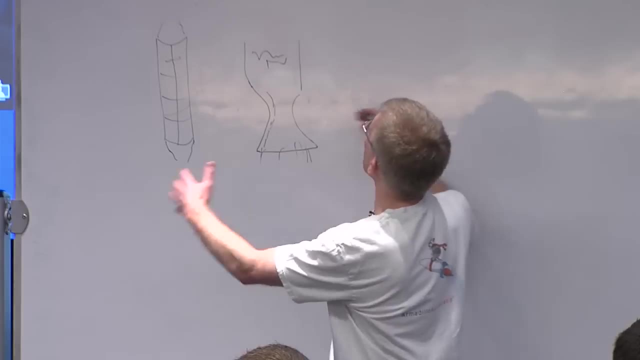 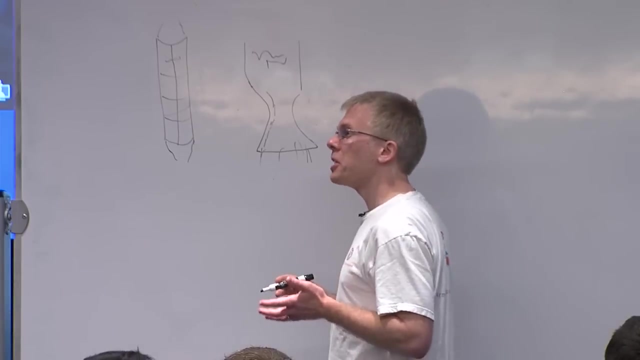 up here and it expands mostly through and accelerates and converts the thermal energy into kinetic energy coming out, and there's all these issues about how i, you want a large expansion to accelerate it, but you can't do that inside the atmosphere. again an unrelated thing comes up. i read some statistics about muzzle velocities of battleship guns and there's an 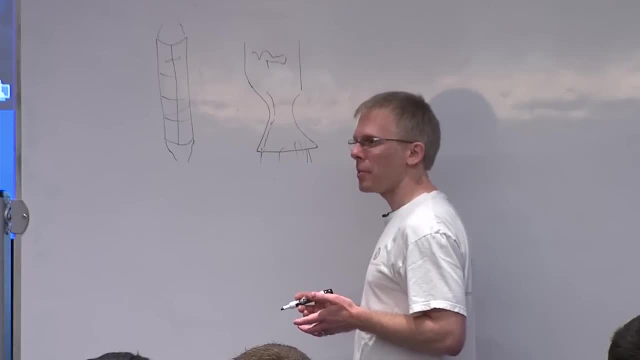 interesting aspect about that, where they can fire at several times the speed of sound, even though the charge that's firing a, you know the shell is less than half of the full munition weight there and you run the numbers from the traditional rocket equation and they're going faster than. 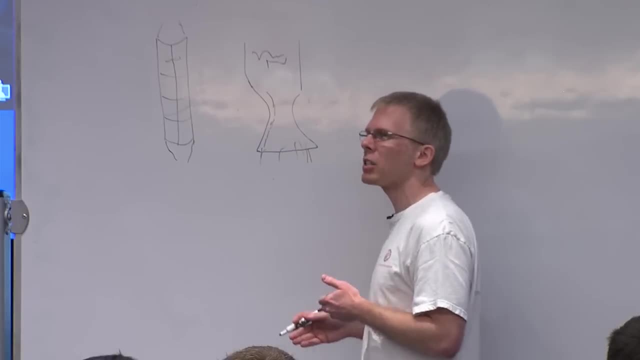 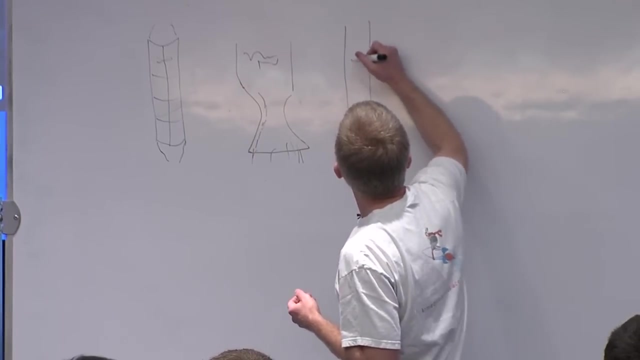 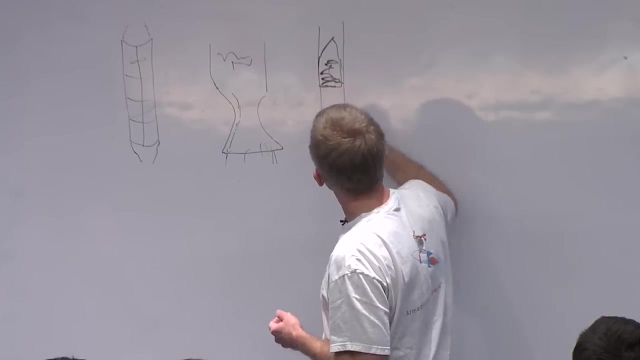 than they should be if it was a rocket with that amount of propellant of that isp. and it's for an interesting reason, a when you have a, a gun, you have a whole bunch of propellant in here. with a rocket engine, propellant comes in and 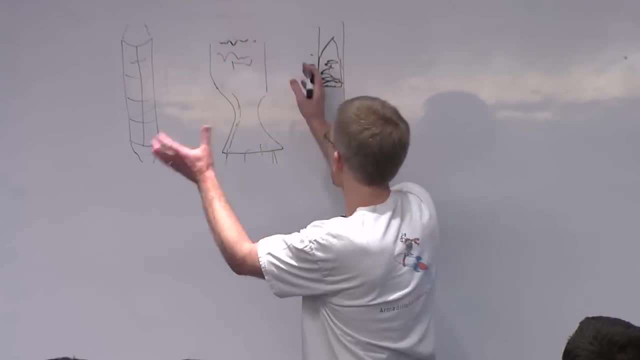 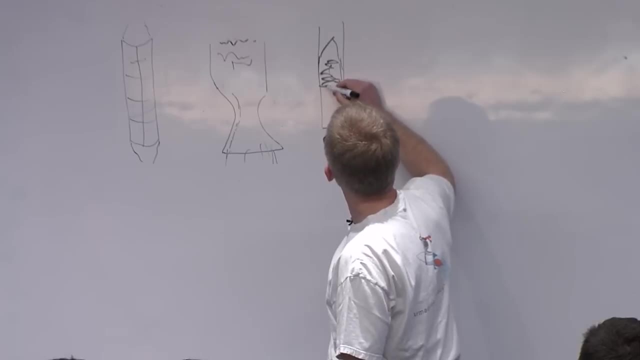 it turns into gas. kind of immediately it comes in, turns into gas here, the gas it combusts and accelerates, uh, with a gun, you wind up having something where it starts burning in different cases, but instead of burning at the end, like if you flipped a shell around and lit the end of it. 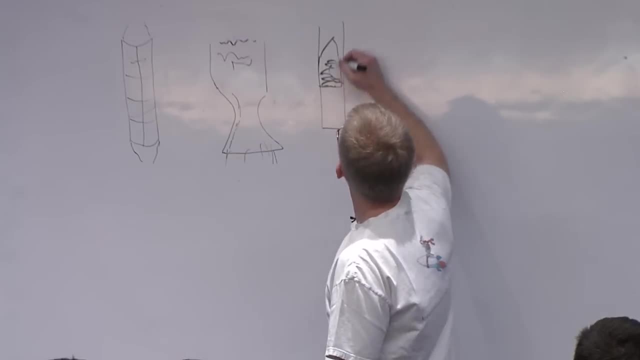 it would be a gas generator, rather like a rocket. but if you're actually pushing it out, the interesting thing is that the burning propellant here is not only pushing the payload, but it's pushing the other propellant. so the propellant gets pushed and then it starts burning and you 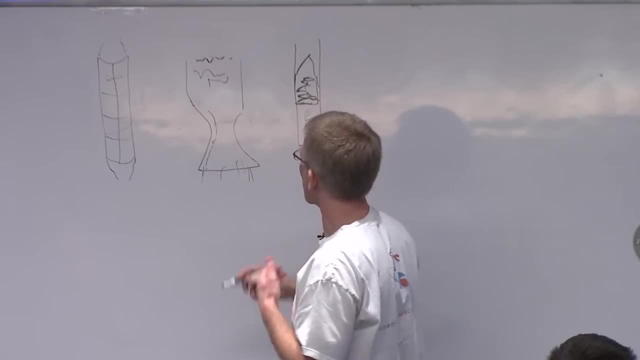 wind up being able to achieve, in some cases, a lot of the same thing, but you're actually pushing the, the propellant, out of the way, and then you're actually pushing the payload out of the way, and a higher velocity than you can with a traditional rocket. so i spend this time thinking about well. 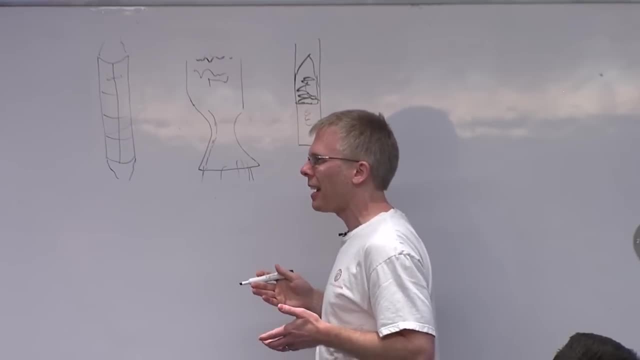 how can we make a rocket engine that might have gun barrel type dynamics? and i idly think about this now and i've got sort of a test plan in mind, but it'll be years before i wind up kind of getting around to spinning something up to to try this again i'm. but then there are ideas that are at. 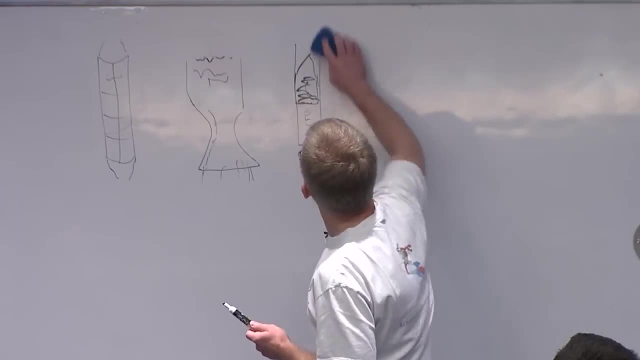 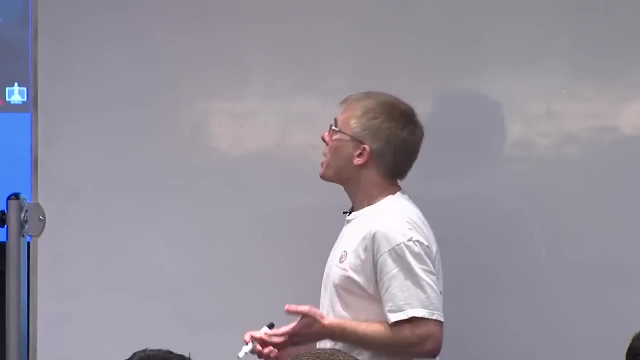 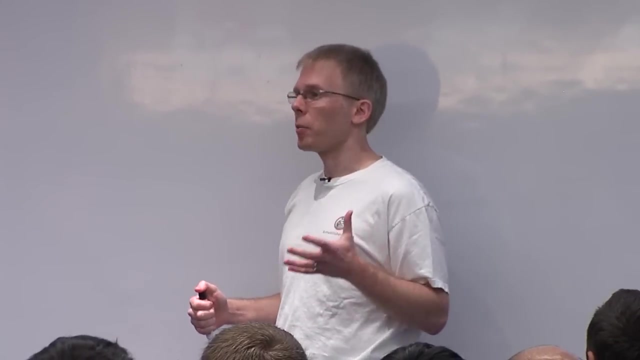 this middle ground where, uh, light fields are an interesting technology. this is again something from recent months, i so we have in virtual reality, we have panoramic videos, panoramic photos where you basically you can take. the two kinds that we have right now in production are monoscopic panoramic photos, which 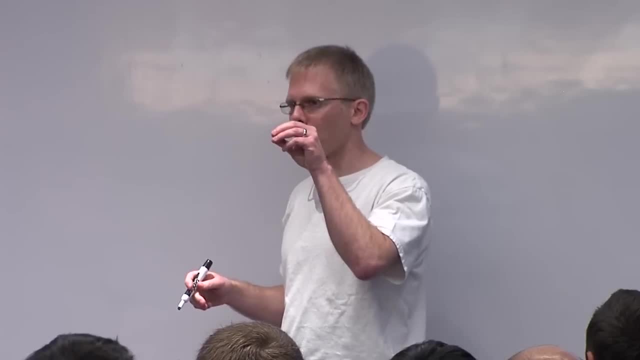 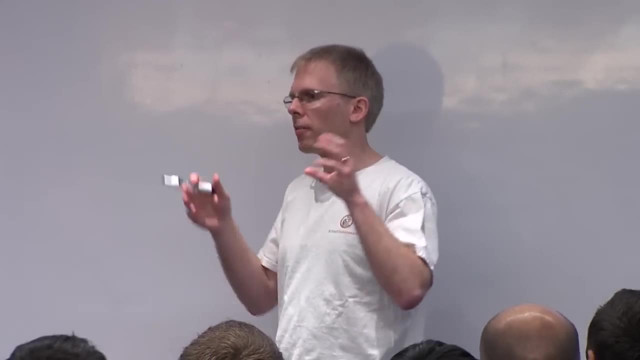 is where you sample the environment around you as if, theoretically, it was from a single point source. realistically, they're multiple lenses and they have to deal with stitching and warping things around, but it's a sampling of the environment from one source and those are, you know, easy to. 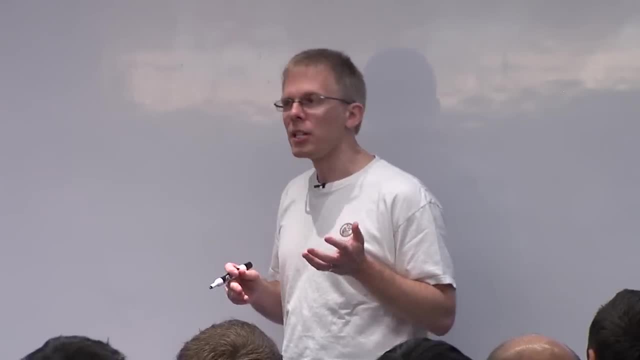 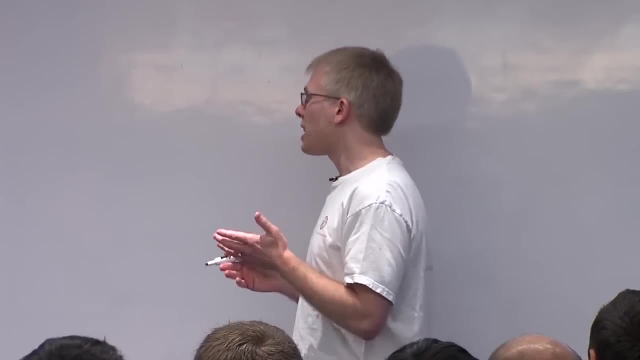 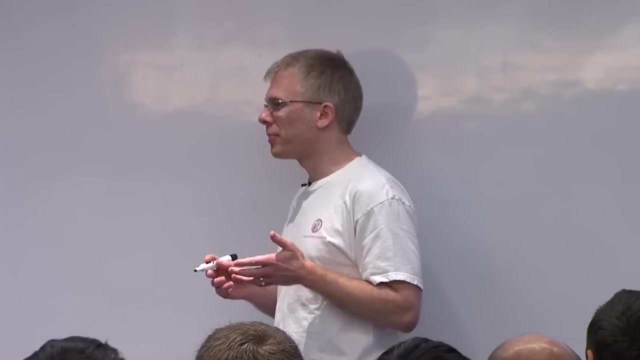 make fairly reliably, but you don't have any ability to have depth perception between your eyes or to kind of move around between it at all. i am. the next step up from that are the stereo panoramas- and i am- and videos, which are an enormous hack. i am. they're. 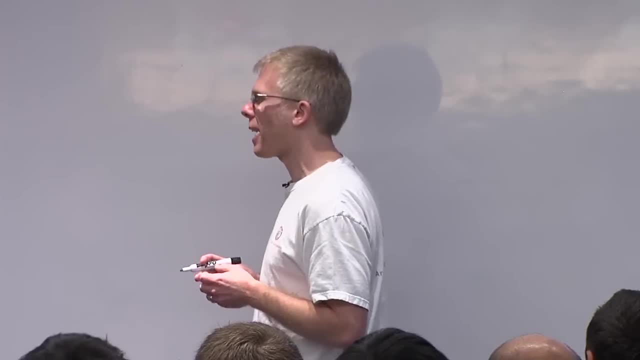 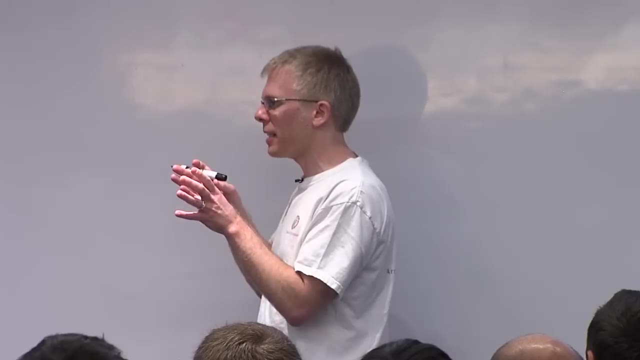 they deliver value for us right now, but it's really kind of a mess how they're, uh, how they're defined and how they're created. that takes lots more cameras that are somewhat offsets rather than all focusing into the center, and you stitch together something that looks kind of right for. 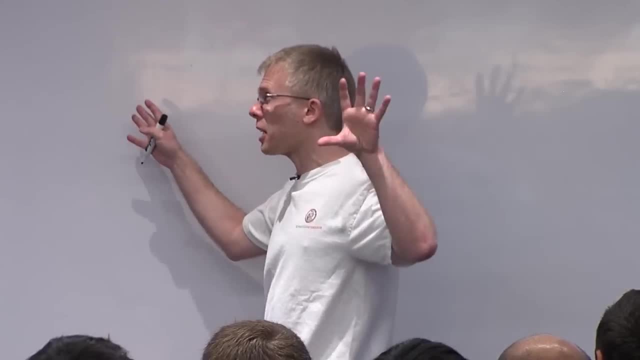 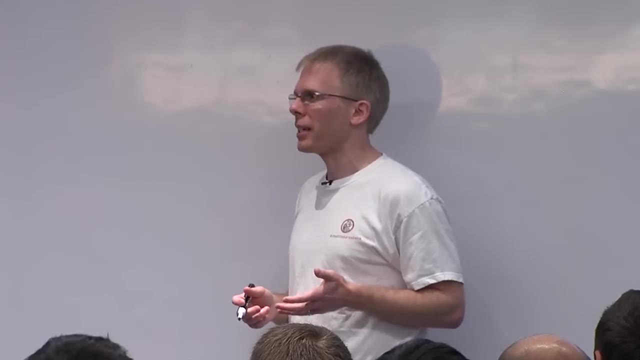 your two eyes and can deliver stereo when you're looking at things, but the things further away from the center aren't as right until you look over at them. it's an intermediate step, but where we all really want to be going is something close to light field technology and the idea behind. 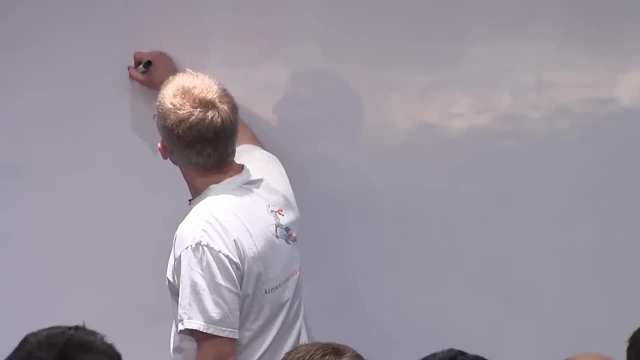 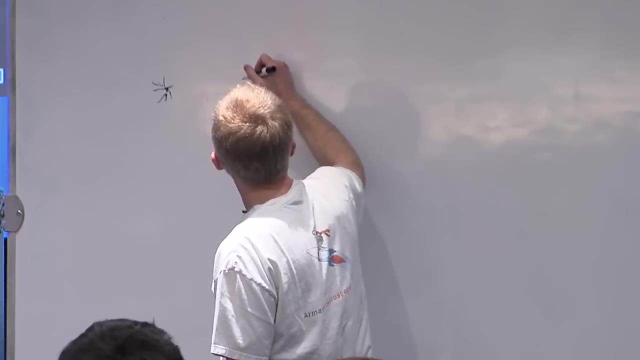 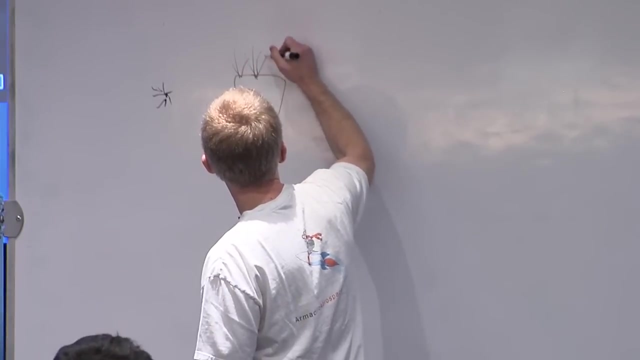 light fields is that, if you have- i like our normal systems here- you just have rays coming off from one point sampling an environment around you. if, instead, you had some bounding region around you, and from each of these regions you had light rays coming off in all the different directions? 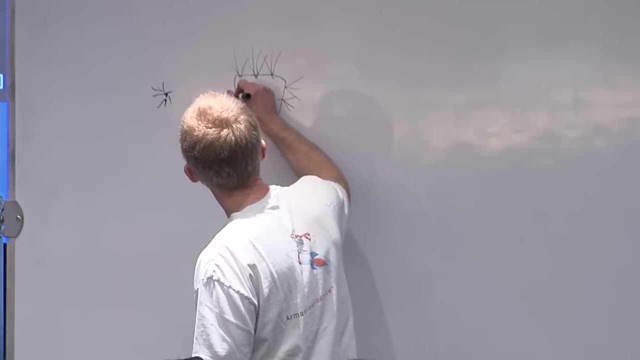 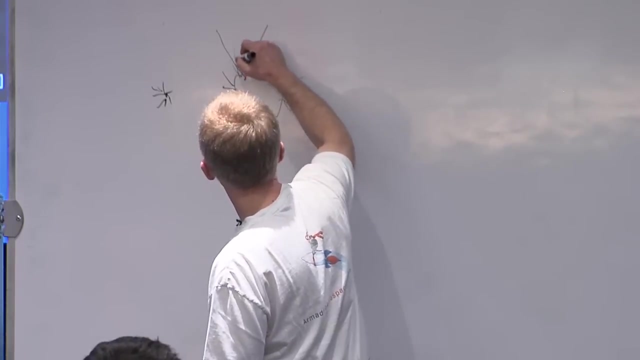 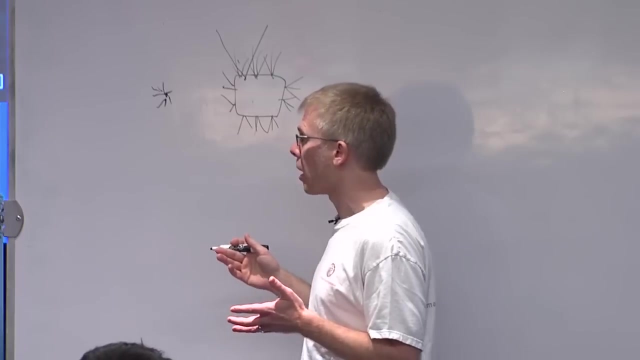 you could, in theory, then synthesize any view inside here, so you could say: well, i'm going to view up here, i want to make a view this way: i'll take some of the rays from here and some of the rays from here and this- this actually works- you can have if you have enough rays to be able to build the stuff from. 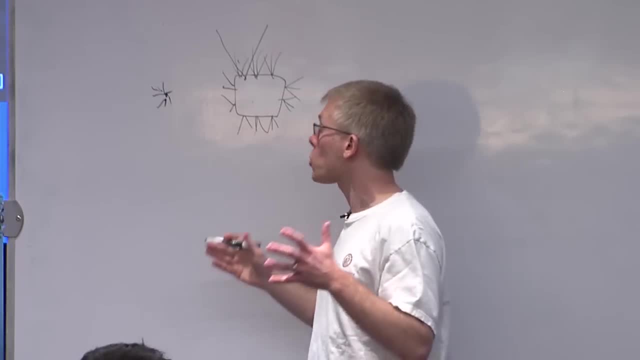 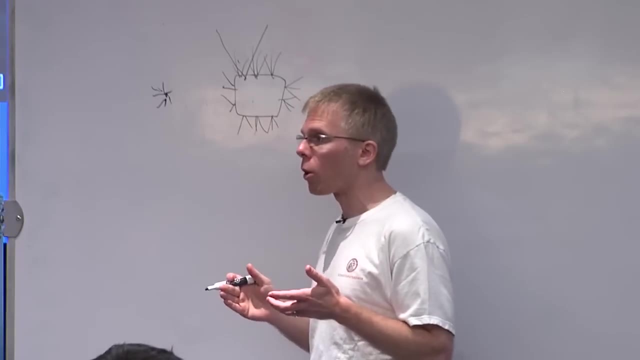 i am. you can synthesize moving around in an area and that's pretty magical. i think that this is what we want from our vr snapshots, where you know you can duck down, you can look around a corner, you can get all of this, but a raw light field takes an enormous 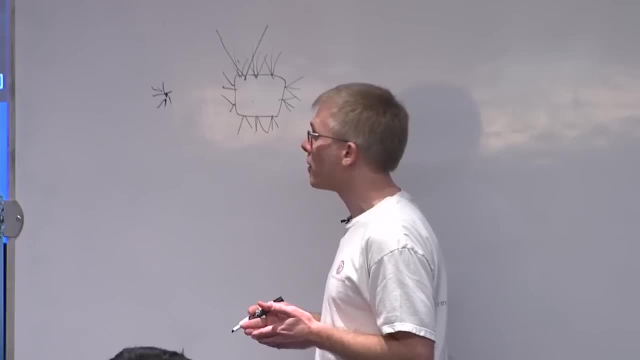 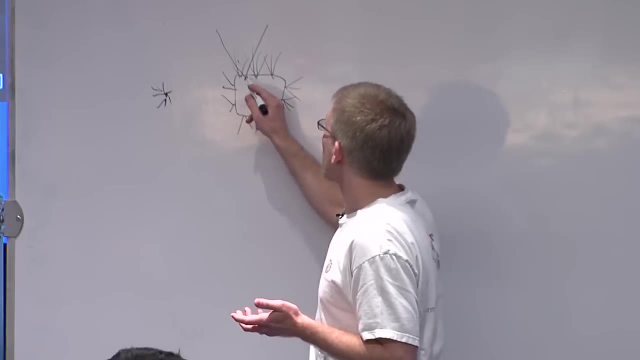 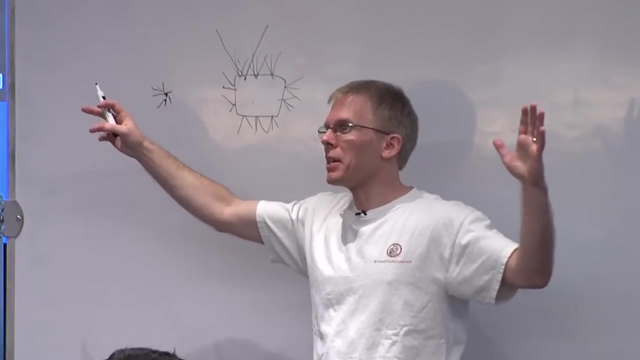 amount of data. you know it's gigs and gigs and gigs of of data and you're trading off resolution at all times because i, in the extreme case, you, want to have what winds up being one rendering sort of for every millimeter you can take the box that you want to view in. you want a one meter box. 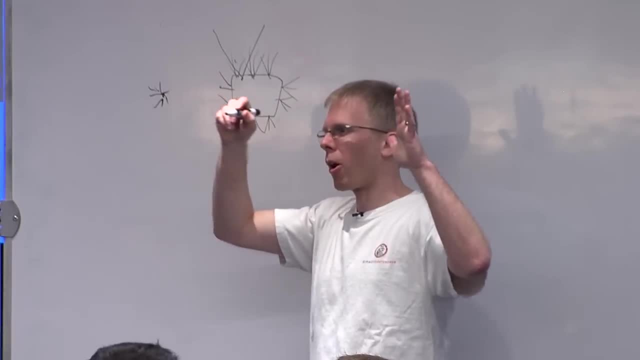 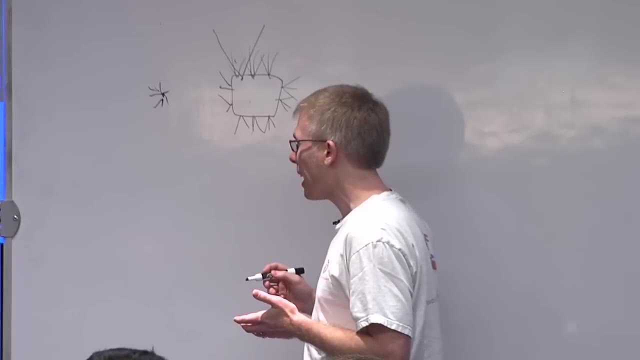 in most raw case. you want to step every millimeter or two across there and make these thousands and thousands of renders at the full resolution that you want to be using- and this is interesting for you know- for demos. there are some things that have been done in these relatively blurry images. 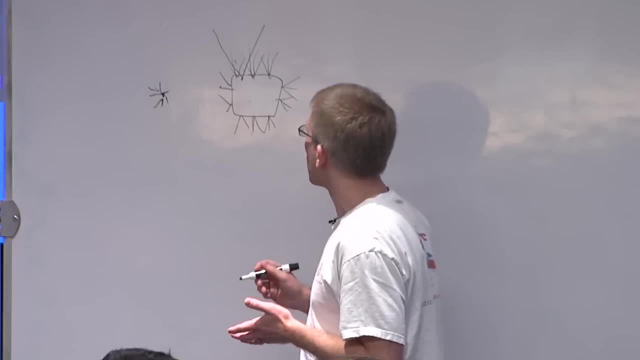 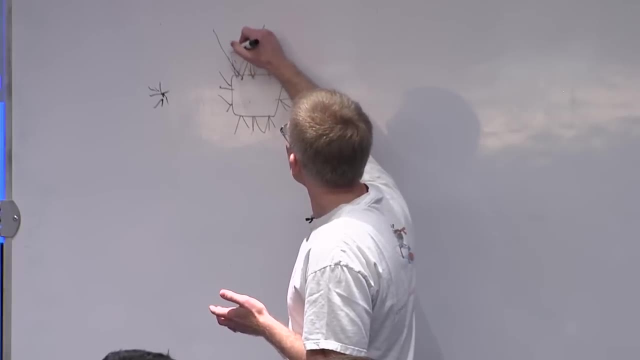 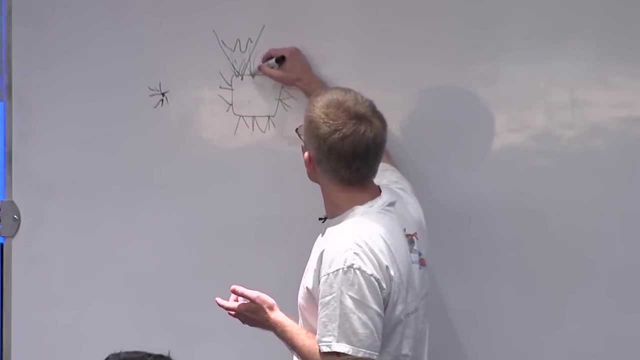 the step that people take generally to start making this more practical is to turn. it is to not just have rays with directions, but include depth. so you take an image here and you've got for it, but you've also got a depth field for it, and that lets you do much smarter things as 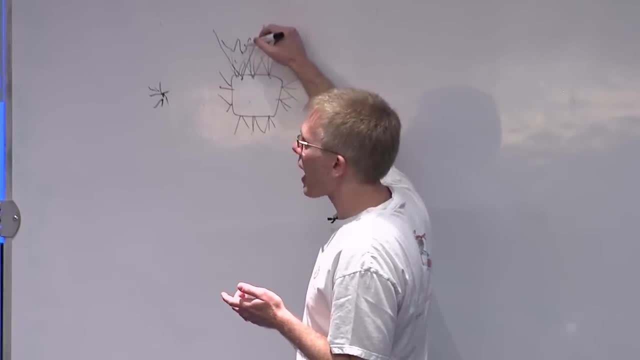 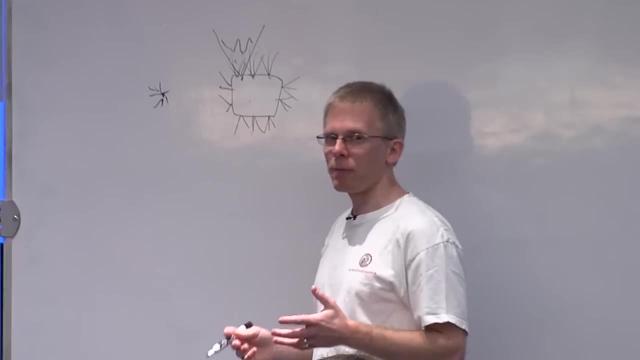 far as saying, well, i want a sample array here. i'm going to hit it at that depth and i can say, well, that's not exactly the one that i want. i probably want something over here. in the simplest case, if you were inside a beach ball, then you could have one panoramic photo with 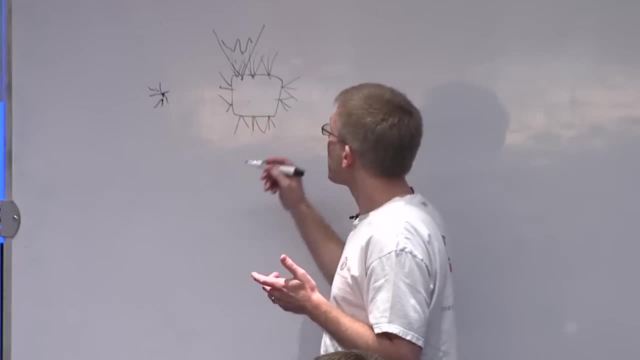 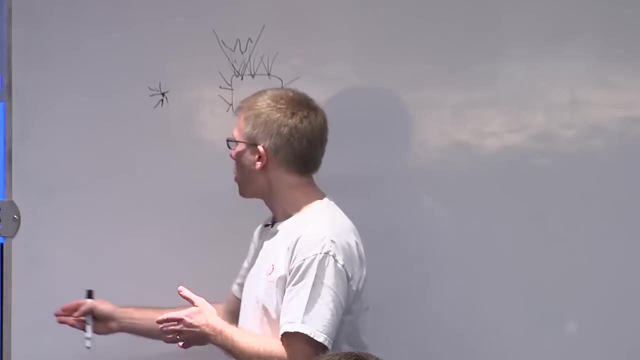 one depth and if it didn't have- i, if it didn't have surfaces that changed a lot in their view as you moved around. that would be all the information you needed, but in most cases we have a occluders. you know, if I'm from here, I need to be able to know that what's behind that occlusion. 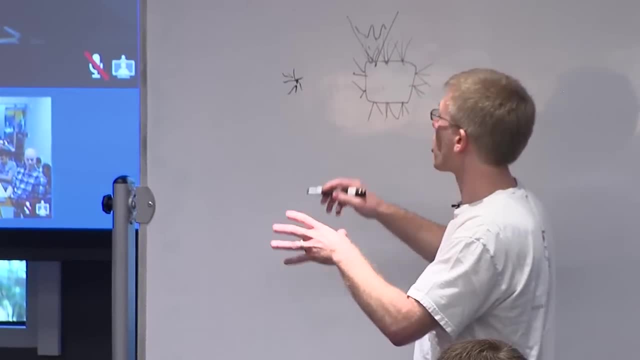 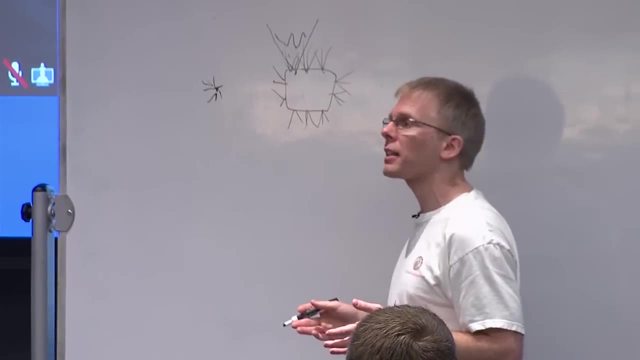 over there. So you have surfaces that you have views that are rendered in more from more points of view. The depths are tricky to get If it's synthetic, if it's just a ray traced image, then you've got the information immediately. But if it's a real world capture, then you start having. 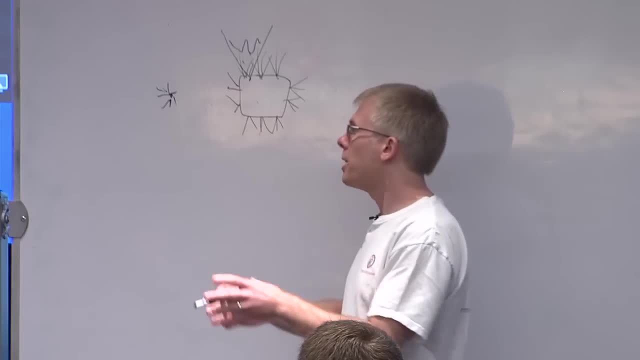 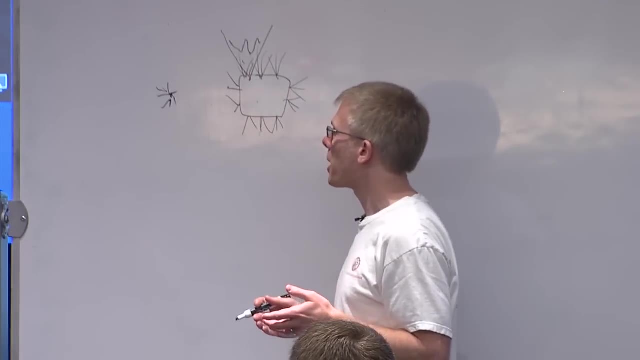 to apply these computer vision, computational photography things to take your multiple cameras, extract depths from them, add them to your structure here so that you can start re-rendering them, But they still take an enormous amount of data. You still wind up. if you want to have, 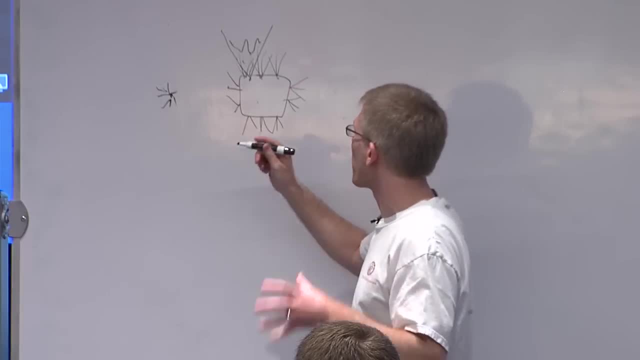 significant occlusion and like complex structure there you may need dozens of images at these full resolutions that you want that wind up being circles or hemicubes or something along all these things, to the point where it's still stressful on even modern high-end systems. 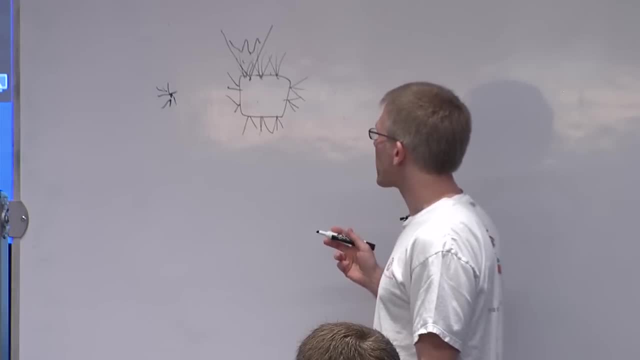 So the idea that you know I started thinking about on this, and this came as a result of, you know, getting Otoys demos, talking with them about their stuff and then you know, I toss the ideas back their way. see what everybody thinks about it. But the trick, when you do a projection from here, 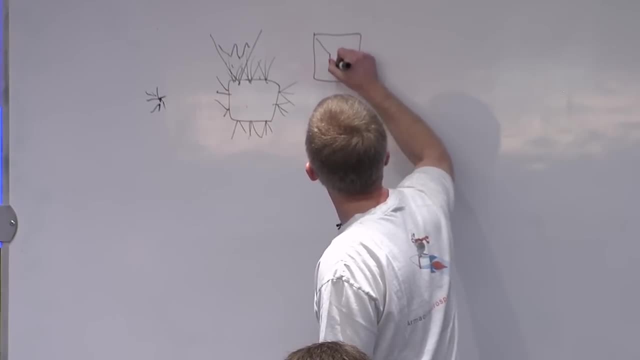 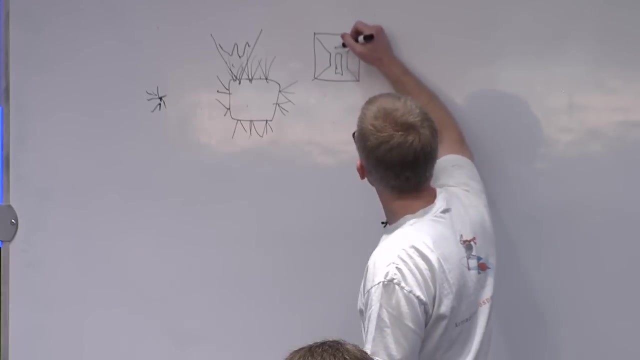 if you have an image and say it's, you've got a room and you've got some object inside there, so you've got big depth discontinuities here. When you wind up sampling a point on there from a ray, that's not exactly where this camera came from. 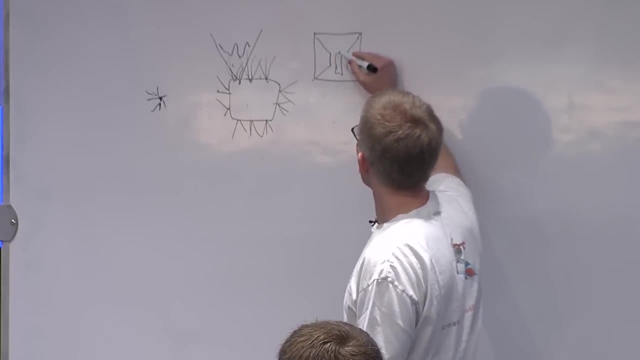 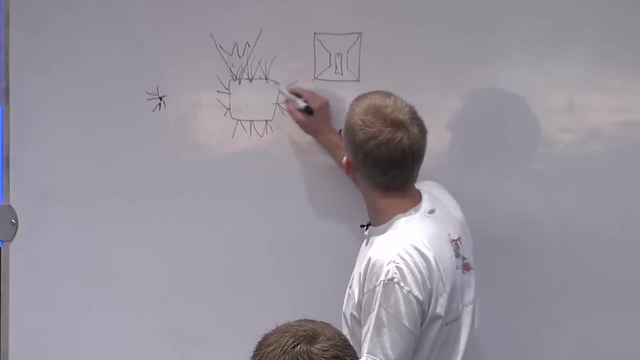 you have to wind up making an adjustment to the sample, that to the position where you get, Because you could say this would be exactly the right point if I was exactly at this camera point. If I'm offset from this, then the point's actually going to be over here a little bit. 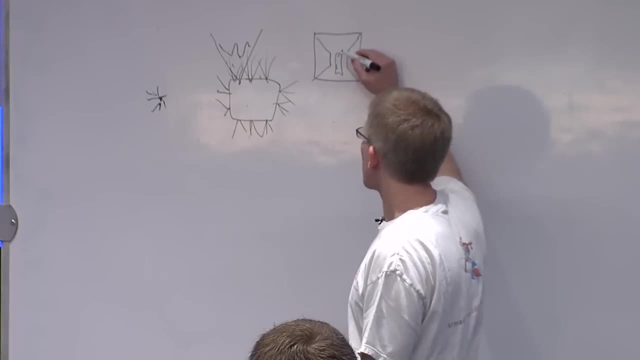 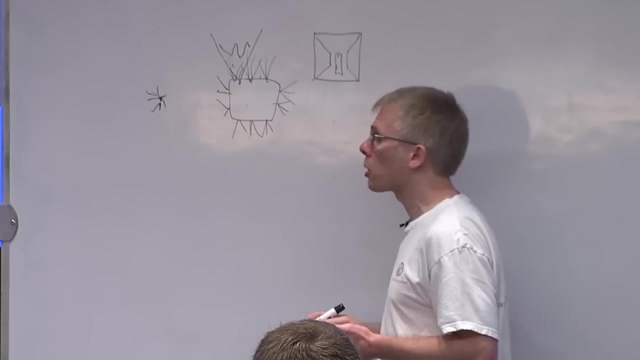 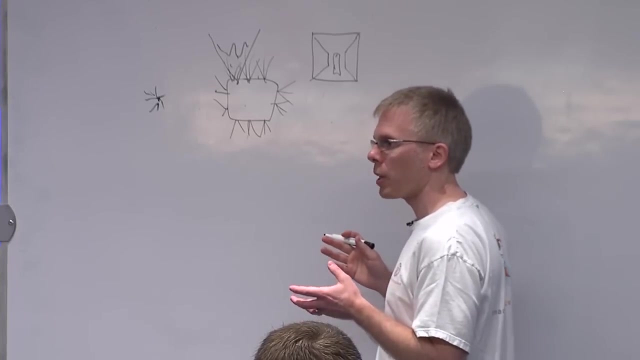 And you can tell, make a calculation based on the depth. Now, interestingly, this is exactly the same system for doing what we call depth correct- asynchronous or depth correct- time warping, where we have this system that we apply to the virtual reality renders. 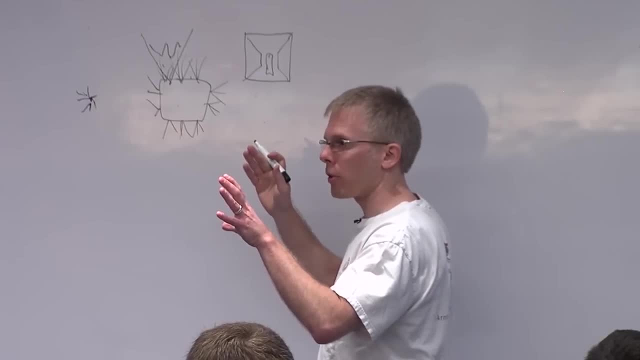 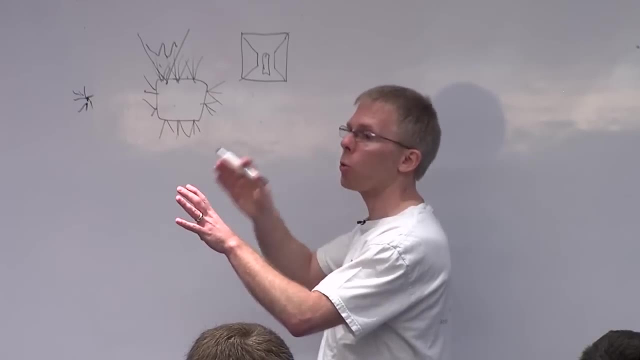 where you render your scene and then, at the very last moment before we show it on the screen, we sample the sensors again and we distort that scene in a way that lets it be closer to where you actually are, rather than where you were when you started on it. 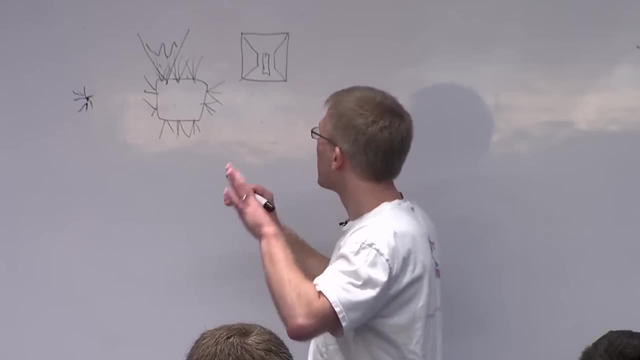 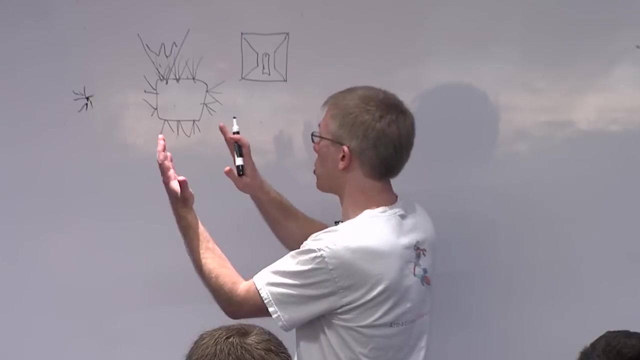 Normally we only do this for attitude, which is a simple projection, but if you have all the depth, you can do this reprojection so that even if you're moving just side to side, you can have it, do some of this stuff. 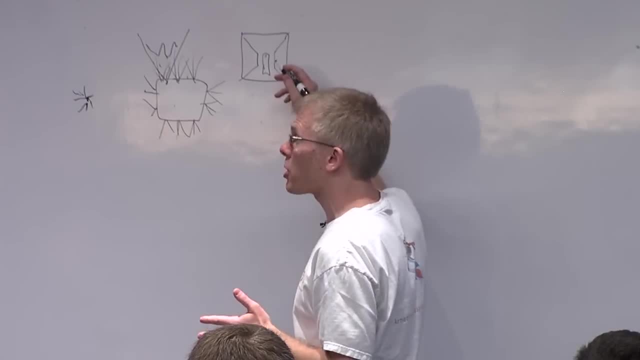 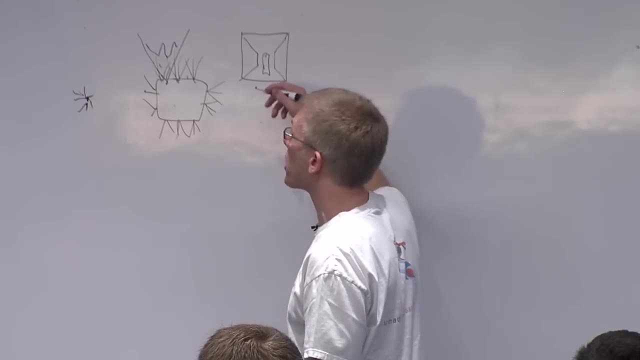 You'll wind up with problems at the silhouette edges, but it's interesting that this is a technique that I had been working on years ago just for the time warp reprojection, but it's also directly applicable for all of these light fields. So the one of the problems with that is that if you start it, you hit this point on the depth. 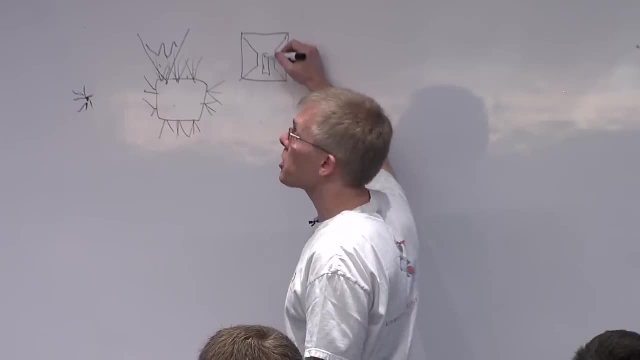 if it actually says: well, you should be over here. if that's on the same surface, then that's really a good point, It's a good approximation. but if it's moved off of that surface and it's on something different, then that's actually going to be pretty wrong. 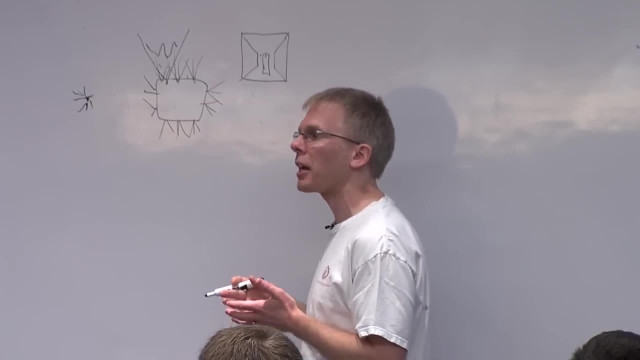 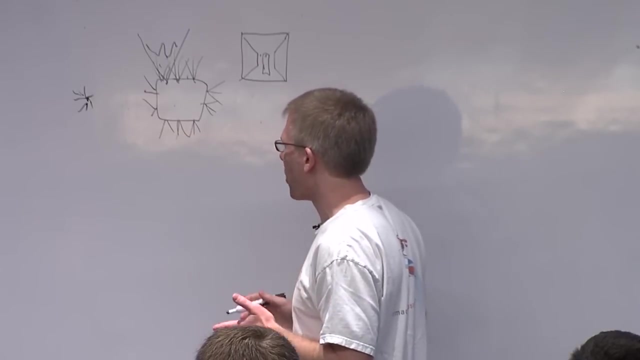 And if you look closely at a lot of the- if you get a chance to look at light field renderings, you'll often see this on cases where I guess technically we should call these luma graphs, if they've got depth, depth, augmented information with them. 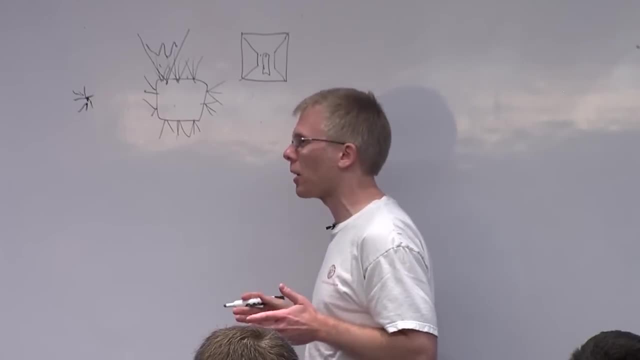 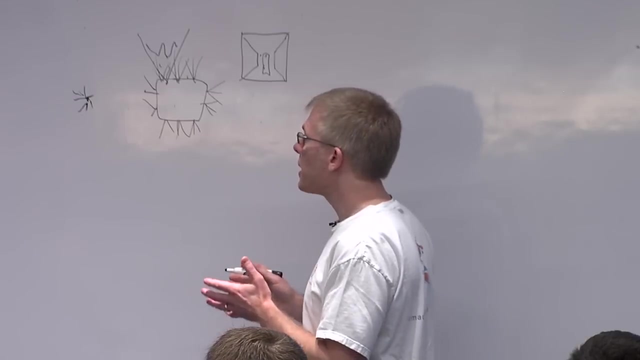 but there's a lot of confusion about terminology and everybody's making a light field camera now if they've got more than one lens. just that's the buzzword to put it. But you'll see that in general, these things look remarkably good when you have surfaces without a lot of occlusions. 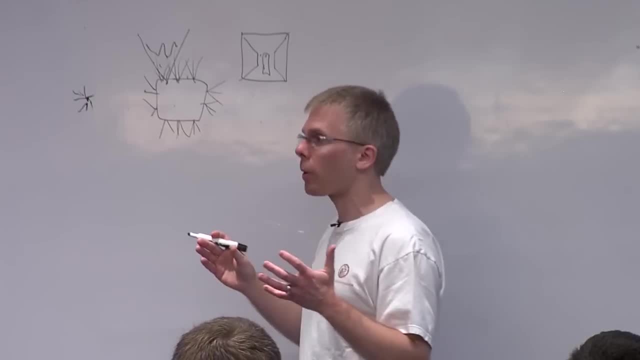 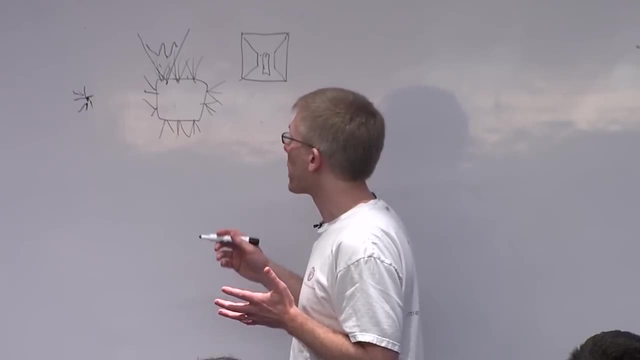 You can look at it and it can be great. You can duck down, move around, look at it from different angles and see changes in specular highlights and everything. but there are usually problems there at the edges of things, like if we had a light field here as I'm looking around, that occluder there. 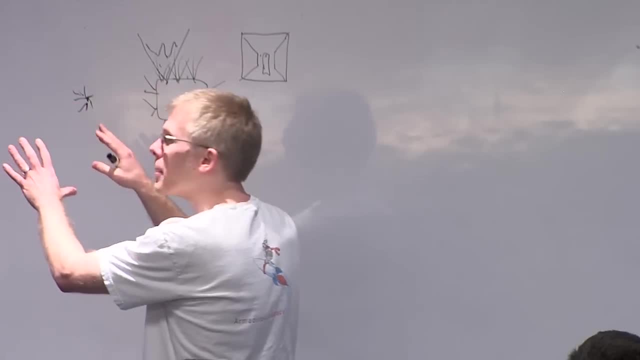 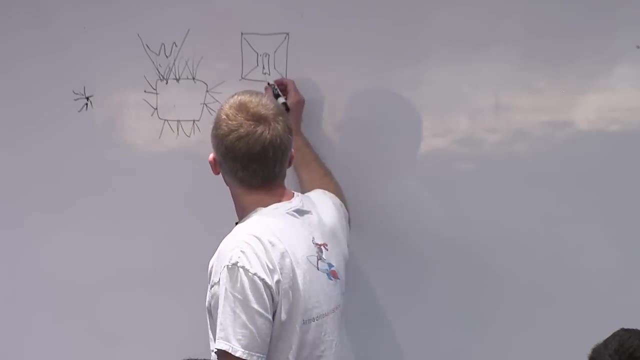 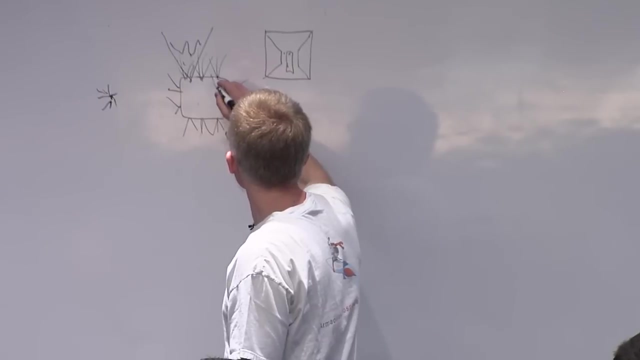 there would be issues where you would see ghosts and double images and some of these other artifacts for it. So my thinking is- my thinking for this is that if you just sample from, you've got a grid of light field, images, of images captures here. 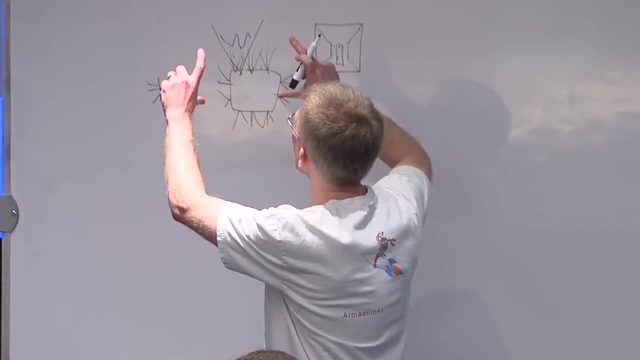 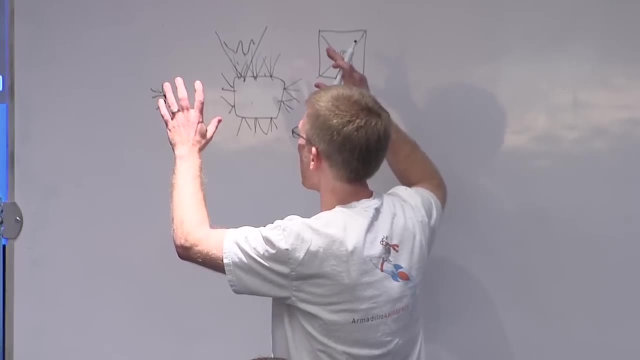 and you can sample between the four of them. there you've got the four closest images and then you can find the four closest rays on each of those and you can do this just straight, filtering through all of those, but you wind up with ghost images. 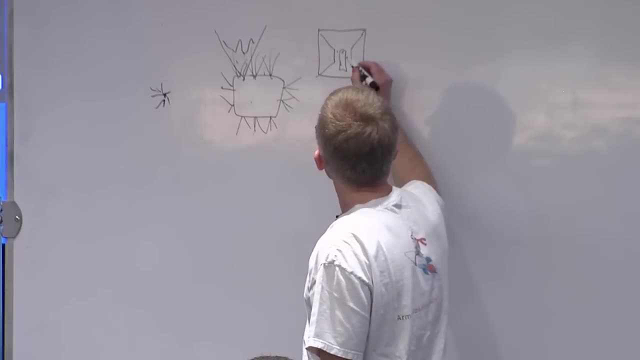 My first thought on this was that, well, we can actually tell from the initial point and then the final point- there we've got a depth. from that We can tell whether that was close or wildly off from what we were initially looking for. 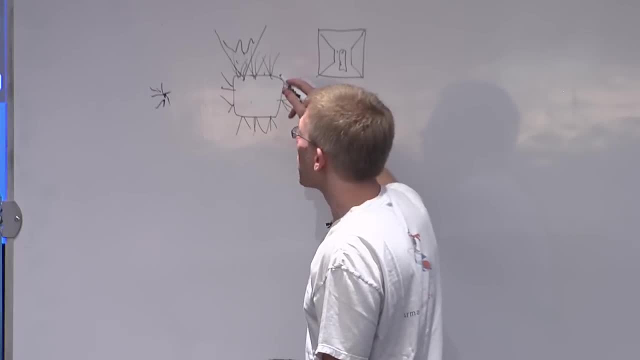 So instead of just blindly blending all of those samples back together, we should go ahead and look at them and throw out the ones that have clearly gone to another surface, So you wind up just sampling from the ones that are the closest there to get rid of most of the ghosting. 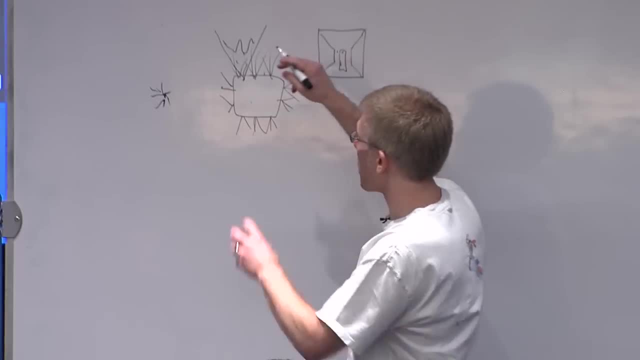 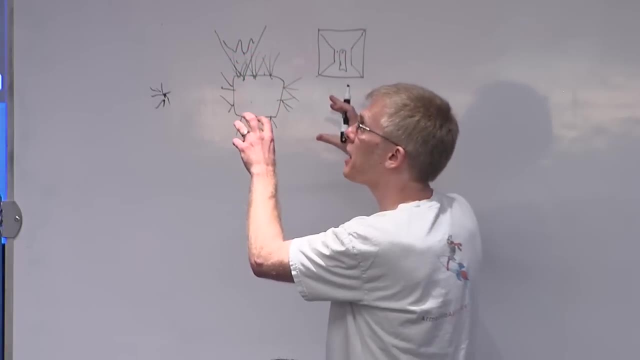 But then, as I started thinking about the samples that we're looking at here, the ones that we're getting, you're in between four samples there. you've got four samples that the ray's going to be between. There's going to be 16 samples at your disposal. 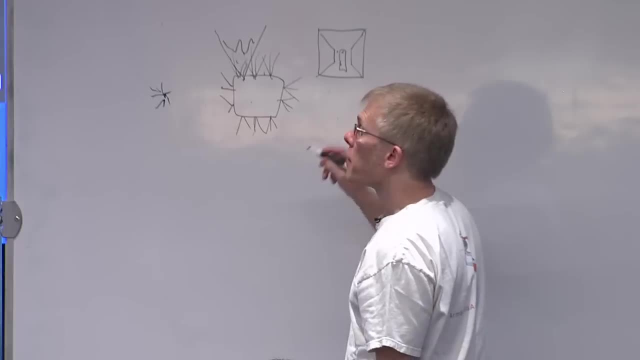 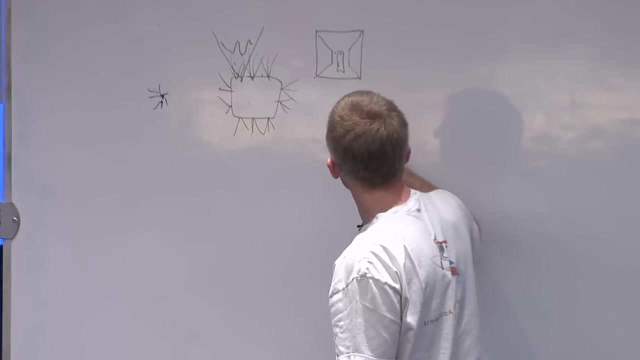 but what you really want to do is find three of them that bound the sample that you want, where you want to be able to say that I have a sample from here, a sample from here, a sample from here, and then here's where I am. 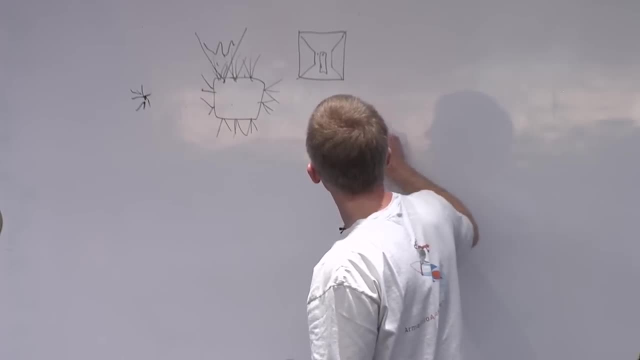 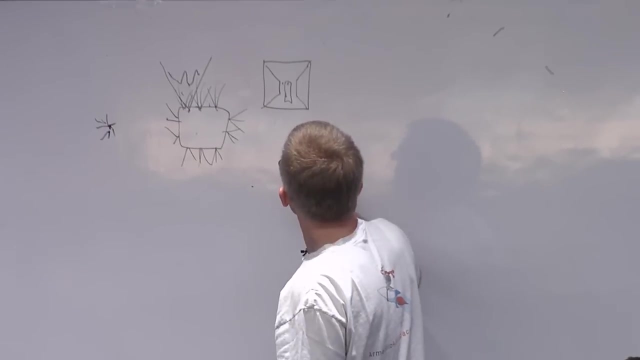 and just do the interpolation between those, because you may have other samples that are out here and then some of them that are way over here because they actually went to the wrong surface. If you can identify the samples there, there's an interesting idea that occurred to me. 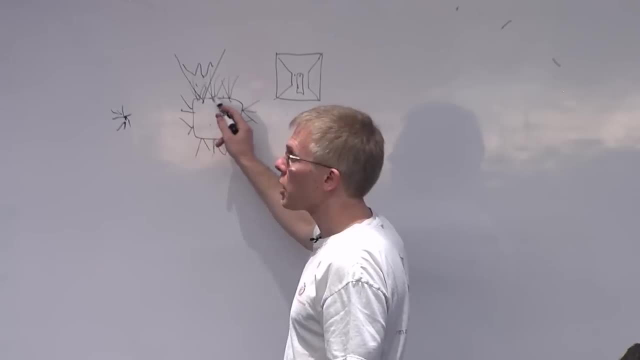 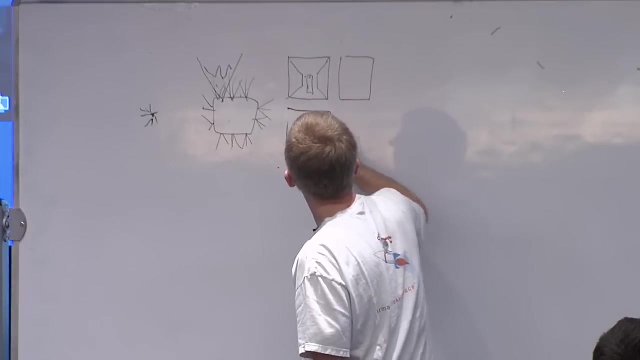 that we may be able to save three-quarters of our pixel samples here by saying that we have the four images that are the nearest ones for what we're doing here. They're all slightly different, So similar images, They're very close and you look at that and say: 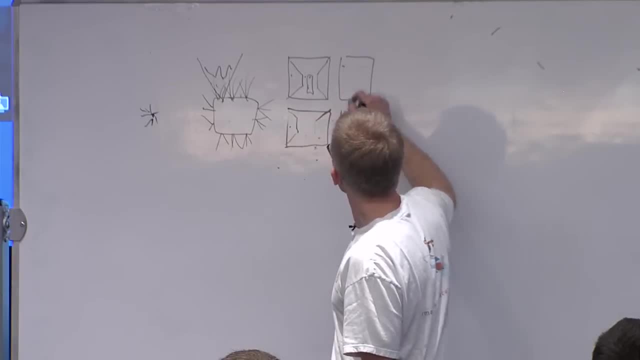 there's an enormous amount of waste where it looks like the same wall on each of these. It is slightly different. They're slightly different positions, so they have slightly different rendering artifacts for them, but there's a lot of commonality. Now these compress quite well. 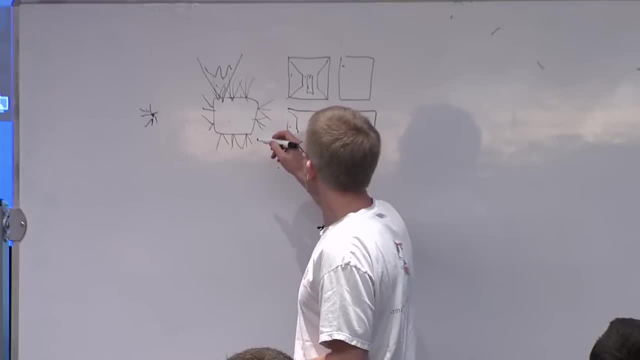 What you wind up doing if you want to compress these for transport, is you wind up saying you have 64 images or something on here? You just wind a spiral out, video encode it, because it does very much look like these linear moves moving around. 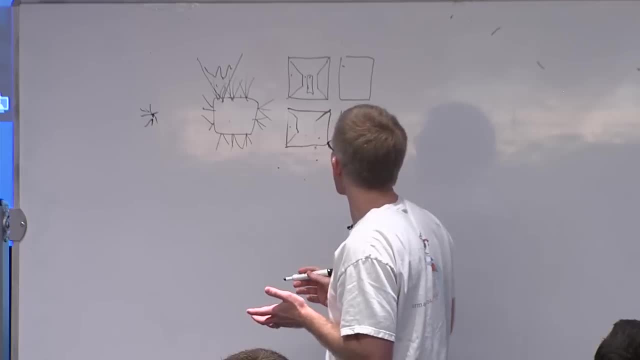 and it encodes quite well, but you need them all decompressed to actually render with them. So the idea that I'm excited about- that I have not yet proven or disproven here- is that if, instead of making these from exactly the same central render points, 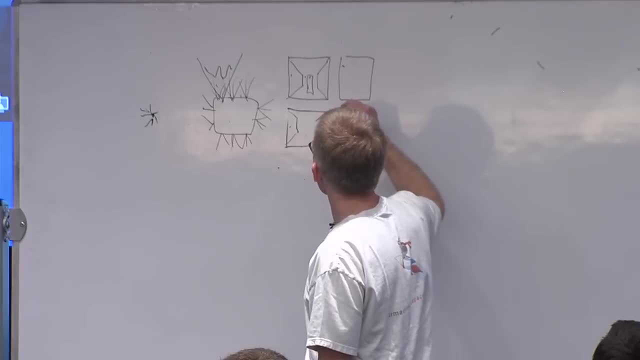 if we offset them by a pixel each way so that you have a dithered interleave of the samples. so if you had a sample from like this, one might have samples from those angles and then the next one over as an exaggerated scale. 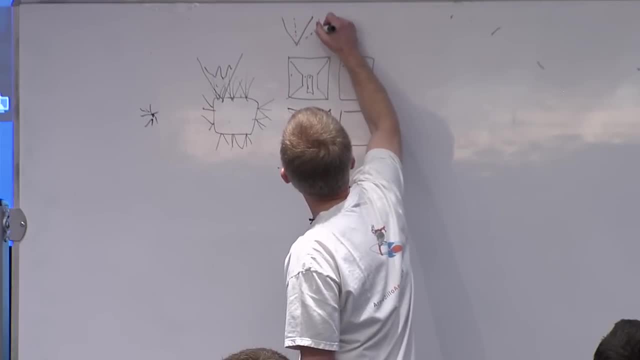 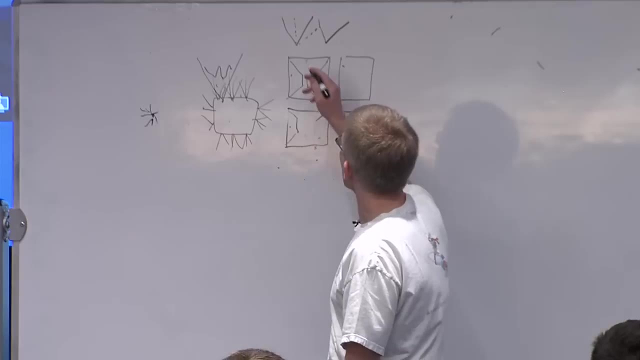 might have samples from that angle, so that they are sampling different sets of angles. Now that would mean that the image there would be aliased. You couldn't sample it directly because it's stepping over information that you would need for the direct referencing. 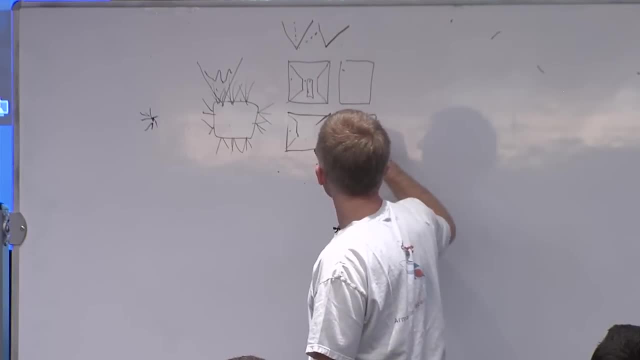 but if you gather the potentially 16 samples- and it may only need to be done with potentially four samples even you gather the samples from those different ways- throw out the ones that have these kind of off-kilter depth values and then you find which ones bound the surface there. 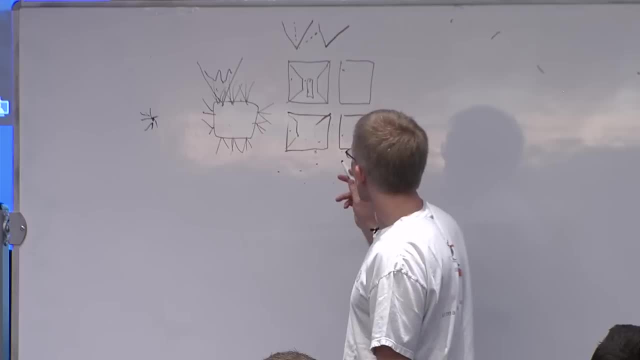 I think that that can be done where you can get a 4x space savings, And again, 4x is actually usually the number where things start mattering. I mentioned that on the resolution side of things and I used to say that about a lot of computer speed stuff. 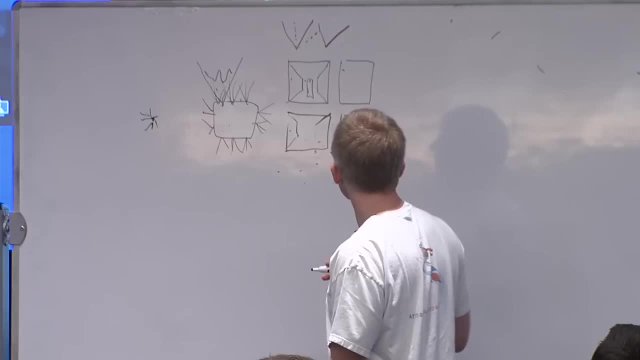 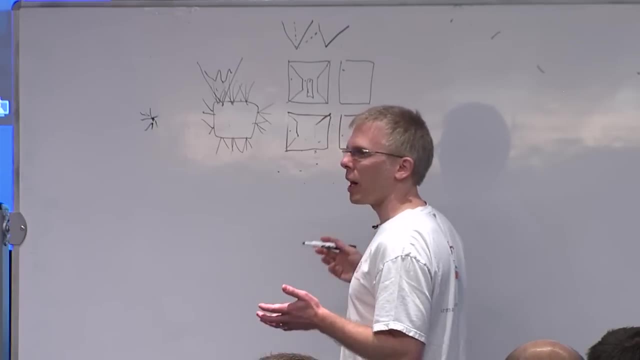 where 4x is, when you know your computer got a whole lot faster. That would be a great way to do that. It's a great thing, and I need to find the time to go and test this. It's great when you wind up having more ideas than you get an opportunity to explore. 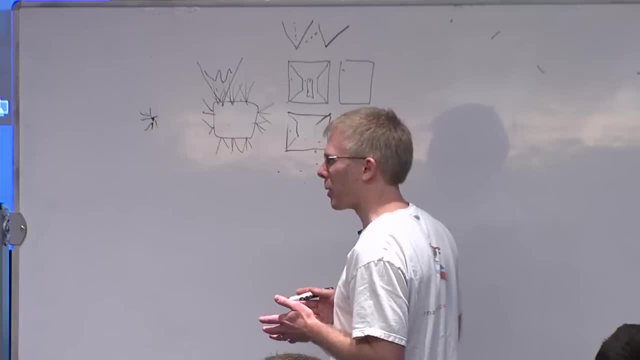 So of course I send some of these things over to Otoy and I hope they get to go explore them, because I'm happy if it just works out And it's possible that this could even be extended more ways where, if you can tile by or if you can interleave on a 2x2 factor. 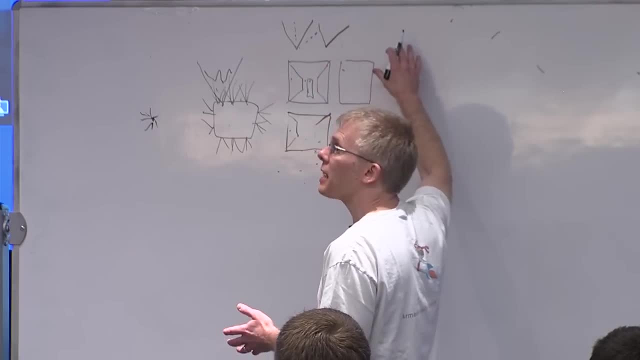 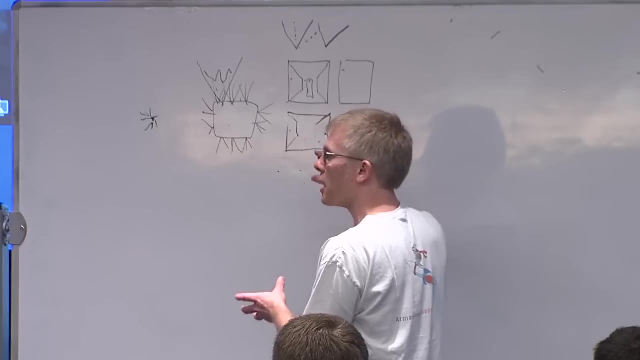 maybe you can interleave on a 3x or a 4x4 factor. Maybe there's a 16x factor that you could get. That would mean more sampling. You could trade a more expensive fragment shader to go and gather all of these. 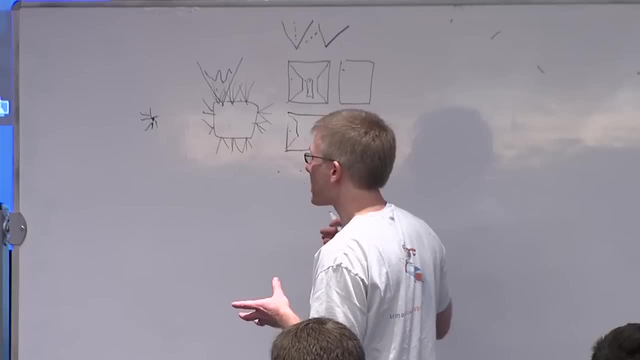 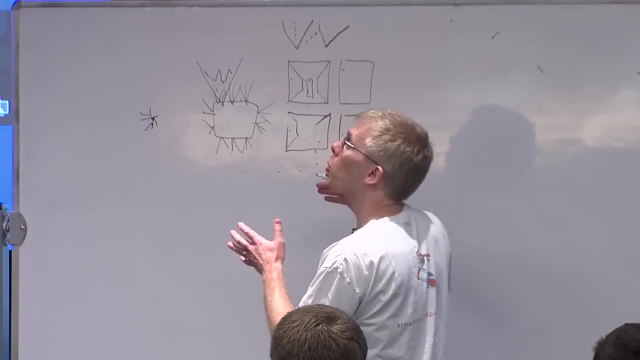 and discard them and do those tests there. But it's a potentially larger impact there. If you go too far, you wind up getting to the point where some of the changes in visual effect from different angles that you want to get, from things like light fields- 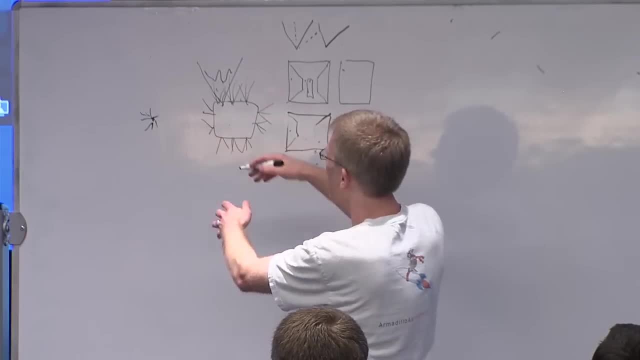 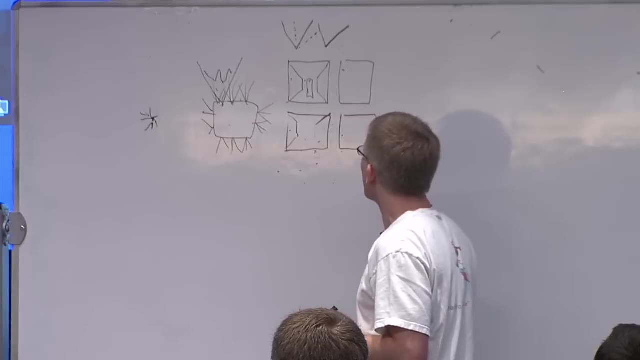 you might not get because you would have something all the way over here contributing samples that go over to it, But I'm suspecting it may be good for at least this kind of factor of 4,, which is a good thing, Which is exciting. 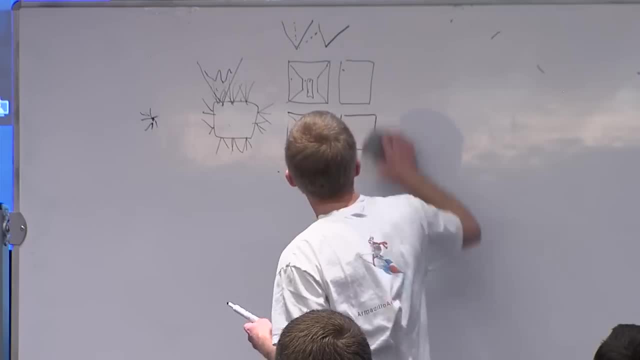 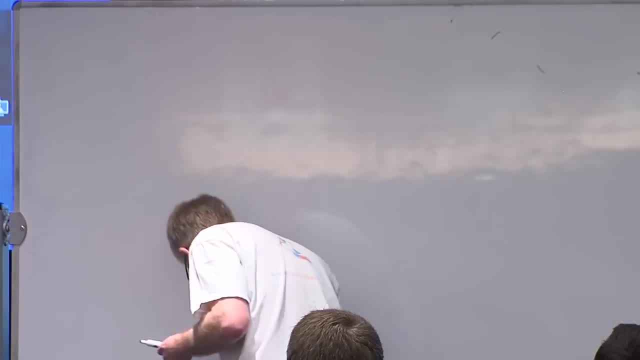 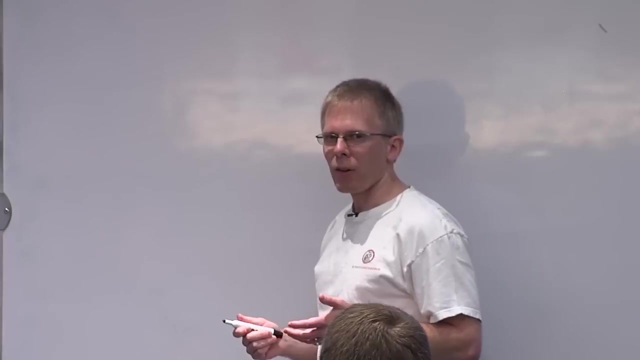 And maybe it's good for even more. Another path of an idea in the last month that is actually working out extremely well is again on the Minecraft project. One of the things that we've learned in virtual reality is that the simulator sickness that most people associate with VR 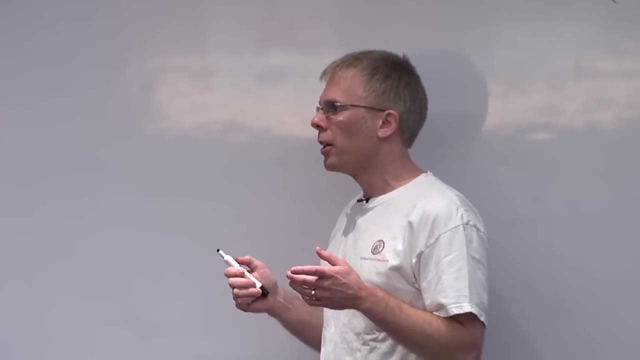 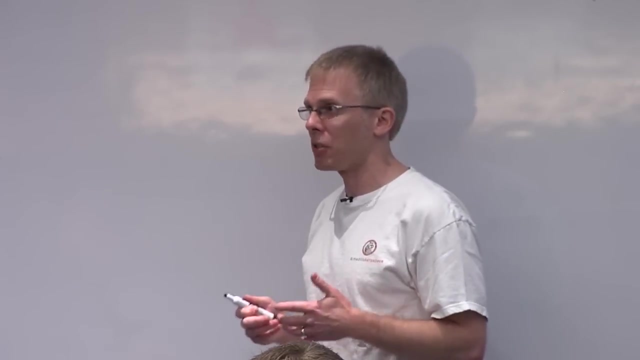 there's a lot of different types of discomfort that are issues in VR. There's eye strain from focus, eye strain from vergence mismatch, But what most people associate it with is the kind of sick-to-your-stomach, queasy feeling of eye simulator sickness. 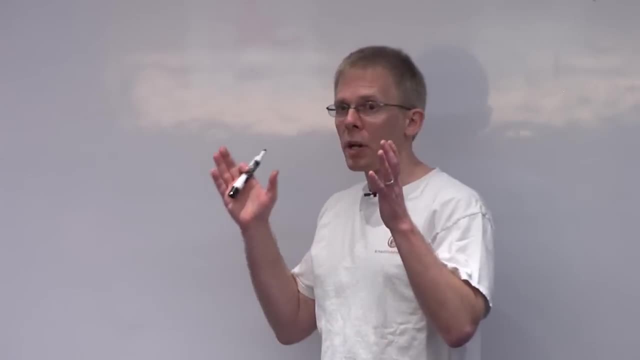 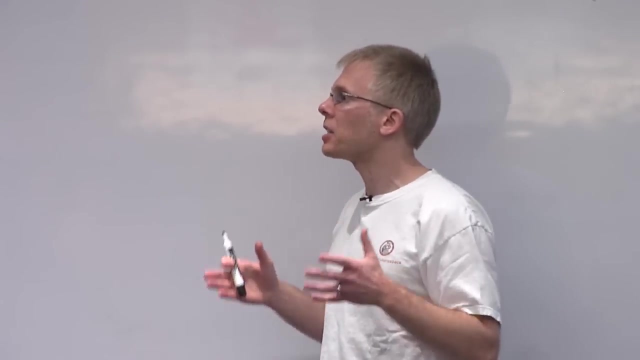 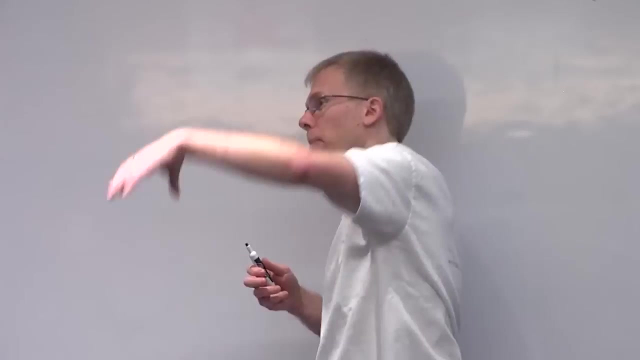 which is mostly a matter of when your brain is seeing an image set that it accepts well enough and it's accelerating in some way that's different from what your vestibular system is telling you. that mismatch causes the discomfort. So if you've got something curving up on a roller coaster in virtual reality, 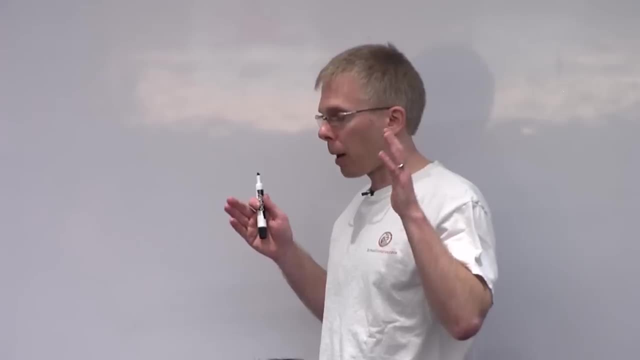 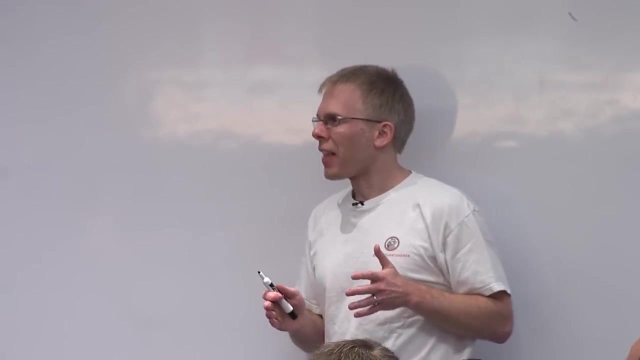 but your body is staying still. your body is saying it's like my eyes and my vestibular system are not matching. You probably ate poison You should throw up. And that's the kind of general theory behind a lot of this. 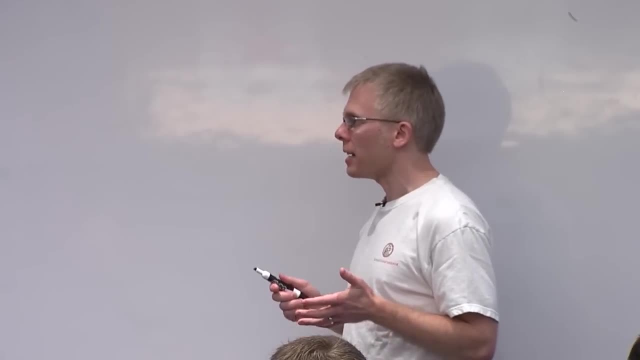 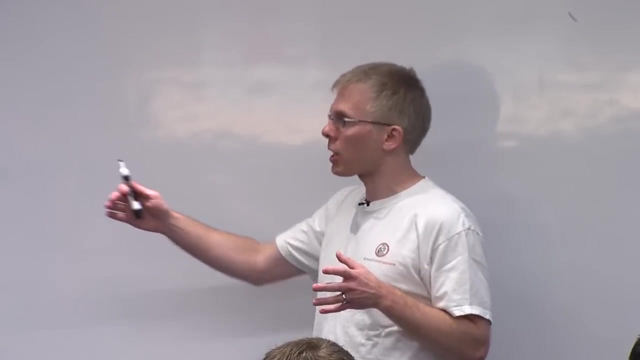 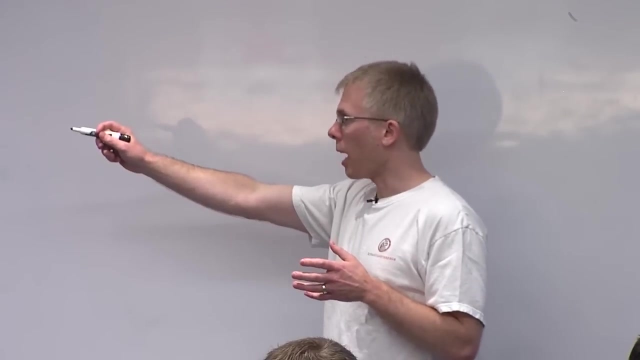 So in VR the thing to avoid is accelerations. If you assume that your user is seated or standing roughly in place, any time you're accelerating, that's when the body is going to complain. Linear motions are generally not a problem. You can be kind of moving along, rocketing along. 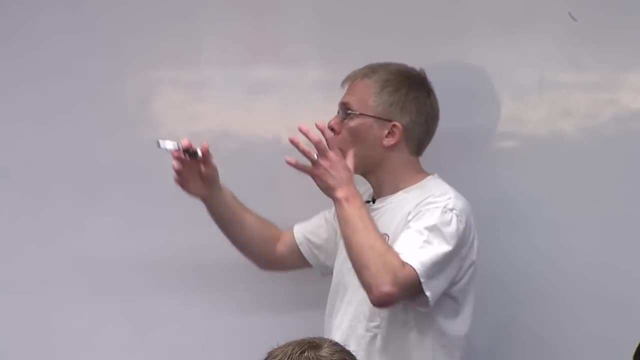 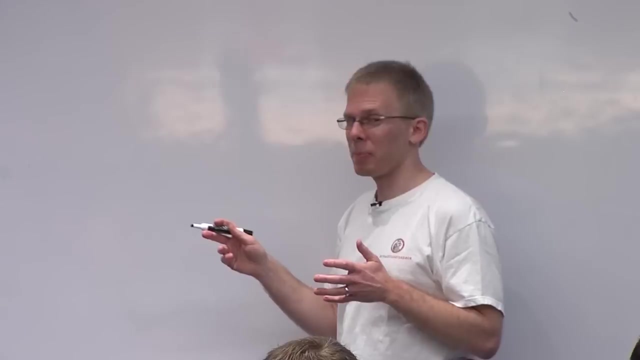 even at speed in a straight direction, And if there's not too much stuff like cluttering up your view, that's usually not a problem. But if you slowly accelerate up to a specific point, like certain space game launchers, that kind of rocket you down an area. 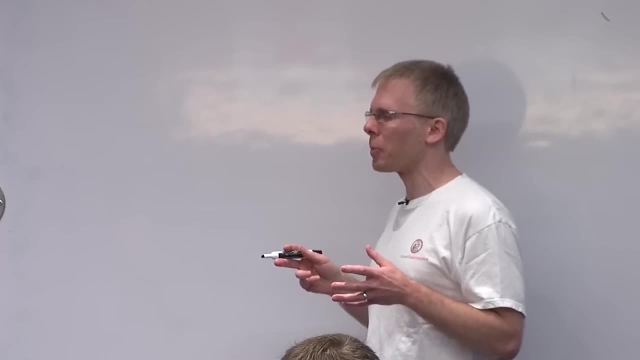 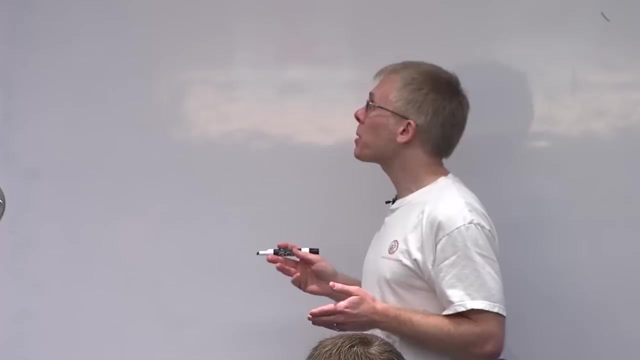 that's particularly bad news, And some people are just like I close my eyes for that point because it's going to make you uncomfortable. Now there's an interesting aspect about this where if you make changes in discrete enough changes that it just chops, then it winds up not being uncomfortable. 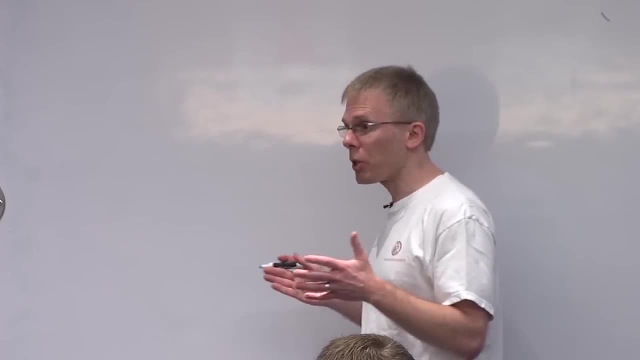 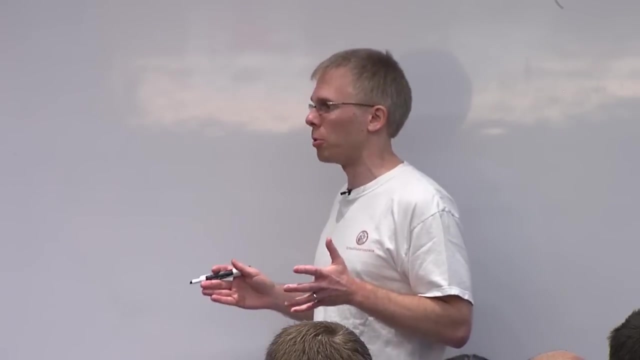 So one of the obvious things that especially affects the PC side of virtual reality is when you're turning. that's an angular acceleration. You may be staying motionless, but the angular acceleration is really bad news And I am far less prone to simulator sickness than most people. 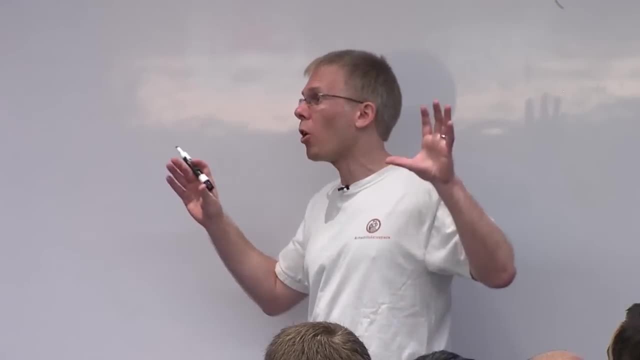 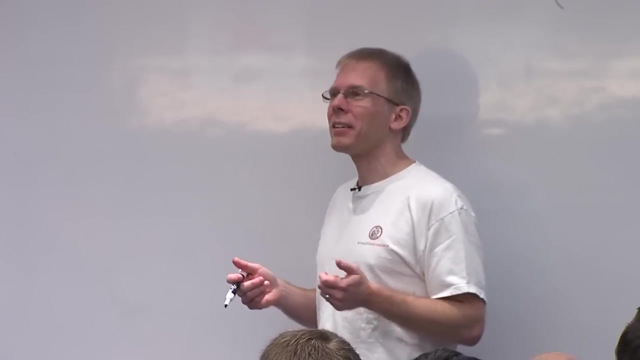 And my theory about that is because I wear multifocal glasses, the world is always swimming a little bit, so it's trained me to be better at virtual reality. But even there, just sitting there and spinning, you know, stick turning, I call it. 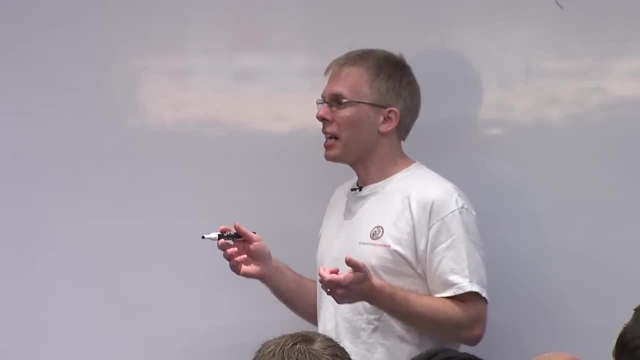 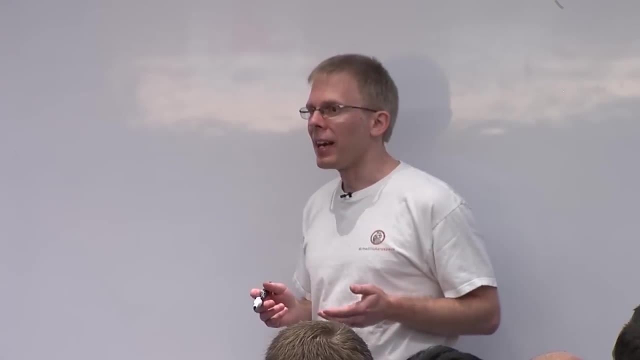 where you're yawing, based on a continuous input, is pretty bad and you don't want to do that for very long And some people will be almost instantly sick from it. But it's been found that if you break that up and you only do it at, say, 10 hertz- 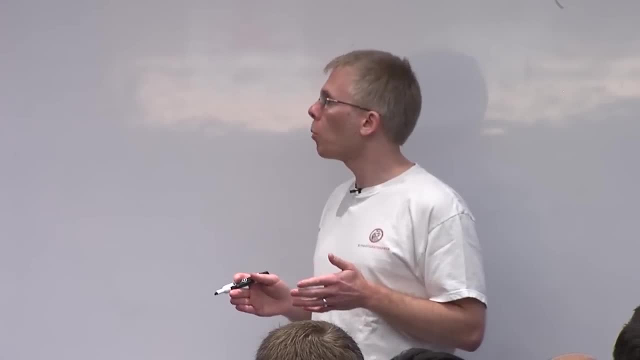 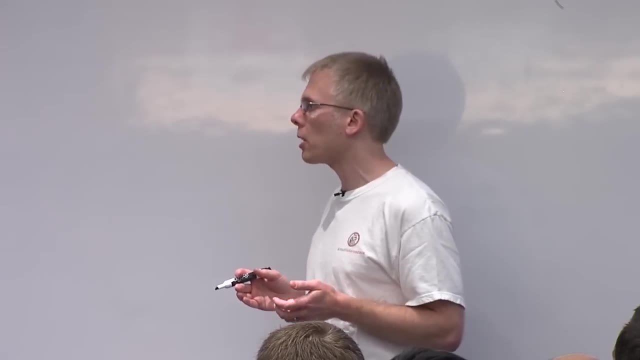 where it's no longer smooth. so it's this choppy stutter turn. it winds up not being uncomfortable. Now it doesn't look great because it's stuttering that way, but people can functionally play through things and wind up not being sick. 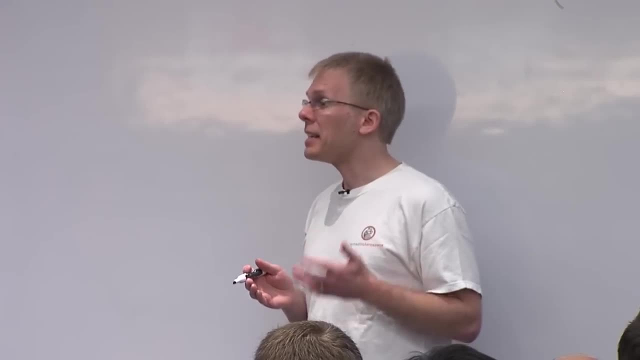 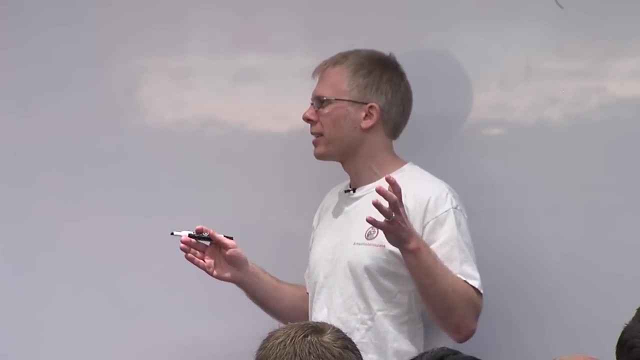 Now there's an interesting trade-off there, because it definitely gets you out of that sense of your brain's like I'm buying this, this is great, I'm in this virtual reality, but stutter, stutter, stutter. you know, that's OK. 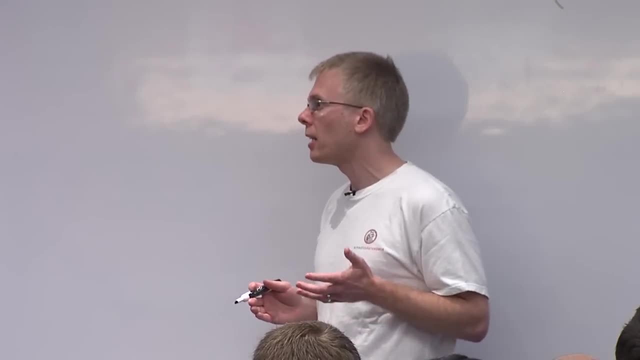 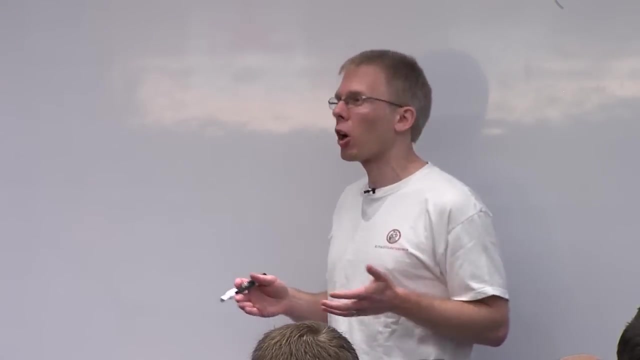 I didn't quite buy that. but at least I'm not sick. But it's a trade-off that you can make. But it's always better to try to remove the kind of accelerations as much as possible. I mean, I advocate for like Gear VR playing in a swivel chair. 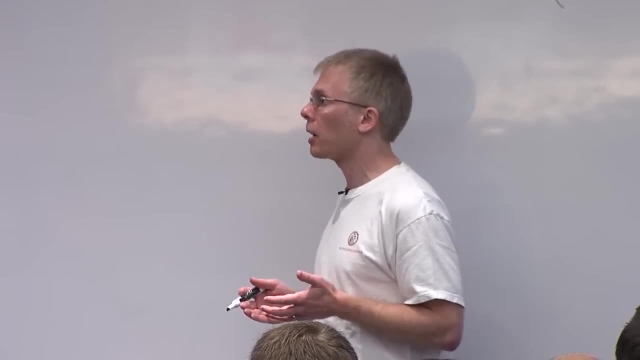 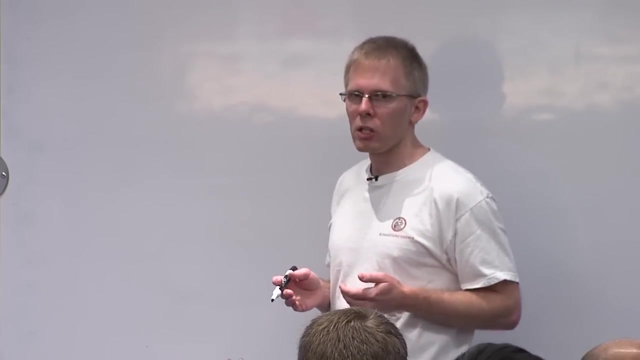 so you can just turn around like that wherever you want, and that's the worst offender kind of solved in a more direct way. But Minecraft is one of these games that is almost the worst possible case for simulator sickness, because not only is it rotating around, as a major part of it, 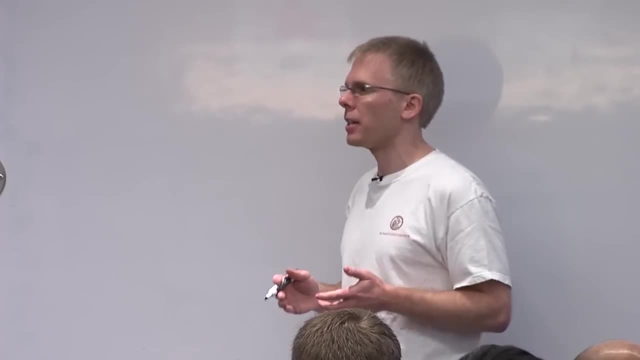 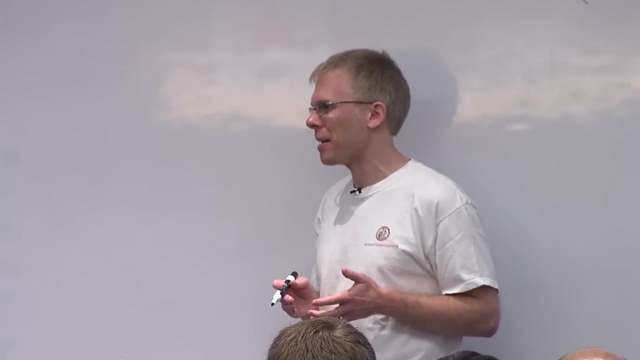 but it's bounding up and down. Parabolic arcs are not your friend in virtual reality, which is a shame. One of our very best games is a jetpack game- Omega Agent- and a lot of people really can't play it because it's lots of arcing around like that. 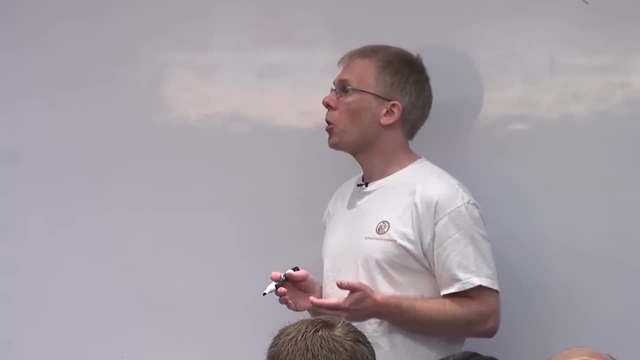 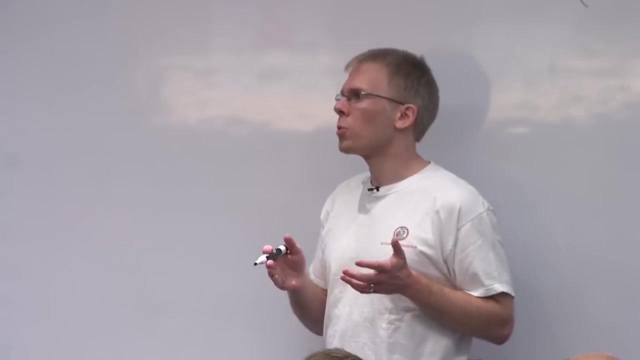 even with some remediating steps that they've taken. But so trying to address the issues in Minecraft has been an interesting challenge. Obviously, I say: well, just don't turn with a stick. Turn in reality whenever you can, And if you need to turn with a stick, well, 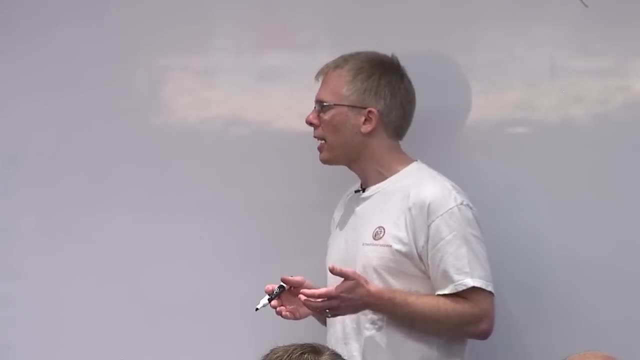 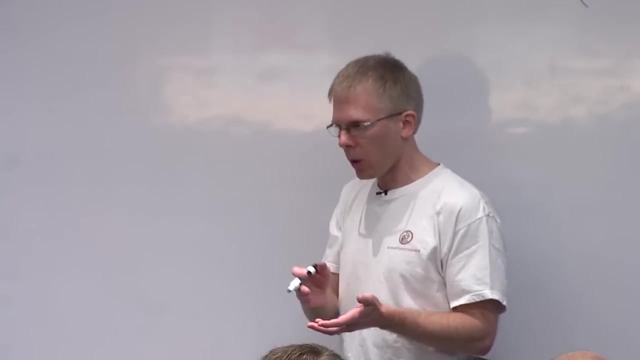 we can do this stutter turning. that's been proven out in a few different places and that largely works. But there's all of these other little things in there, The bounding up. it's so much about hopping up blocks, falling down blocks and that's just bad. 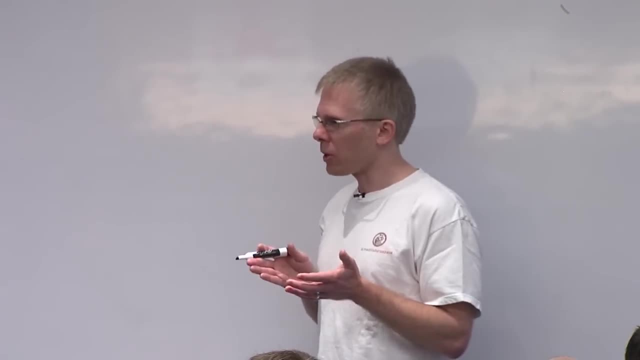 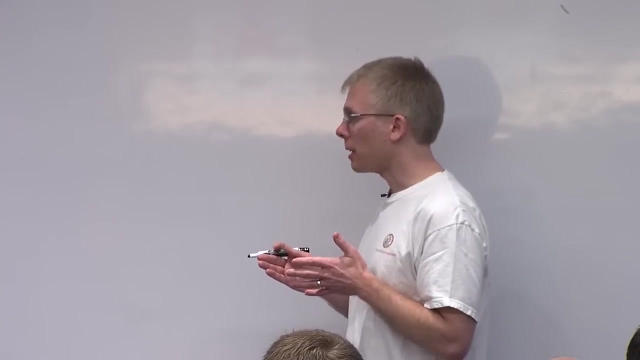 All of these linear, all of these accelerations And there's all these little things with mine, carts and other stuff that do pull you around and even starting and stopping. I've tried to argue that games you should be instantaneous. start None of this, accelerate up and friction ramp down. 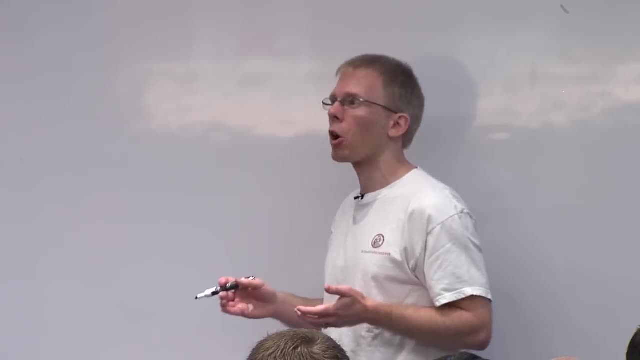 But when it's a game that can be played multiplayer, you don't want the VR people behaving in a different way, and that becomes a sensitive issue from AI, especially when it winds up being competitive. So the idea occurred to me. that's like: 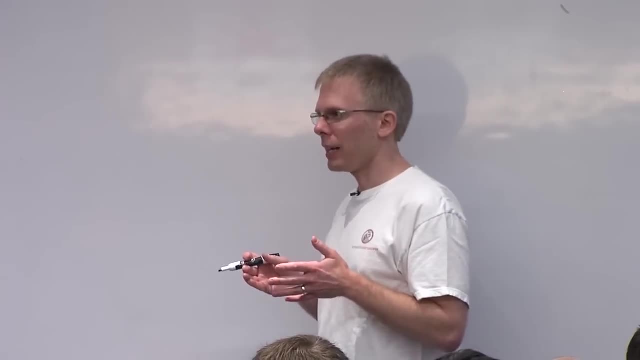 well, what if we know stuttering basically solves the comfort problem? What if I just identified any of the accelerations that are going to cause a problem, whether it's a slow start, a friction stop, a mine cart turn or falling off? 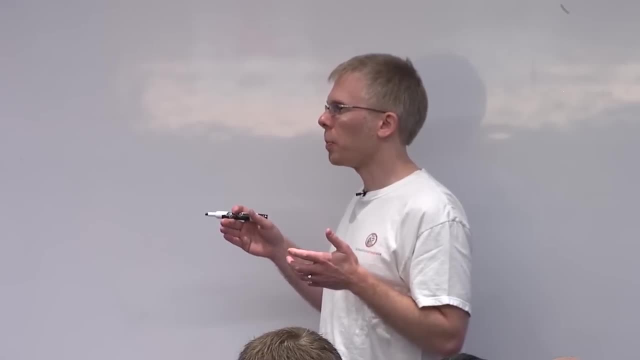 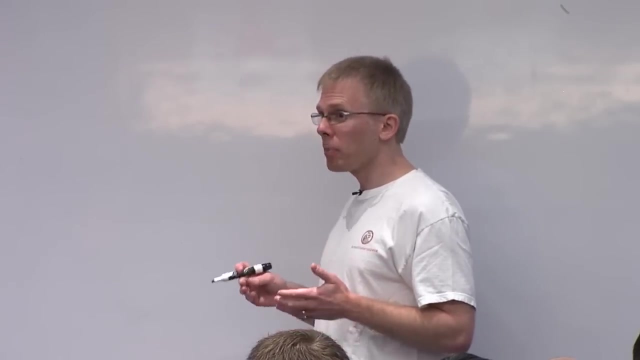 and I just stuttered it to 10 hertz. This would be. it's like: okay, we've identified the root of the problem and here's a solution for it. Maybe this solves everything. Implement it, and it's terrible. 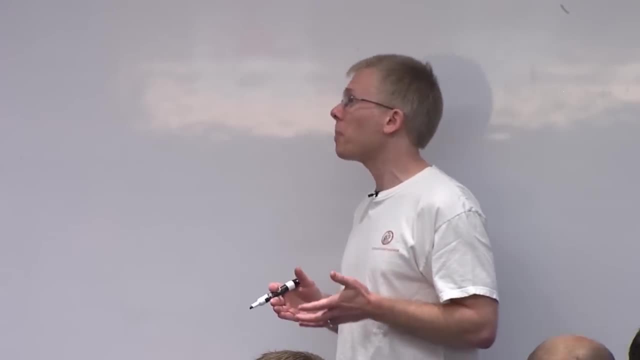 It's jittering, all I mean. it just looks terrible. It doesn't make people sick, but it's not fun to play because it's jerking all the time, It doesn't feel good, It doesn't feel polished, So it's kind of like, well, there's something to that thing. 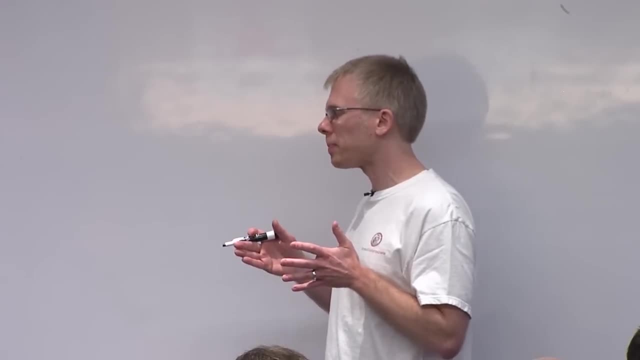 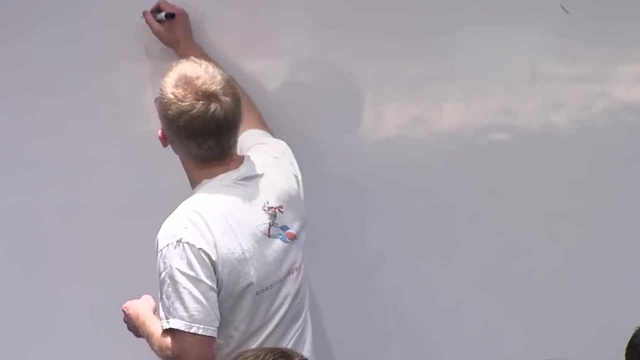 about identifying there's all these things that could cause accelerations and maybe there's a better way to approach it. So what I came to after that is: the idea is like: okay, I'm logging the information. Say you've got a path that goes up like this: 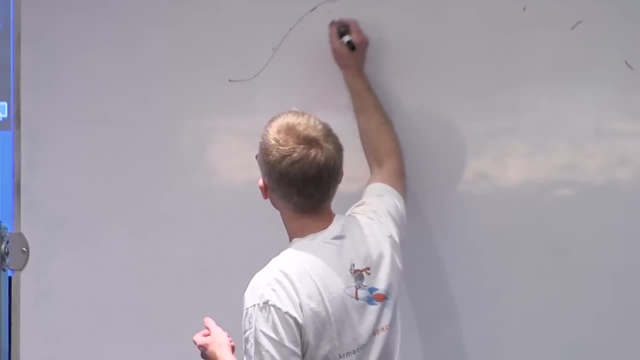 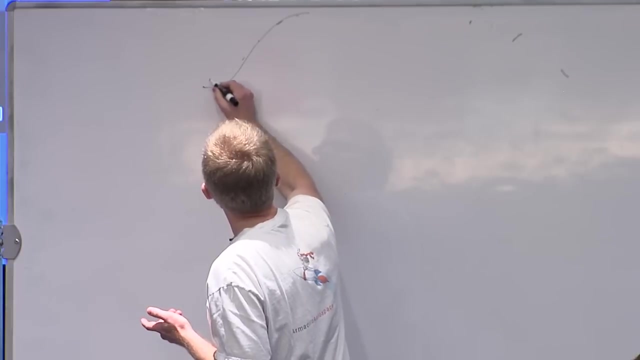 and if you smoothly go through that, that's a set of accelerations. It's going to be uncomfortable, But if you were able to go ahead and linearize that and you just made it a linear ramp from there to there, that's no longer uncomfortable. 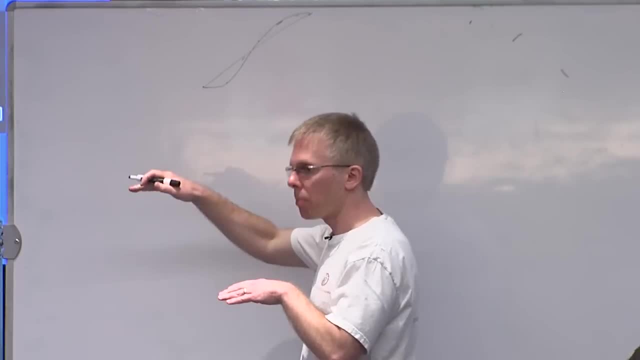 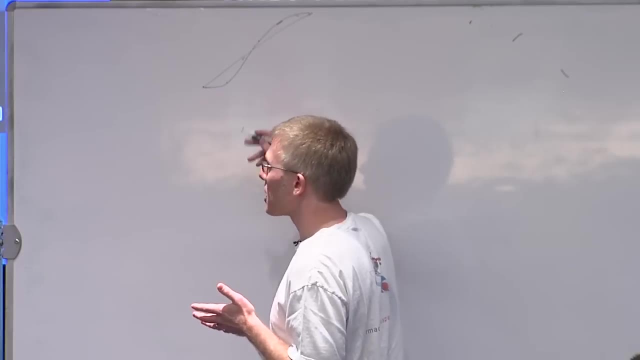 There's one, there's an impulsive change to another slope and another impulsive change when you get off of it. So I logged the positions, positions and velocities. It builds off of the work that I was doing with the kind of stutter elimination. 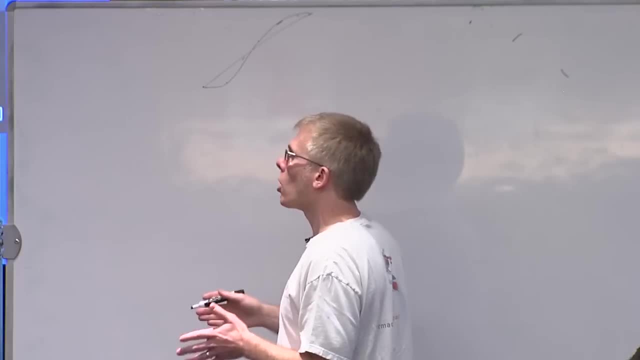 and I kept a little bit of a backlog and I called it lag and linearize. where it lags it a few frames back and then turns it into linear steps And it would do a few kind of smarter things about identifying exactly where 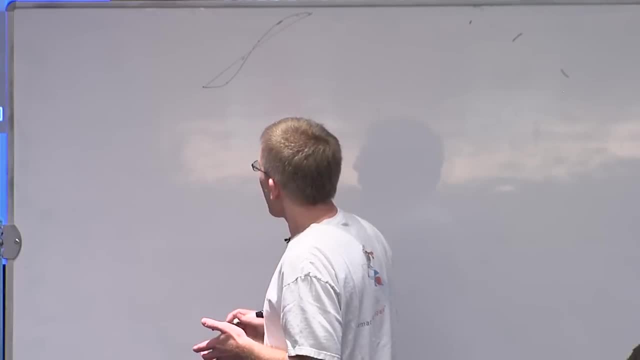 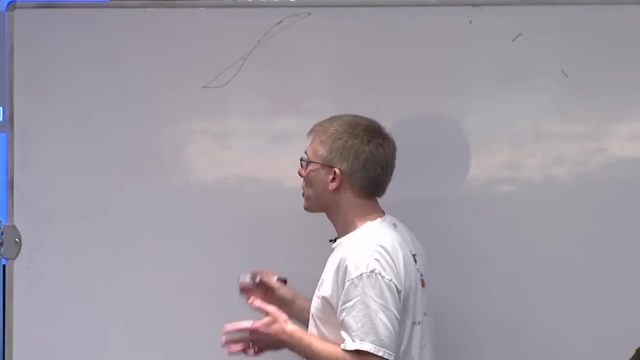 when you made a transition to jumping up or falling off, it could push it there And this worked reasonably well. There was- it was a tunable parameter where you could say at the start: Minecraft works on 20 hertz tick. 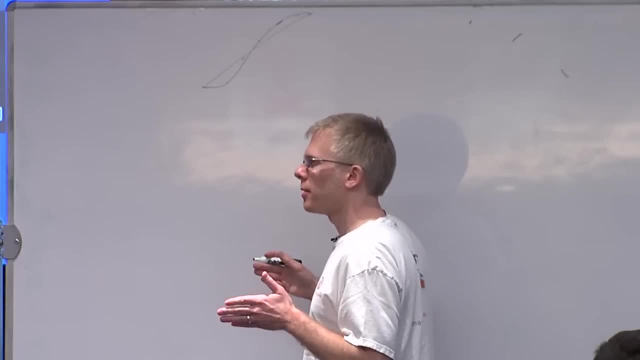 So everything went in multiples of that. So if you doubled that and said: okay, now it's essentially a 10 hertz linear step, that everything gets interpolated between, that helps a little bit. Then you go to three or four steps and then it's clearly doing this linearization thing. 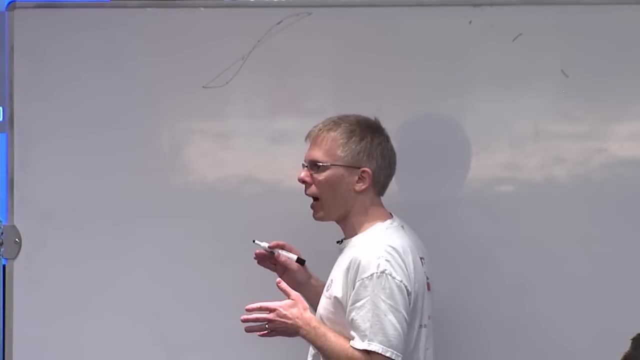 The jumps start looking a little bit more like triangles, you know, not being parabolic, but getting more comfortable, but at the expense of being adding latency to the gameplay, And, of course, latency is something that I crusade against in almost all other cases. 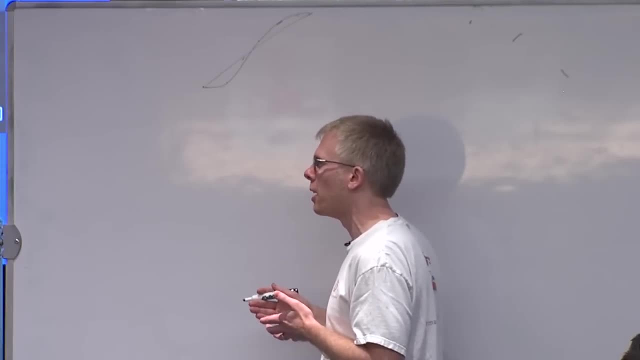 It's strange for me to be saying: well, we're going to add latency here, we're going to spend latency to try to make it more comfortable, And this had, this was having some good benefits. It was something it's hard to estimate. 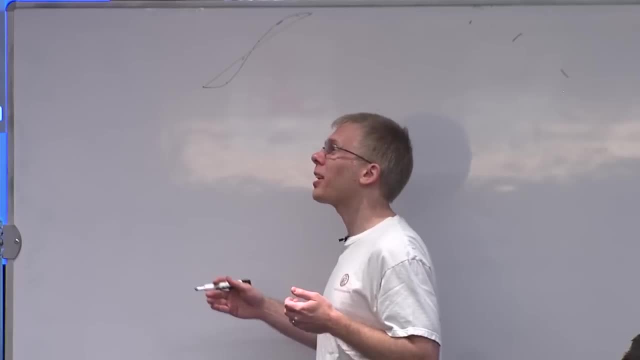 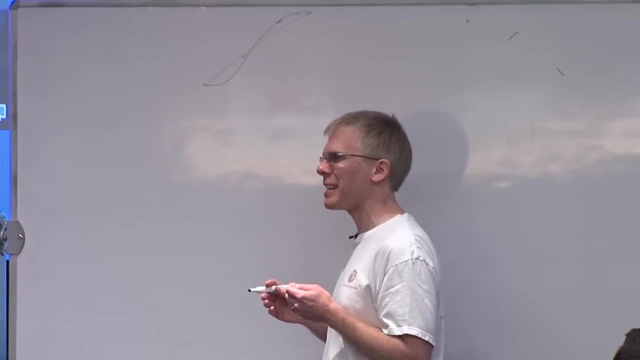 it's hard to evaluate. you know, like, how much less comfortable or uncomfortable are you getting from this? You know you have the test that run up and down the mountains over and over and say it's like: well, do I feel more or less sick? 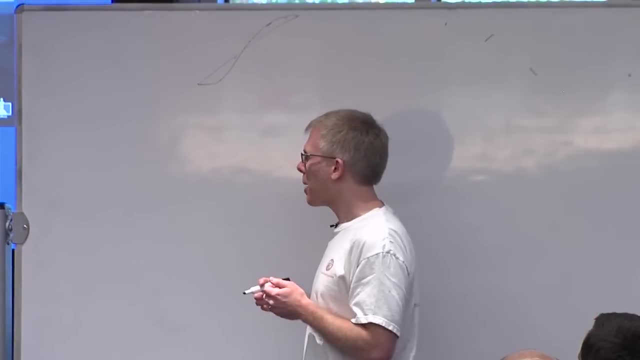 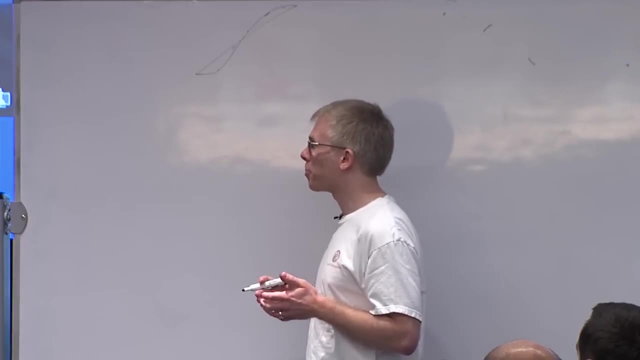 It's hard to get back to a baseline and going through the different cases there, But I would go and play for an hour at a time and say this feels better than what it was before, but I wish there was a more scientific way to make an exact statement about it. 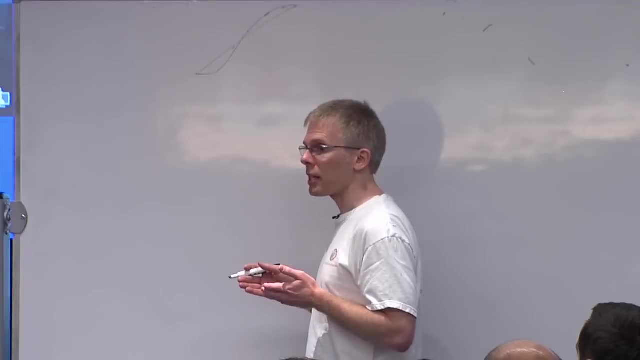 But some other people were complaining about the addition of latency And my thought was that we'd make this a slider where we'd say it's: and you have to be careful how you word things like this, because you don't want it to be something that's like. 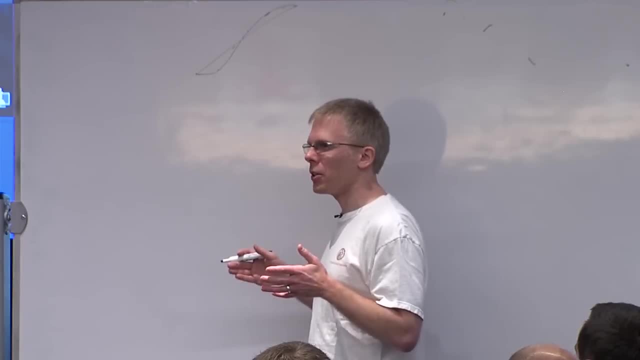 you know, more comfortable, because why would anybody not want to be comfortable? You know you have to. it's the trade off between responsiveness and comfort And I thought we could have a slider that goes from like one to four from there. 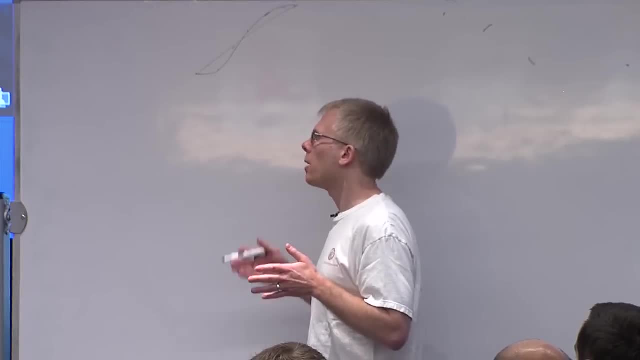 One is just as it is normally, and four would be the more linearized that you could, about the most that you could tolerate before really hating the latency, And we'd leave it up to users. But after beating on the problem a little bit more, 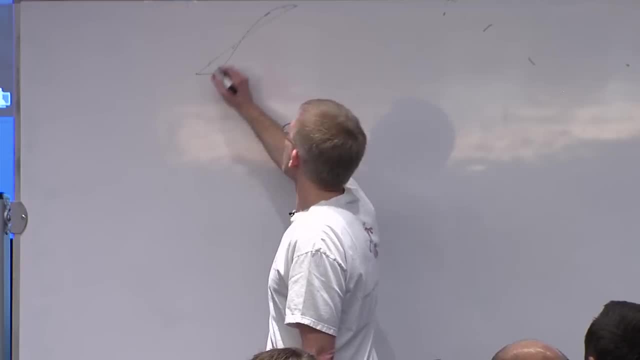 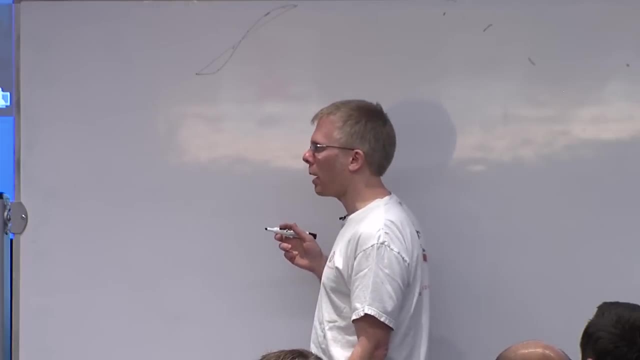 and trying some of these tricks about, like well, identifying exactly when you just start to jump so I could start the linearization there. But I started looking more closely at the actual data of what all these transitions were And it should have been obvious again. 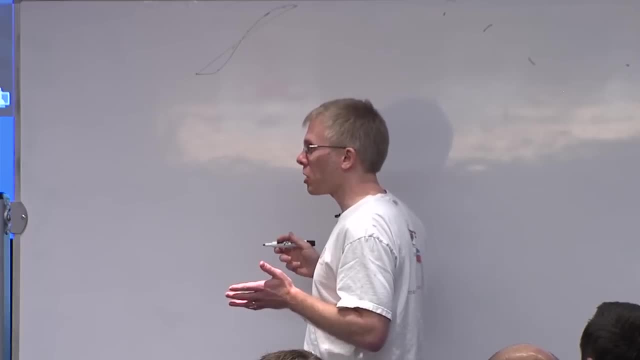 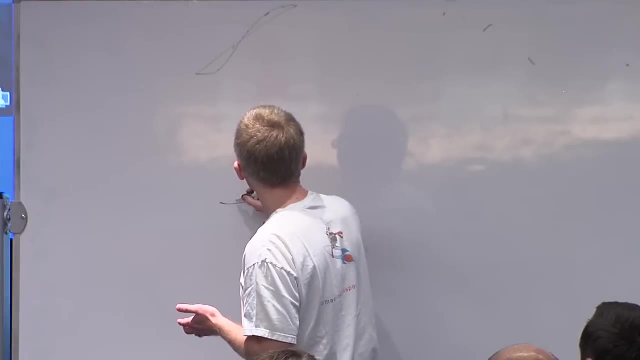 in the beginning, but there's a 20 hertz tick and everything is deterministic. A jump always has the same set of changes where it was, I think nine, something like it, went up to nine frames to go all the way to the top. 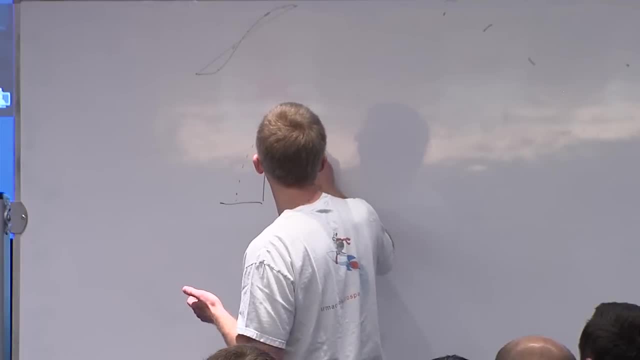 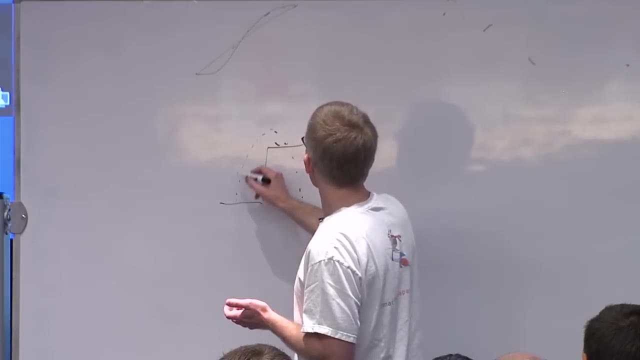 and land on, like the next one, up or 12, if you wind up coming all the way down to the ground. So there were basically three important cases that happened here. There was jumping up, landing on the next block. There was jumping up and landing on the same level. 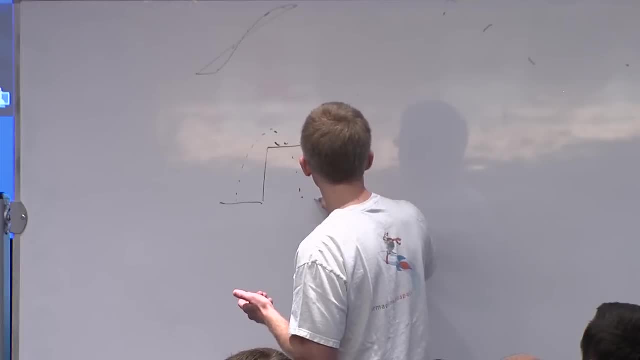 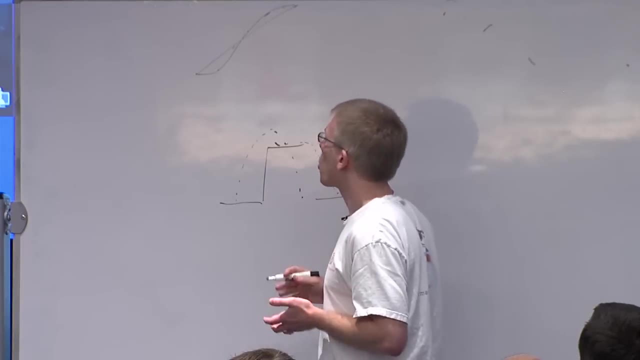 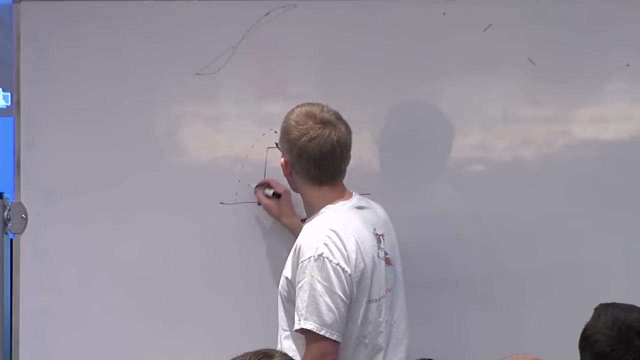 And then there was walking off and falling down to the level below And it turned out that there are a small table of like 20 values that I would take from position and velocity offsets So I could tell what I wanted when you jump from here up to there. 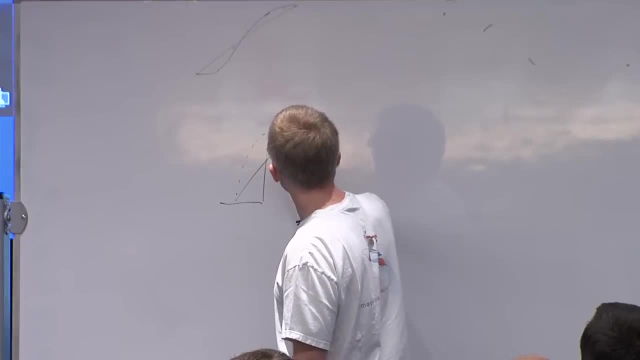 is not this parabolic arc. I wanted this perfect linear arc that just take a linear line that just takes you directly up there, And then from here, one that just takes you straight down. Now, these were 12 ticks. This is far more than I would ever try to put in. 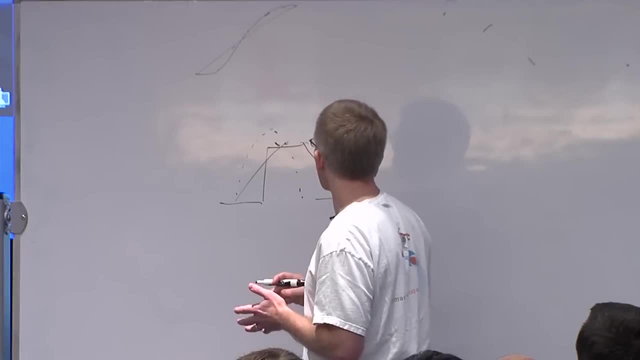 with a lag and linearize approach. That would be just far too much lag to be comfortably playable. But if I could just make this transition from saying: all right, I know that if you are at this offset from a tile then you are at the beginning of a jump. 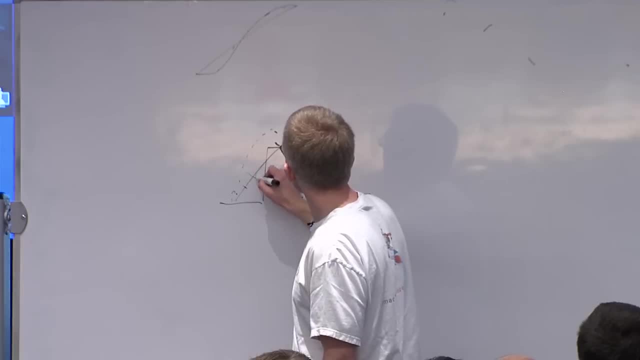 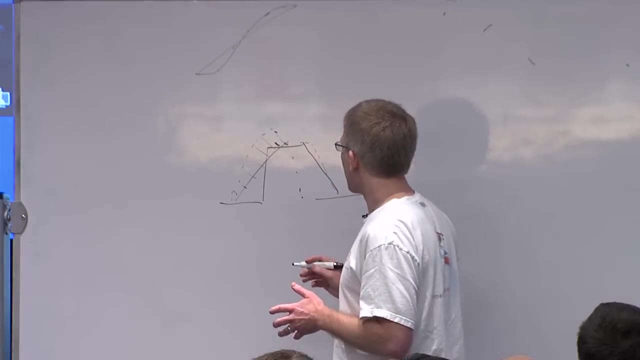 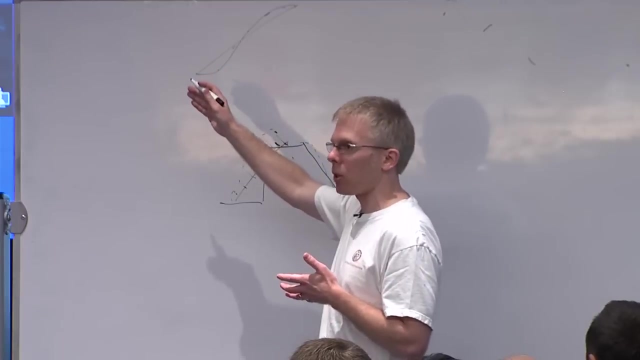 And I could map all of these to points along along the linearized line And this works magically. This is one of these amazing. this is when an idea really turns out right And it's clear that this came from. this was three steps along the way. 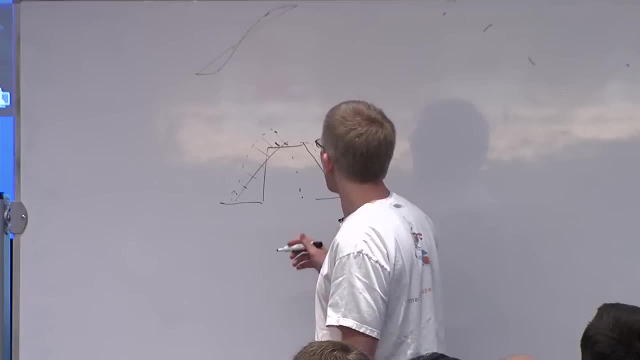 where initial ideas and struggles, working through the different things and then winding up here with something where now you're running around and even if you've got auto jump on, you, bump into the next block and it just slides you straight up like it's on a ramp. 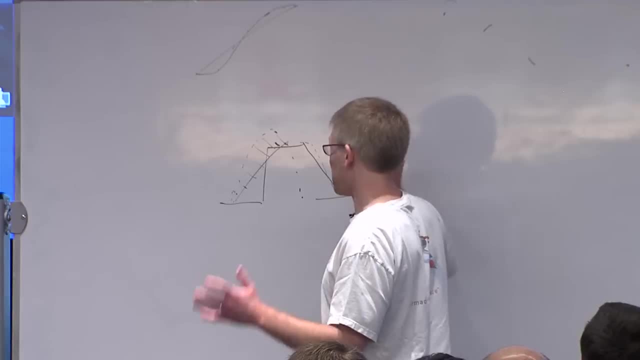 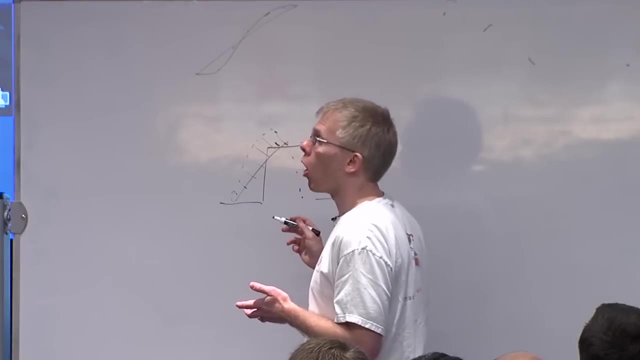 And you slide down And this has been spectacular. So I'm still arguing about whether I need to keep the lag and linearize at all, Because there's still all these other things. There's the slow starts and the friction stops. This kills dead. the problem of 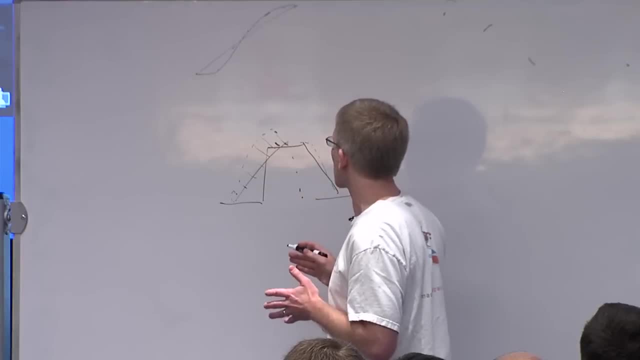 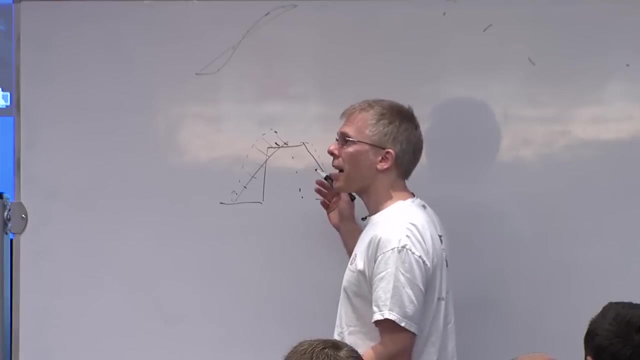 single block step ups and steps down And it works really great. But there are still enough other things where the lag and linearize may still wind up having some utility for that as well, Like there's another, another aspect of comfort with- especially with- Gear VR in navigation games. 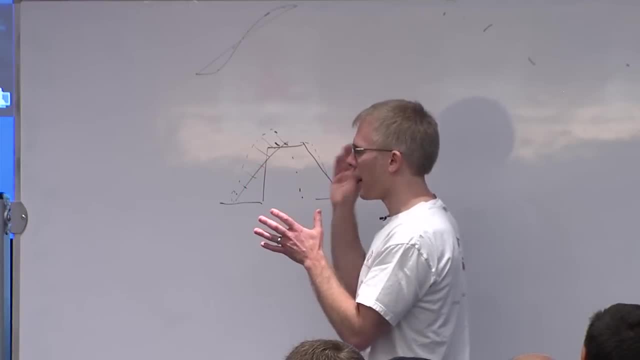 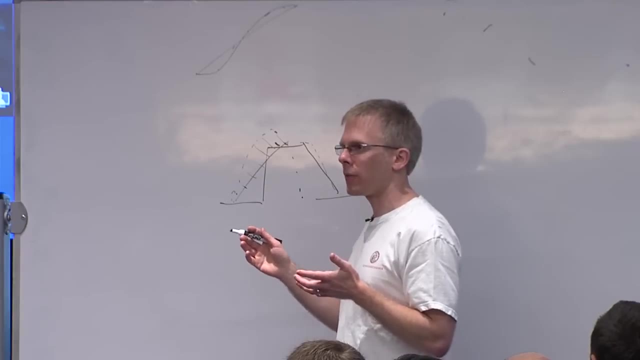 The problem is that we only have a sense that where your head mount is, The tracker that we've got is on the headset, So we know where you're looking. We have to assume that you want to move in the direction that you're looking. 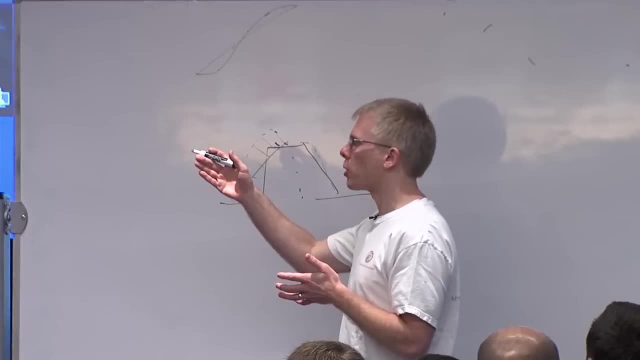 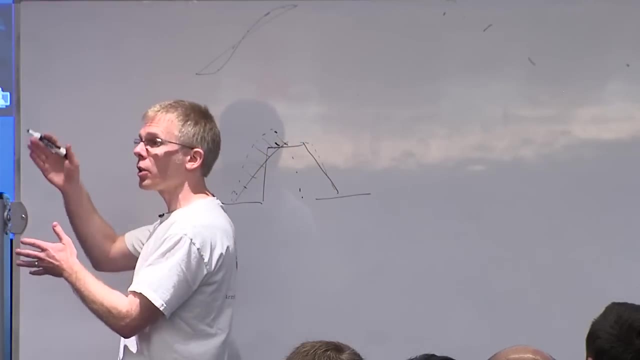 So when you're going forward you're going in the direction of the head mount. Now that causes snake walking where, if you're looking around while you're walking there, instead of walking straight, looking around kind of like you want on a linear path, that would be comfortable. 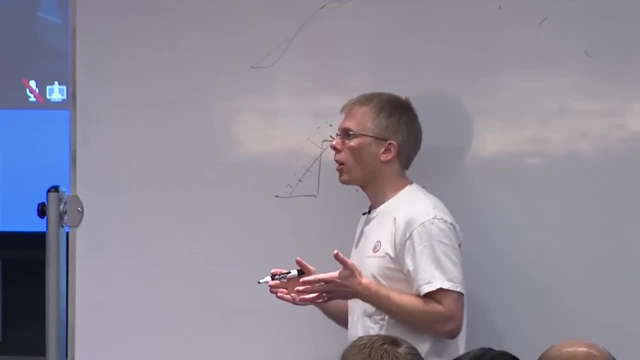 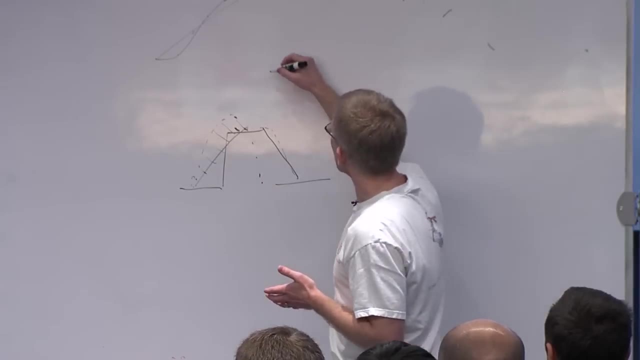 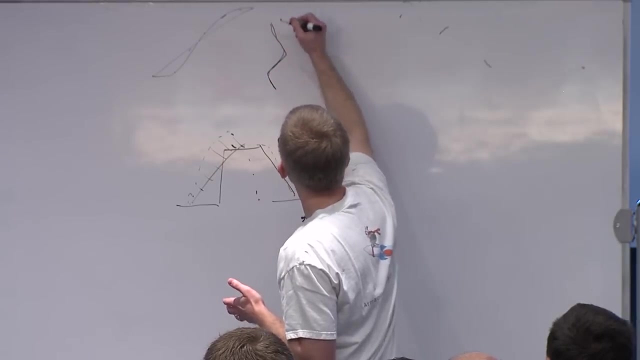 you're weaving as you go through it And that's not comfortable, And the more you look around with your head, the more that happens. So lag and linearize helps that a little bit, where, instead of taking a path like this, you wind up taking more of a linearized path. 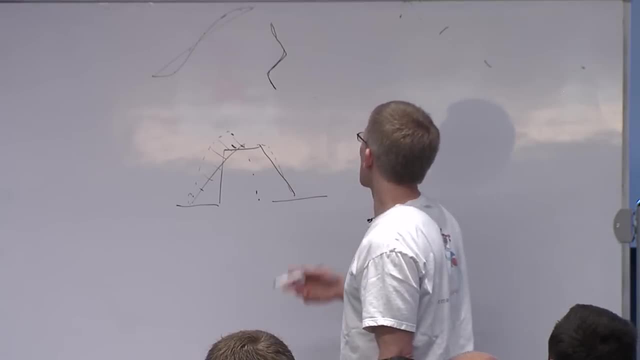 But it's still probably not really what you want. So the other thing that's being at least experimented with as a direction there is that maybe we need to have some offsets between allowing you to look around for some amount of time before changing your actual direction of body movement. 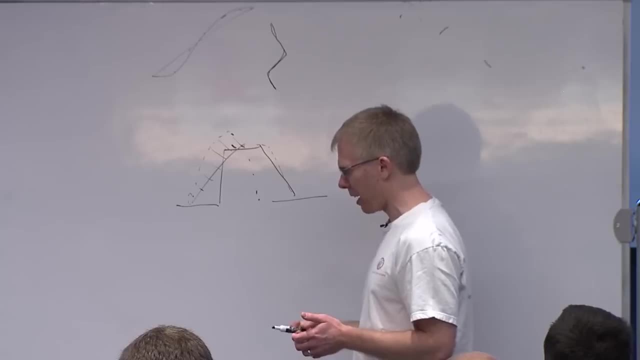 Now what I'd really like to have- and I argue for this on a regular basis- if we had a controller that also had the IMU inside it, so that we could at least track up yaw between it. then you could clearly say: well, the controller determines. 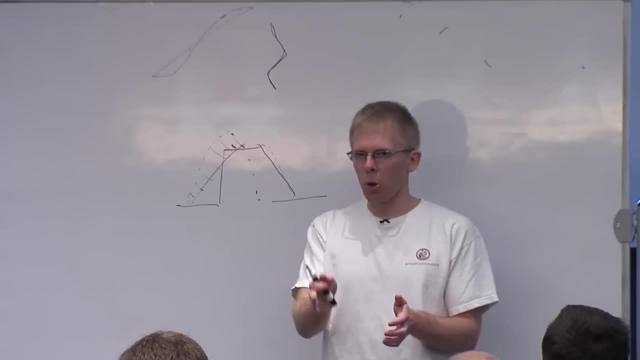 what direction you're going. When you turn in your swivel chair, the controller changes your body direction, your turn direction, and you could turn your head kind of completely independently from that. So maybe we get that at some point. I don't think it's in the cards right now. 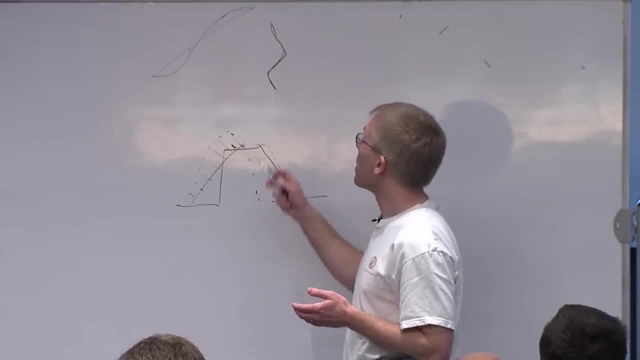 So hacking something around for anti-snake walking, maybe as an aspect of lag and linearize, may be something different, But it was still. this was, and this is all again, mostly stuff that's happened in the last month, or two different ideas that come on. 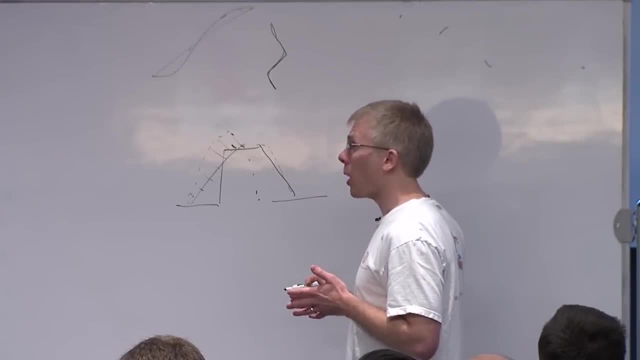 They track kind of continuously about all the different things that are going. There's stuff that I'd love to get back to with some of the vision research work for inside-out tracking where there's that hazard again there, where if I get something that I think is a good idea, 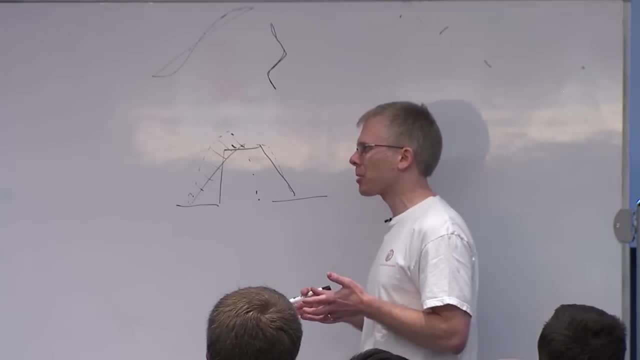 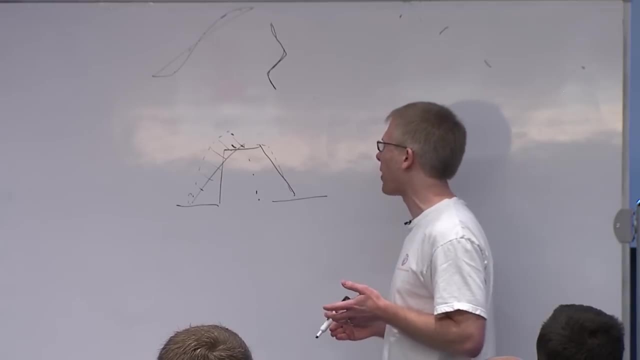 and I don't get to beat on it soon enough. it starts perhaps solidifying into a pet idea in some way, where I maybe won't be as harsh on it when I do finally get around to working on it. So I worry about that.